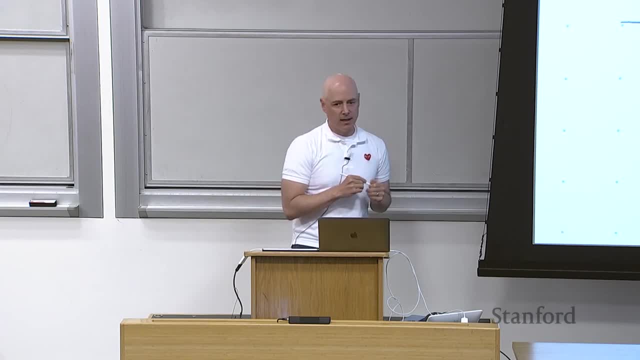 of viewing the world. One of them you're going to use in your homework, called ICA. It's actually the reason I teach it. It's kind of a fun algorithm. It's a weird bit of setup, but it's probably people's favorite homework problems when we look through the kind of feedback. 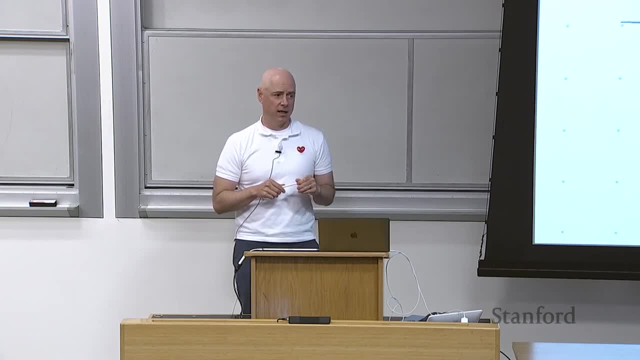 It's a fun problem if you remember the cocktail problem from the first day, where you have people talking in a party and you have microphones scattered around the edge and you want to know who said what. You want to do- what's called sometimes source separation- and understand. 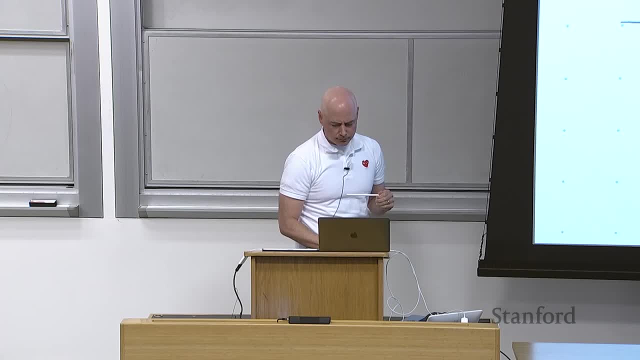 the sources. So we'll do that in the ICA section And then we'll talk about a more advanced topic called weak supervision. Weak supervision is industrially used to create large training sets for big deep learning models, which you've just come out of that. But these are: 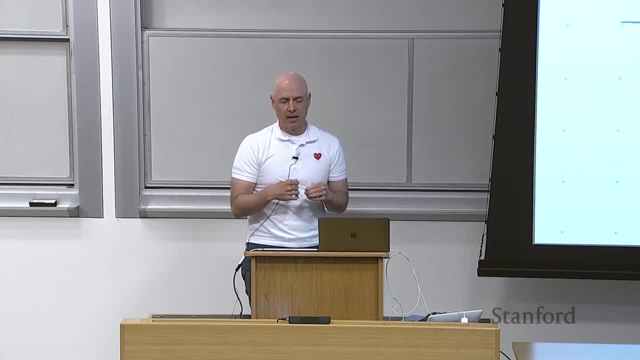 labels that are lower quality than the traditional supervised labels. And then, finally, we'll talk about self-supervised learning, which is really exciting and is one of the big revolutions in machine learning, where we train on something simple like predicting the next word, And 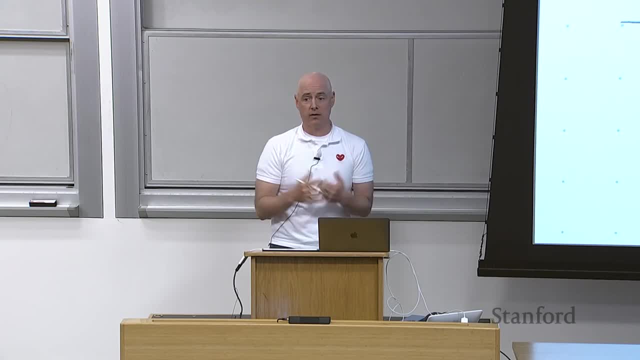 if we train on enough data, we can use it for all these other sometimes called downstream tasks, okay. So that's kind of the program for the next four or five lectures, And today we're going to start with those basics, okay, So we're going to start with the basics as 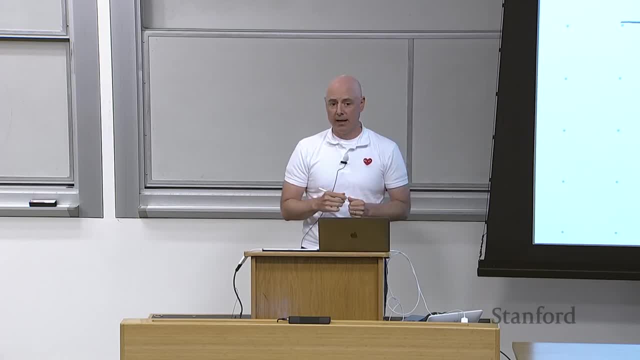 unsupervised and work our way up to pretty modern stuff. And I will say, historically, I would say five years ago, I kind of didn't like teaching unsupervised because it felt kind of squishy and weird. to be honest with you, It didn't. 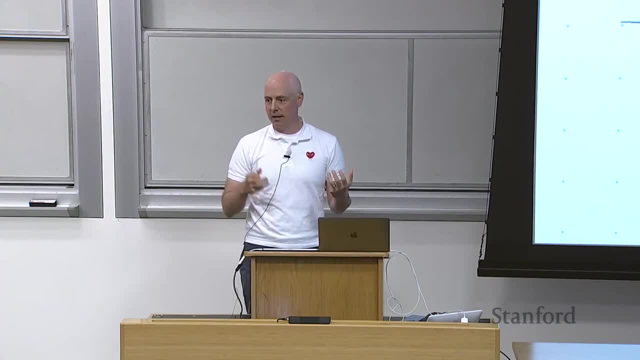 have the beautiful theory or maybe even 10 years ago didn't have the beautiful theory of supervised learning, where you could say like this is the right model and we go find it in a lot of cases. But that's been where almost all of the research activity not only 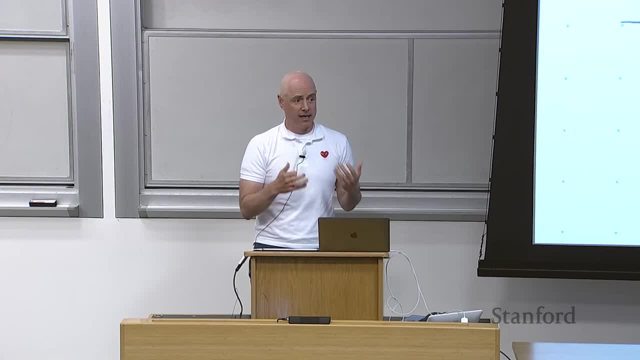 in my group, but kind of from AI over the last three or four years has been in this unsupervised realm. So we'll start with some of the classics and get our way to something really, really exciting. okay, And probably an algorithm you already know or probably you can guess kind of how it works. 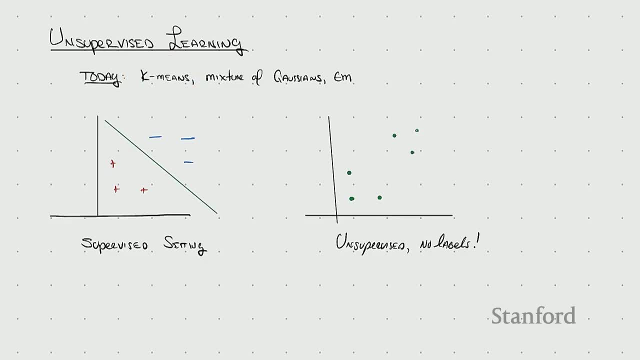 is this algorithm called k-means. all right, And then we'll get to these other ones, But this is the one we're going to start with first. So what's the difference? So, in the supervised setting right, we get points, And the key issue is that the points come. 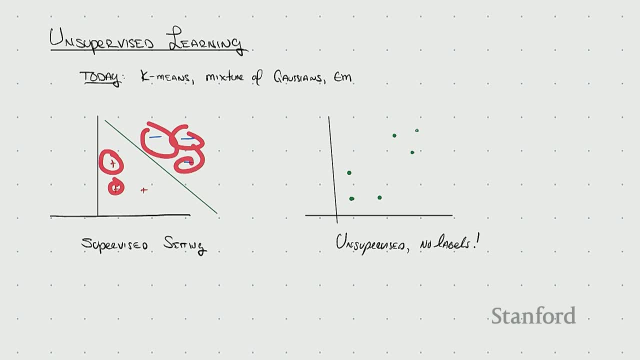 with labels. So you have labeled these plus and these minus, as we were doing, and we would draw a line or a boundary in between them. That was the way we formalized a wide variety of learning tasks. okay, Right, And the point is, is those pluses and minuses? 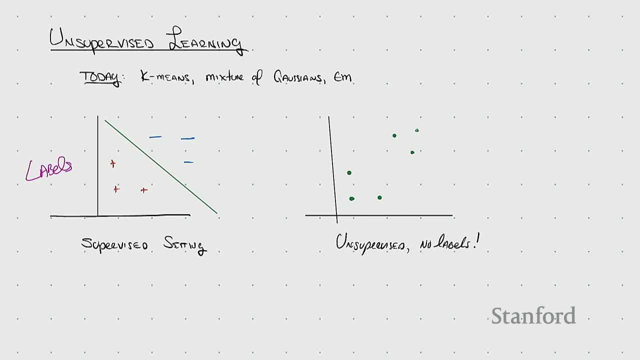 those are labels. right And unsupervised started in this setting. I give you the points, but I don't tell you any labels underneath the covers. okay, Now there are many things on the spectrum between. I give you the labels perfectly to. I don't show you any information about the labels. 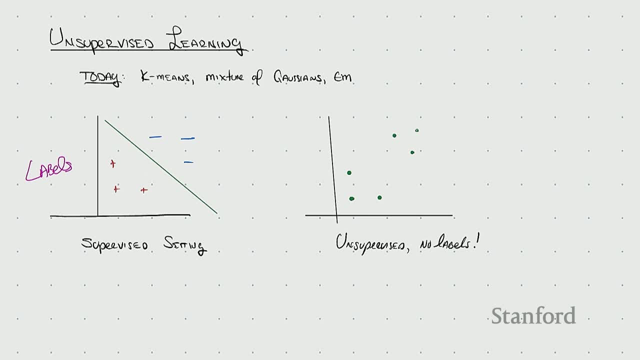 and I just show you the data points And we're going to talk about that spectrum. but now we're going to start in the cleanest setting, in unsupervised, where we just see those points. okay, Right Now. So what we're going to do here is what you should calibrate. here is like: what can we? 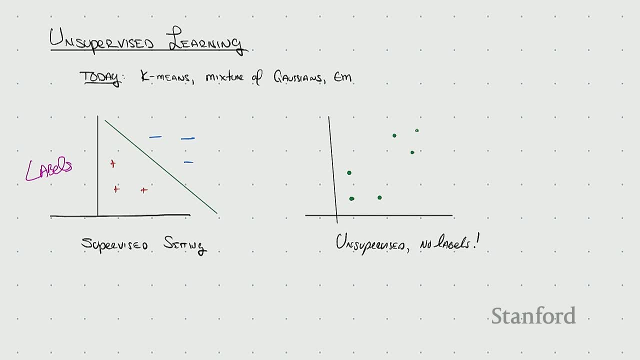 expect as an answer. So in the supervised setting, as I said, it was super clear what we wanted, Like we could talk about what this line is and we can go deeper and deeper into like why that's the right line, why that's the right separating hyperplane. In the unsupervised 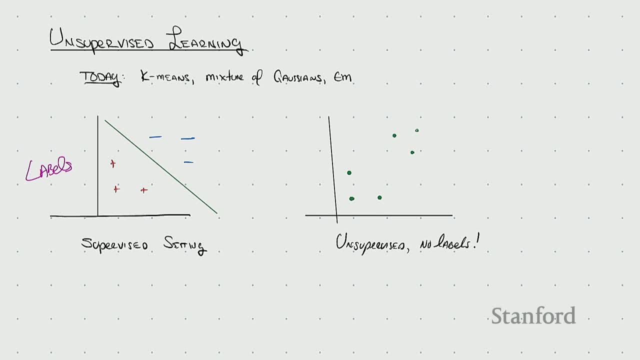 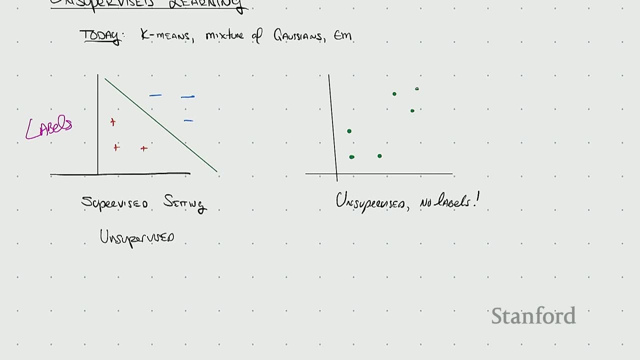 case it's necessarily squishy, and we'll talk about the ways in which it's squishy And what I mean by that is it's harder in some sense. So unsupervised learning is harder, And what I really mean by that than supervised. What I really mean by that is we have to. 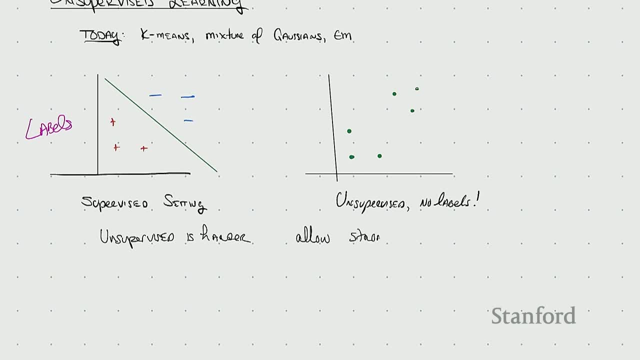 to allow stronger assumptions. okay, Stronger assumptions, Right. so one of the things that kind of pass by you without thinking about it too much in the supervised setting is you're like there's just some data and there exists a separator, there exists some class. 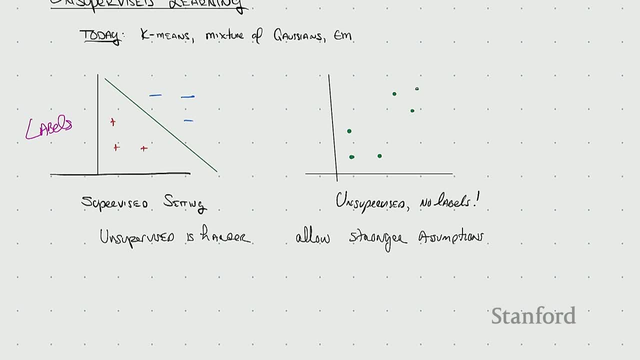 That's pretty weak for what we had to assume about the data For unsupervised. we're gonna have to assume there's some kind of latent or hidden structure And a lot of the conversation is: hey, if that structure is there, can I provably recover it? 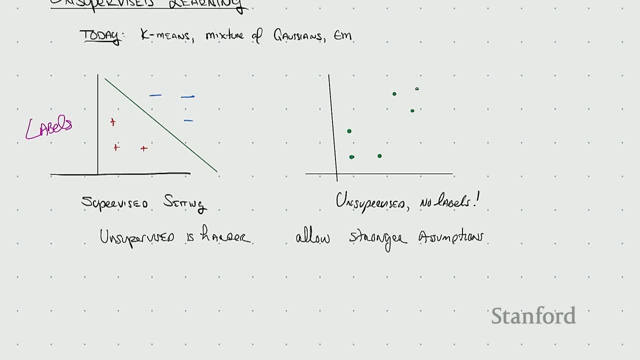 That's the kind of thing that we're going to do, And we're gonna trade off kind of assuming more about our data and trying to find it robustly okay. And now, compared to supervised, we're also gonna accept weaker guarantees okay. 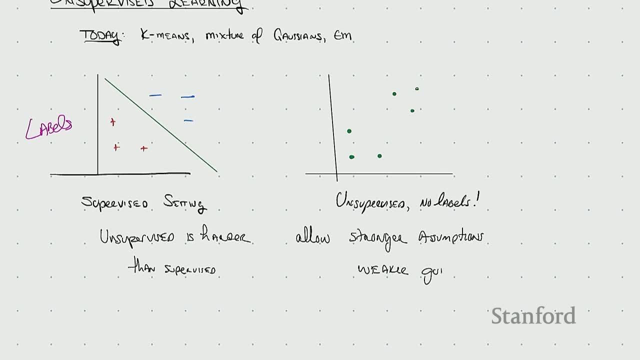 So weaker guarantees. So in supervised learning, in many cases that we cared about weaker guarantees, we would say like we got exactly the right answer. right, This was the right model. We could say: you know, there was some theta star out there. 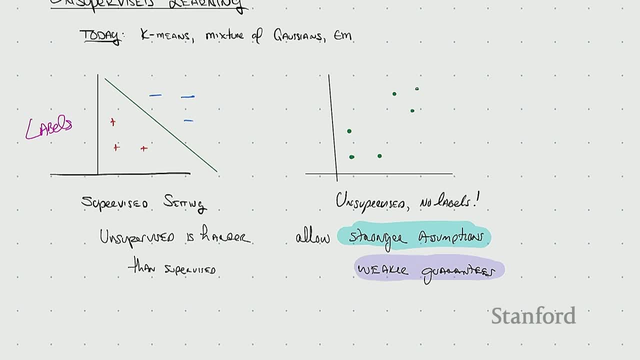 that was just the right thing we were looking at. As we'll see, and I'll come- I'll show some examples in a second. in this unsupervised world, it's not super clear. you know what the right answer should be all the time. 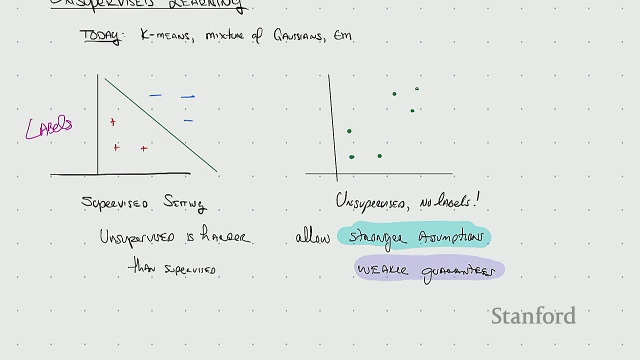 If I just show you this picture and say how many clusters are there, some of you say, well, there's two clusters. Some of you say, well, why aren't there six? There's six points. Why isn't each one in its own cluster? 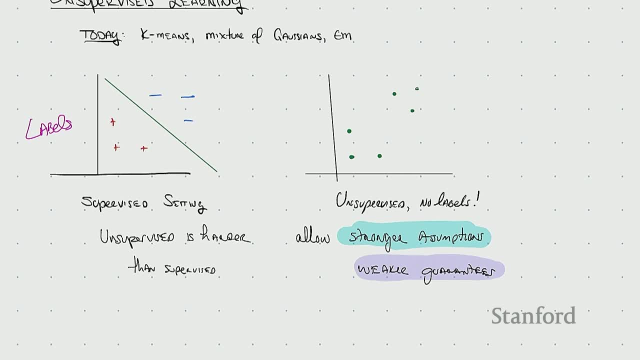 And, if we'll see, in some examples it's not really clear what there is. We have to make some assumption or do some modeling to understand and kind of get to the bottom of our data. okay, And so that's what I mean by weaker guarantees. 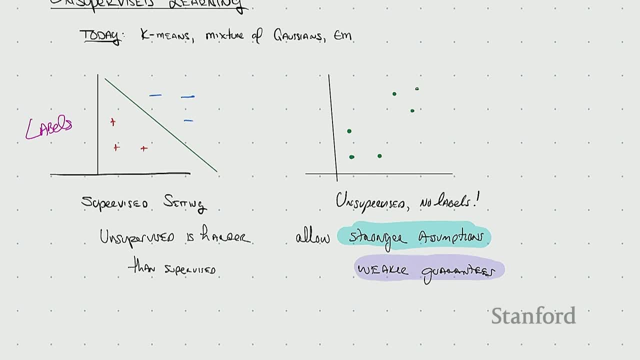 and stronger assumptions And we'll see those mathematically, but just keep them in the back of your head. We're gonna be more comfortable saying, like, what, if our data are generated this way, That's gonna be a stronger assumption. And then we're gonna say: you know? 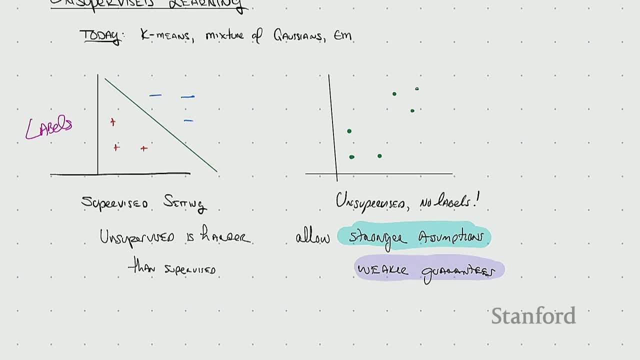 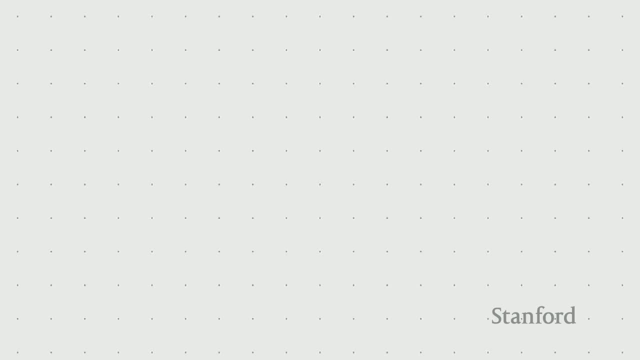 we can recover something that's pretty good some of the time. all right, All right. This is less jarring to you than it was like historically, honestly, because historically we would teach the first part of supervised learning without things like neural nets and all the rest. 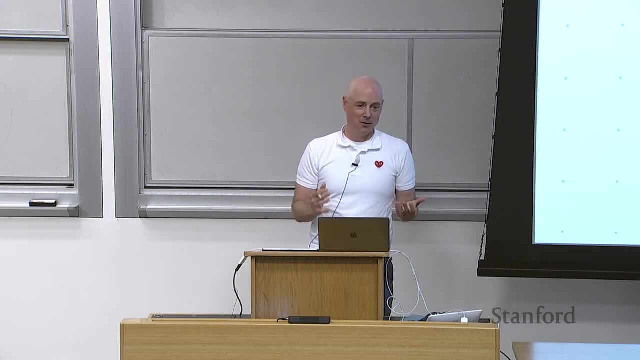 And neural nets. you kind of got comfortable with the fact that, like, hey, maybe it's computing something useful, maybe it's not, We don't know. we just run it for long enough. okay, This used to be a little bit more disturbing, okay. 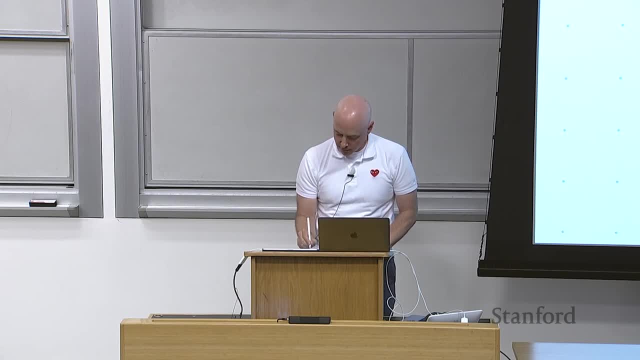 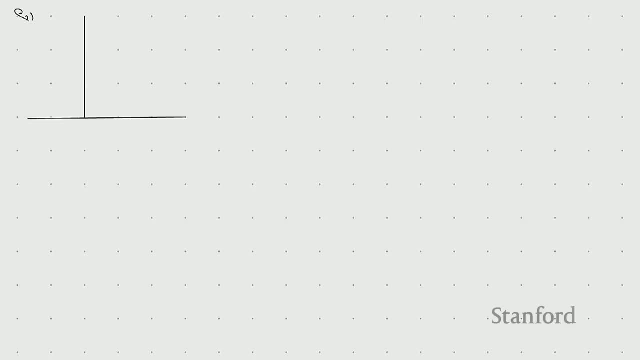 So if you look at the literature, you'll see that in it. So let's start with our first version of this, All right? So what we're gonna be doing? we're gonna be given some data. Oops, it's not very, doesn't look very nice. 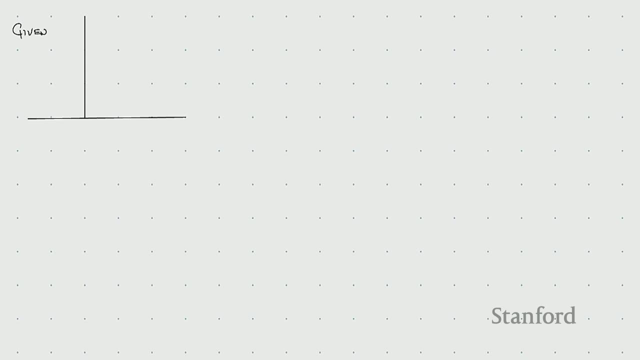 This is our given data, okay, Given, And we have some points, And this is basically me just introducing notation and copying what we had before. all right, We're also here, as I mentioned, that stronger structure. we're gonna also be given a parameter. 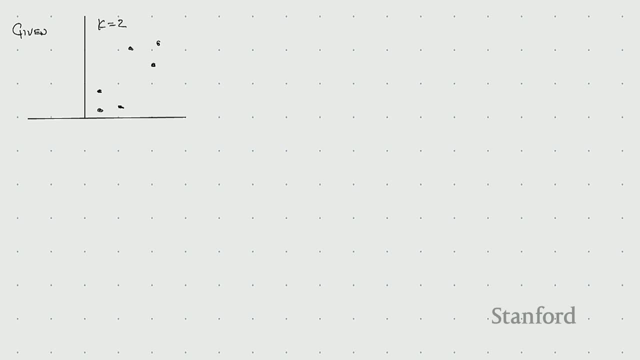 which says how many clusters we think there are. So the game is gonna be here. I'm gonna write down: you know, k is equal to two And our goal is that what we wanna do here is find a good clustering right. 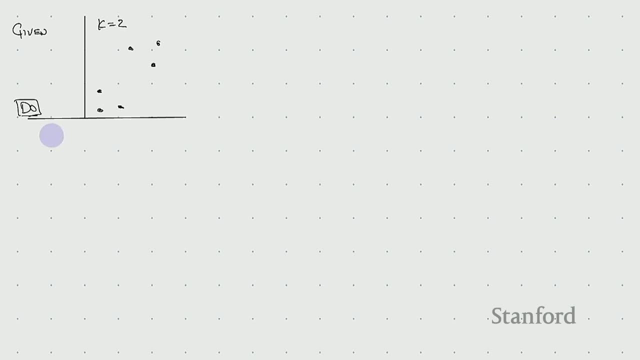 And so our do is: we wanna use two. I'll use colors here, apologies. hopefully it'll be obvious. You don't need to know what the colors are, But you know, we'll kind of find two colors like this: 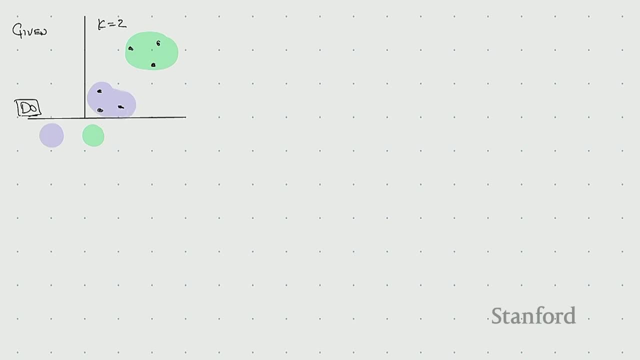 Say like: in what sense is this kind of intuitively good? Okay, This is the same thing we were doing in supervised learning, right? We're like this is an intuitively good thing. We talked about different loss functions. You're kind of an old hat at that. 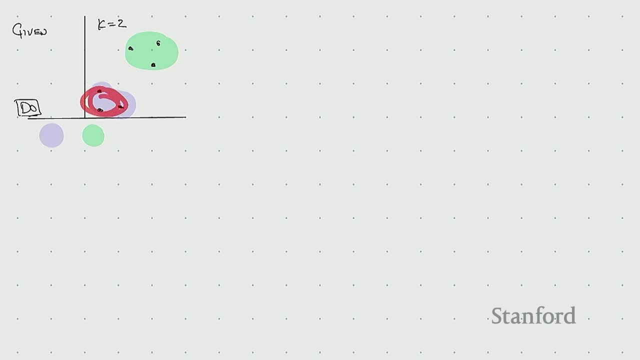 So you can kind of imagine what we're gonna do, Like: oh, the loss in some way from some object shouldn't be too far away. okay, Now the k means is hinting at that object is gonna be the mean or the center of that cluster. 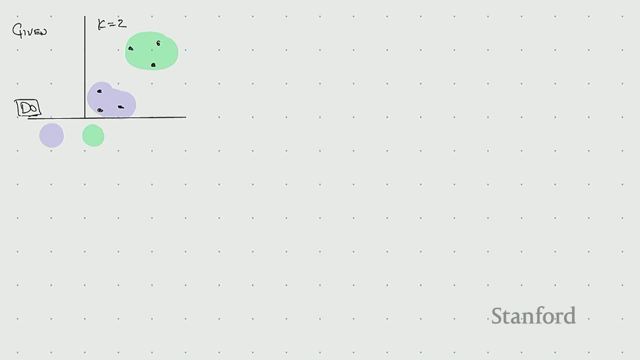 You kind of wanna minimize that center cluster. That's not obvious. We'll come back to it. Okay, so this is what we're given: Given data, we're given this k parameter and our goal is to create some clustering that we're gonna talk about. 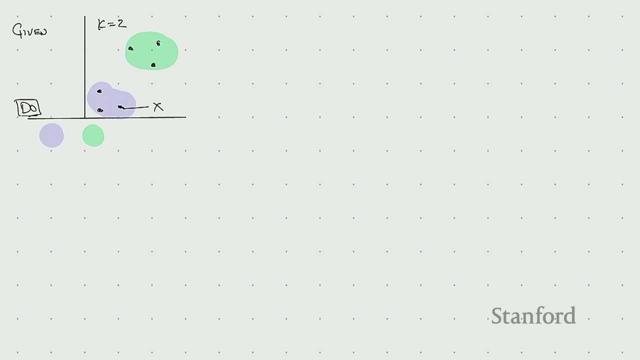 So we need a little bit more notation. okay, Now this guy, we'll call some point x one, we'll call this point, say x three, And that's just the notation. I'm gonna write the notation formally in a second, okay. 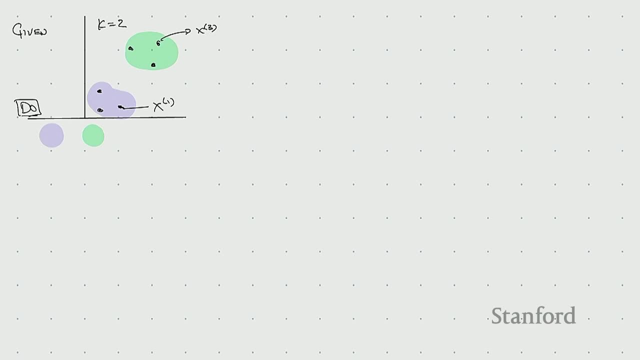 But before I do that, is it clear, kind of, what the setup is? You give me some points, you don't tell me any labels. You'll also tell me how many clusters you're looking for and then it's my job to find them, find those clusters. 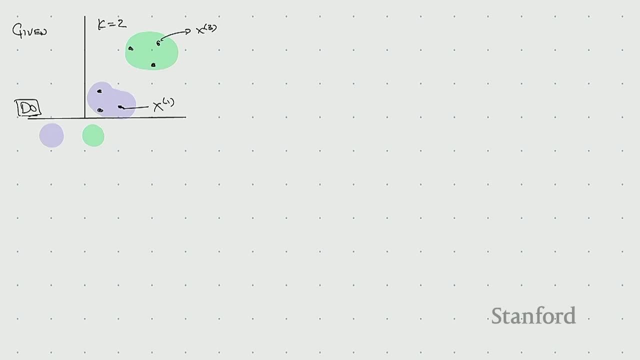 and we'll talk about how to make that precise and formal in a second Awesome. So I'll just write down some notation and if there are any questions, please pop in. There's one question: Sure, Why are you going with x? 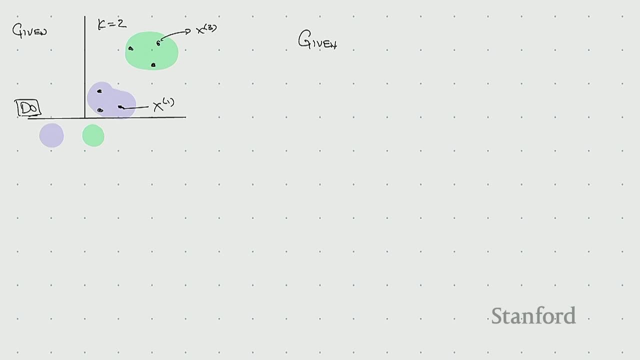 Why x three? I'll show you that notation in just one second. So yeah, let me write the notation down and then I'll come back to what I'm calling there. Great question, Also on the end thread. sorry that I forgot to do it earlier. 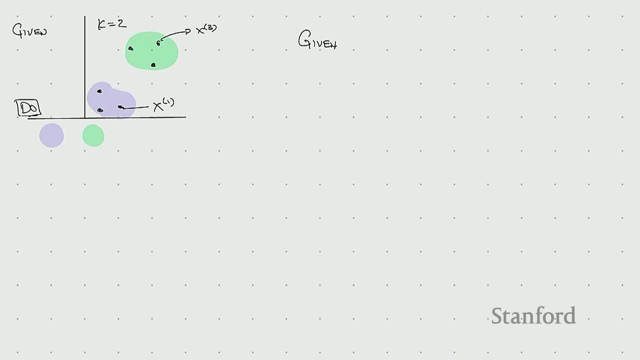 someone's asking: what about the unknown k case? We'll come back to how to select k later. Some of our algorithms, as we'll see, just to go ahead, some of our algorithms will actually have a natural test for k. We'll be able to basically try all the different k's. 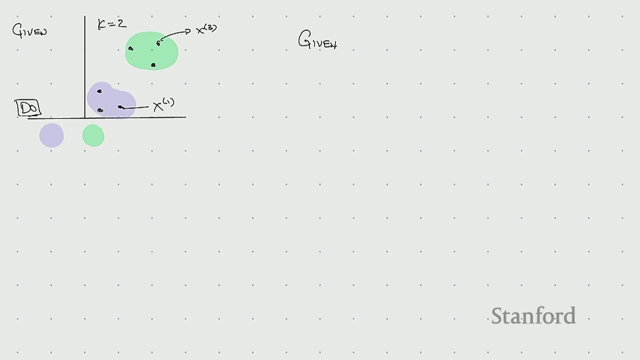 and pick one. Some of them will not and it will be a modeling decision. And let's come back to that question, for how k is unknown. By the way, it's not super unrealistic that k isn't known. You may know. 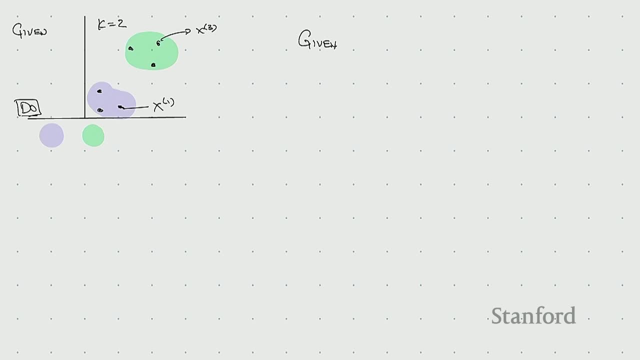 by looking at your data that roughly you think there are about three or four products or something that people are talking about or various different topics, And those are the kinds of situations you will need kind of k means in. But let's come back to it. 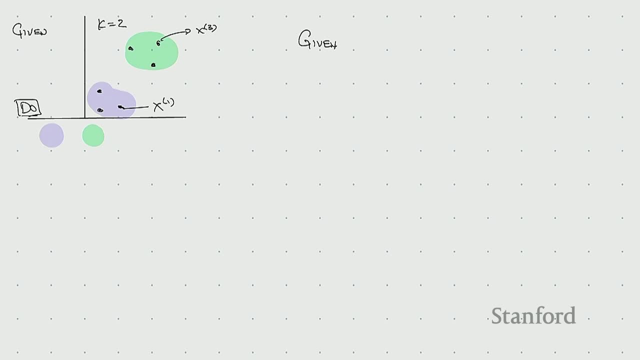 Great question on the end thread. All right, so let me give you some proper notation so we can actually talk about this, maybe a little bit more mathematically. We won't be super heavy on that today, So what we're given in general is some x one to x n. 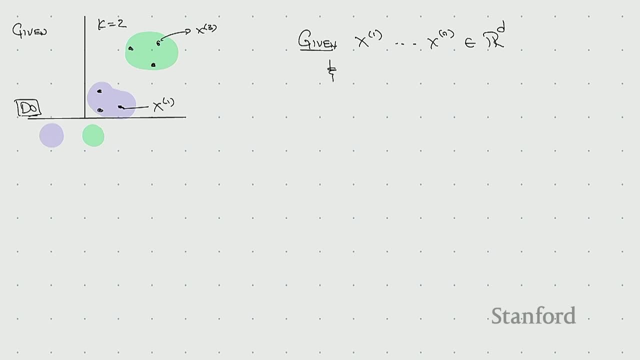 that live in some vector space. And here we're given some k, which is the number of clusters. number of clusters. We need one bit of notation to do this. So how am I gonna make these colors into notation? Well, I'm gonna introduce this thing. 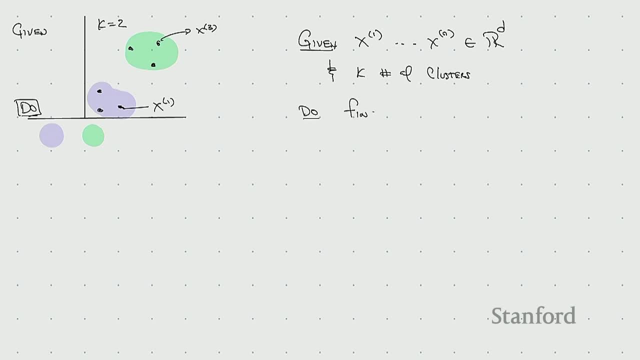 We're gonna find an assignment- oops, find an assignment- of points to clusters, Of points to clusters. Okay, so how do we do that to the k clusters? So what we're gonna have is we're gonna have a map that's called ci equals j means point i to cluster j. 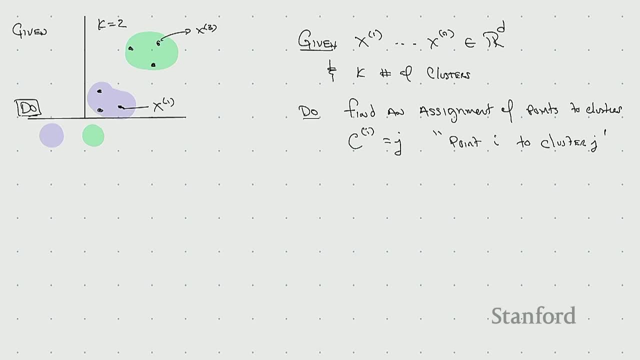 Okay, so here i is gonna run from one to n and j is gonna be from one to k. right, These are the same. this k and this k are the same. okay, So back to this. So when I was drawing, I got a little ahead of myself. 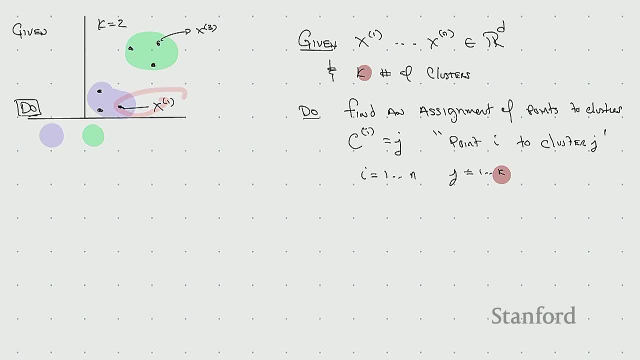 I started to draw the notation before giving it. This is just saying we can call this point x one, this point x three. I'm just noting down what the points themselves are And then what our goal is to find this map that I drew by kind of this highlighted color. 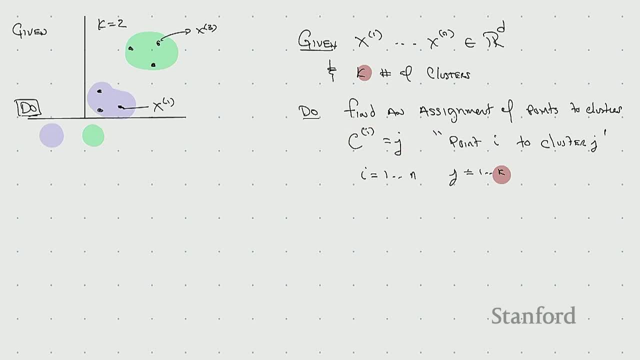 and that's gonna be this ci j character here. So this is highlighted in yellow. for reasons not really sure why I picked yellow. okay, So, for example, c three equals two encodes this fact that c three is in cluster two and I made the green cluster two. 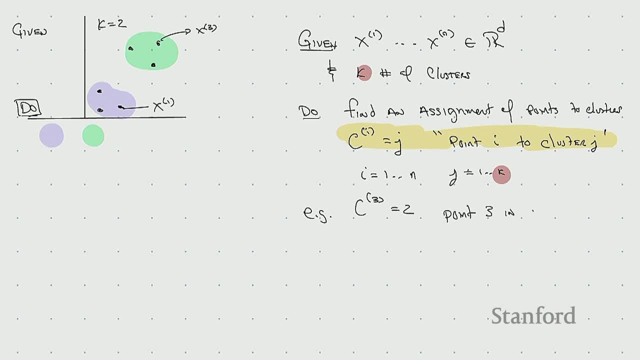 So point three in cluster two, okay. Okay, this will sound kind of opaque at the moment, but this is a hard assignment. We're saying every point belongs to exactly one cluster. The reason I'm signaling that is in the end of the lecture. 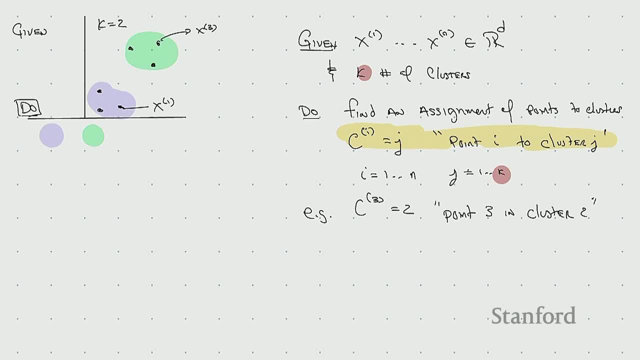 we'll talk about a soft assignment where we have a different version of this. okay, But that's what this is. Anything that's obtuse about this: okay, That's what this is. Anything that's obtuse about this- okay. 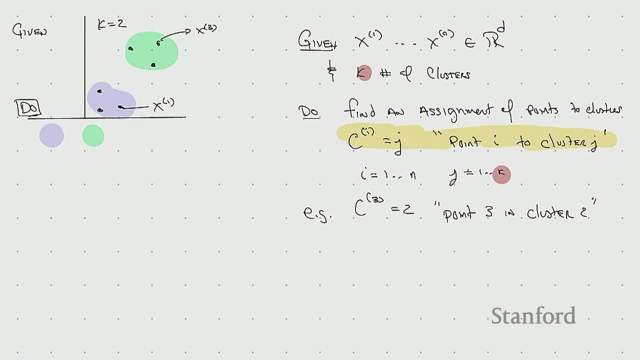 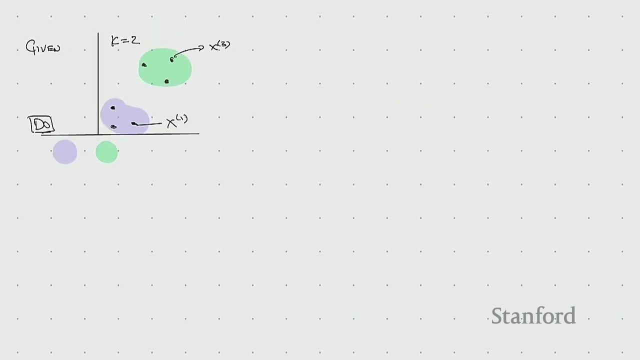 That's what this is. What about the setup? All right, let's see an algorithm. All right, so let me copy this piece. All right, drag it over there. All right, get rid of these characters, because we don't see them. 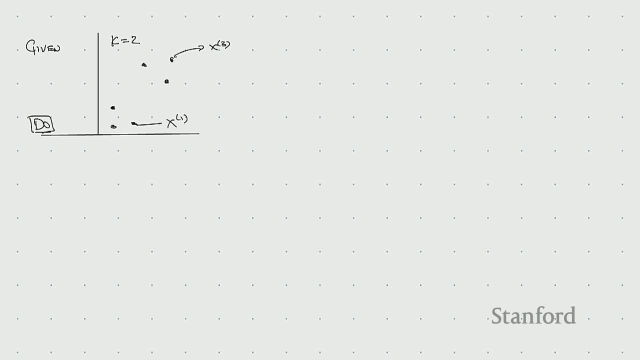 And this is our input, okay, So the question we want to ask is: how do we find the clusters? How do we find the clusters? How do we find the clusters? Now, there are many ways to do this And if you're a complexity kind of nerd, 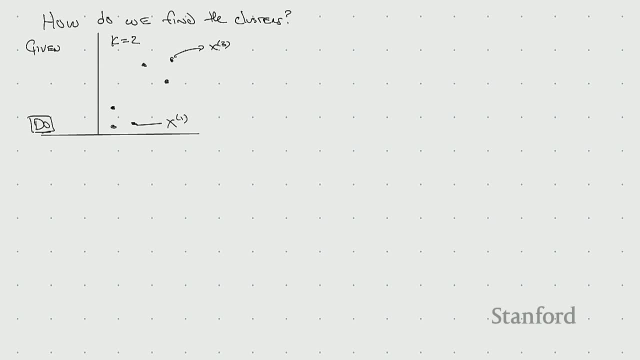 then you would say like: is there a polynomial time algorithm for this and all the rest? The answer's no. Actually, it turns out there's an NP-hard problem, So we're gonna have to use a heuristic-based algorithm to do this. 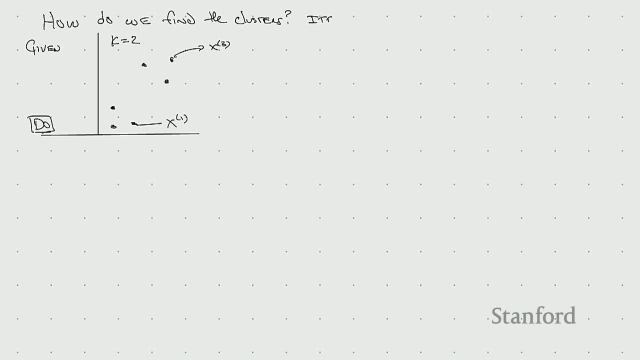 And let's see the most natural kind of iterative approach Here. okay, So how does it work? Okay, so, here's the idea. We're gonna start by randomly picking cluster centers, And then what we're gonna try and do is the way we're thinking about k-means is. 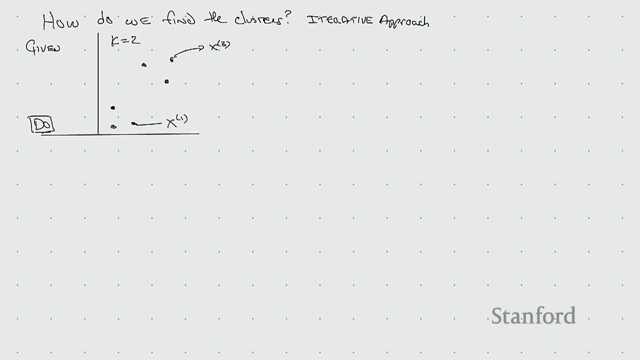 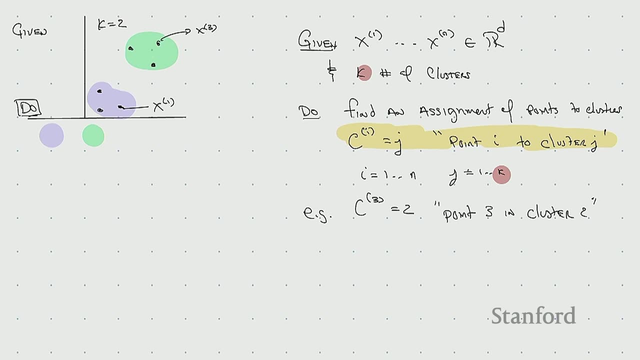 we're gonna try and find our clusters that are described by two cluster centers. So intuitively, let me just jump back. Sorry about this Jump back. We'll kind of try and find a point, say like here and a point here, that are good cluster centers. 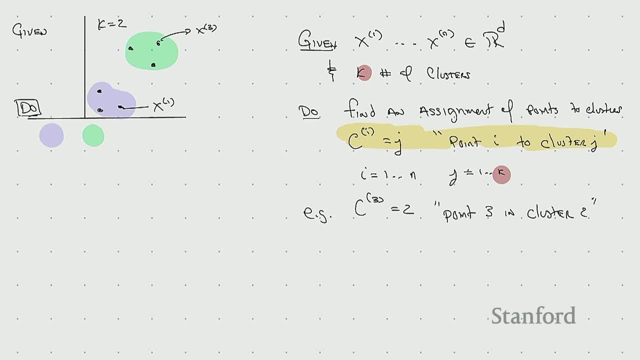 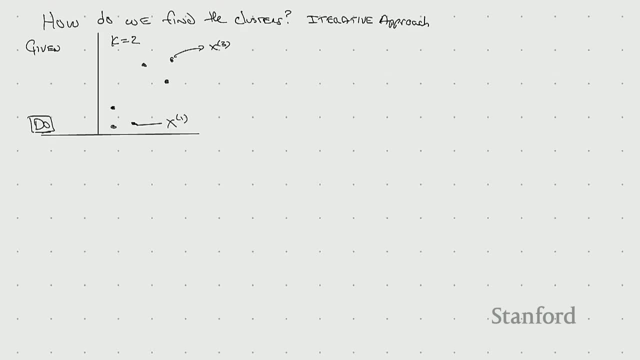 And they're cluster centers in the sense that all the points in their cluster are closer to the center than they are to any other center. Okay, And that's how we're gonna construct our CID. So we'll start by picking these means, The means. where are we gonna pick? 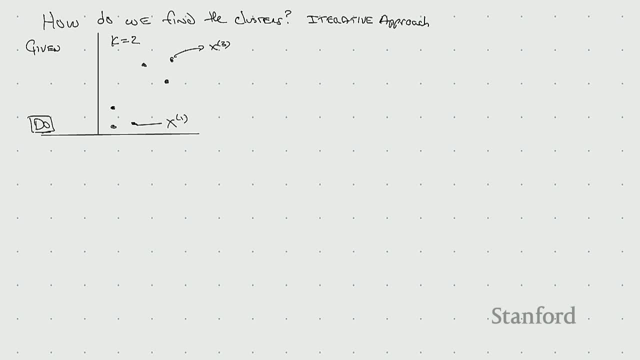 If we knew where to pick them optimally, we'd be done. So we just pick them randomly to start with. So I'll pick the cluster center for two up here and I'll pick the cluster center for one down here. Oops, I'm gonna use a different color. 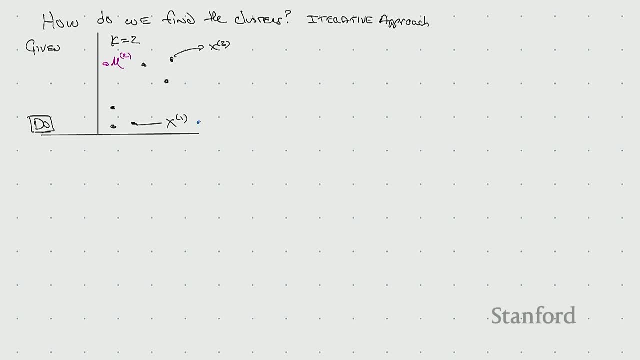 for deep-seated reasons? No, for no reason. I just like different colors. Okay, Sound good. So I just pick those points. Maybe I wanna move this one, just to make my life a little bit easier. I'm gonna delete that and drag it over. 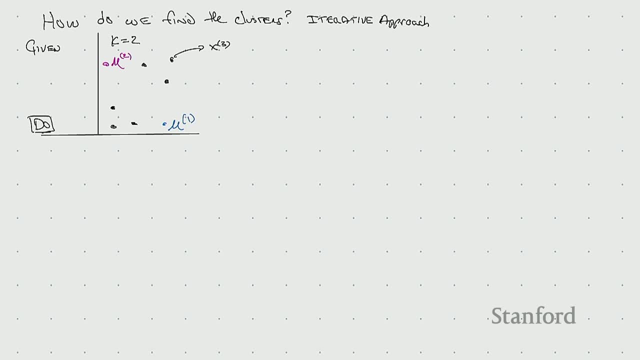 You say: why are you dragging it over? Because it's like a cooking show and I wanna make it just look a little nicer when I draw the pictures. Yeah, The list of points that we have, they can be-. No, these were not lists of points. 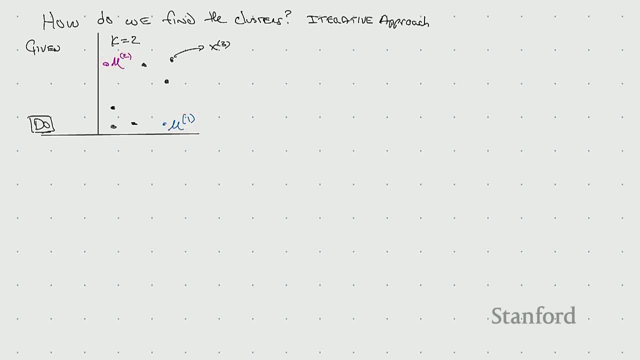 These are just two random initialized points in the plane. I just randomly picked them in RD. We'll talk about a smarter way to initialize them in a second, but just for the moment they're just random points. They are not points. They do not have to be points in that you were given. 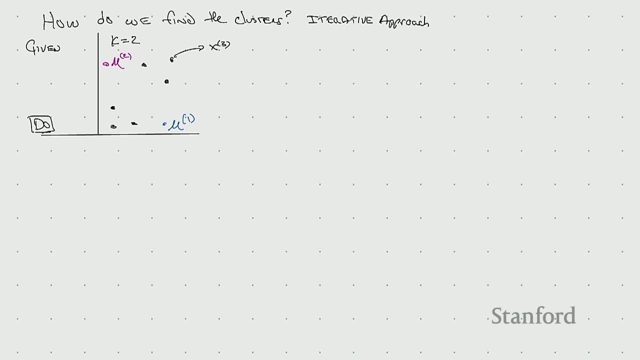 We'll talk about how to initialize them later, And you may not exactly wanna do that, but you wanna do something similar, Okay So, okay, so let's see how the algorithm runs. So the first thing is: what would the clustering be if these were the centroids? 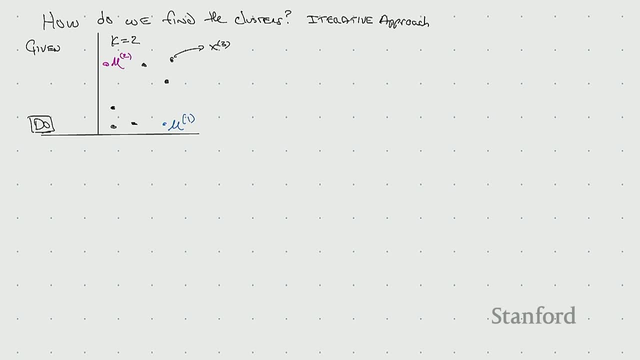 These were the center points. Oh, go ahead. Oh sorry, what is the name of the algorithm? K-means? Sorry, yeah, I wrote it above it. This is called K-means. Great question, Please. How do you? I guess this is a simple case. 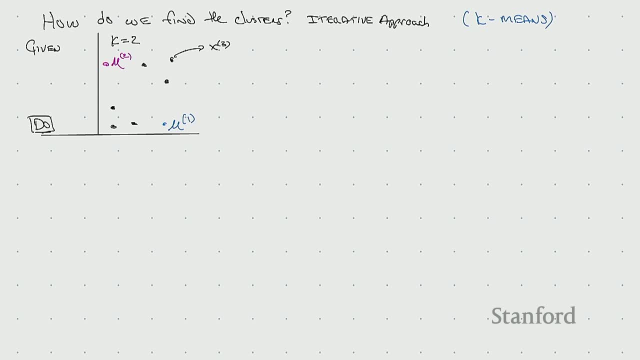 of the data. so how do you determine what K-means is? So, for the moment, K is gonna be given to us as input. We'll come back, as I talked about about how to select K in a minute, But let's run through the algorithm once. 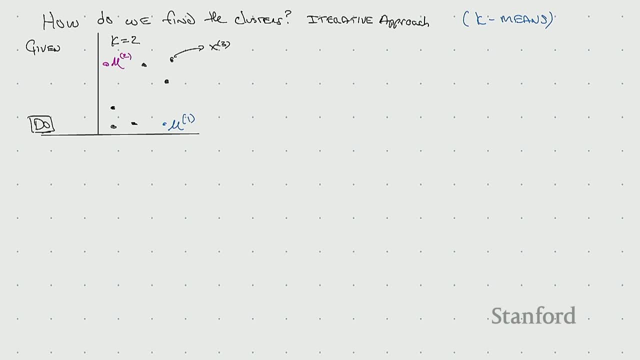 and see how it works. Then we'll talk about kind of what goes wrong and how to extend it. These are wonderful questions, really great questions. Are there others? Awesome? okay, We'll come back to that And please, both questions, please come back to those. 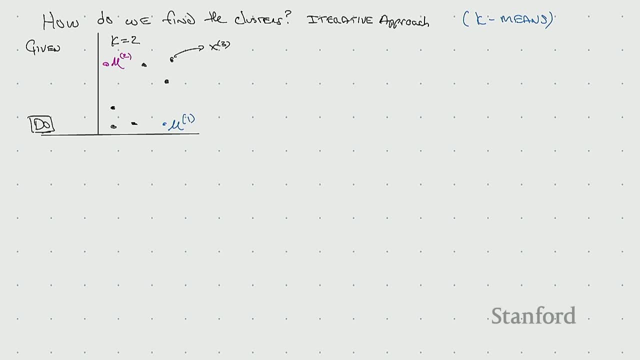 as I said. All right, so the first thing is we have these randomly centered cluster points. Okay, so this is our first step of the algorithm is that we're randomly initializing cluster points. Randomly initialize Mu one and mu two. 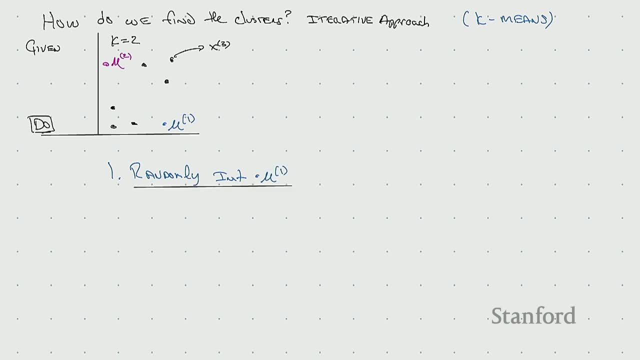 Copy paste. oops, got more than I bargained for. boom, And this one Paste. Okay, so we just randomly initialize where those characters live, okay. Two, we then assign each point to a cluster. Okay, and the way we do it is. 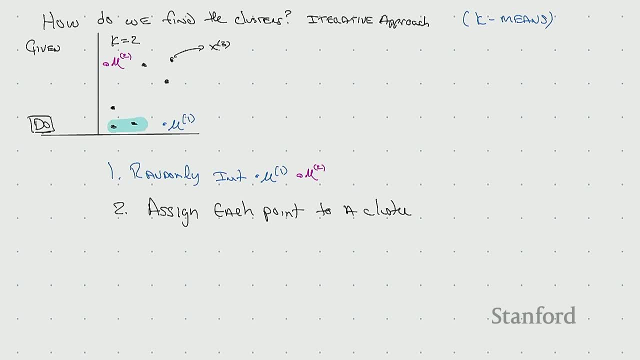 which point are you closest to? So I think you know if my drawing's- okay, those are all you know- closer to mu one, And maybe this one and these couple are closer to mu two. Okay, So you're clear enough what I've done. 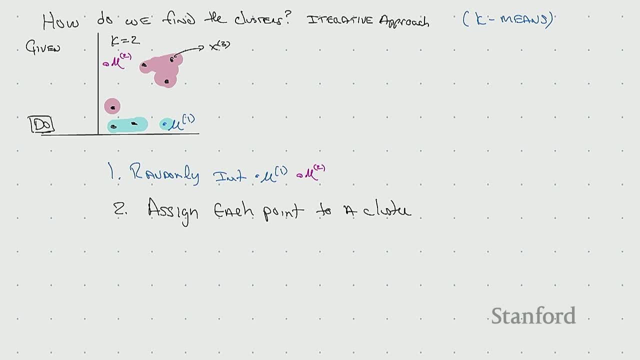 This is the cluster assignment And I can write it kind of mathematically in one second. If you'd like, I'll- actually I'll vamp a little bit and say how I did this. more precisely: Max over J, One to K. 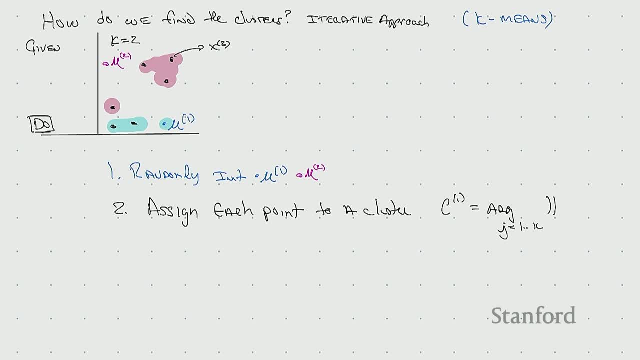 Min, oh sorry, min, arg, min C or mu. let me write this clear What's going on: Mu J minus X, I Okay, and I'm gonna put a square there, just because I like squares, Because we do it not really too problematic. 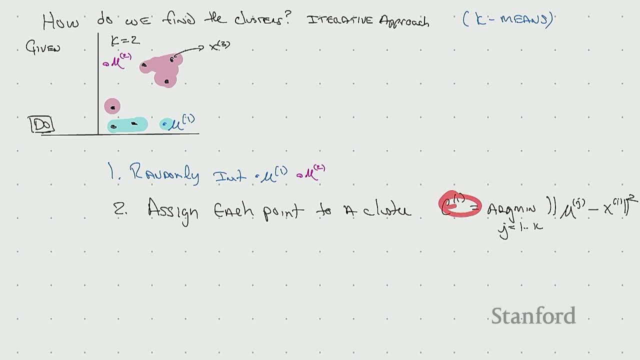 So, and they're the same distance. So this says C I, where I'm at and where I'm mapping the ith point. well, I just find the closest mu J to it, My current mu J. Okay, That's the way I'm doing the assignment. 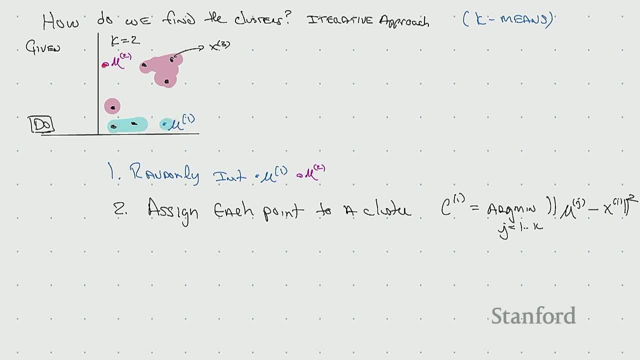 Every point goes to its closest neighbor And I'm like arbitrarily saying, this guy's closer than mu two. Alright, now I have to improve my clustering because, remember, it's iterative. So what do I do? I'm gonna copy it so you can. 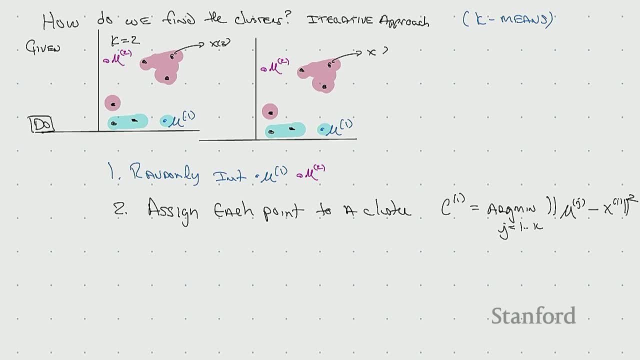 so I don't have to overwrite it. What happens? Well, what do you think I should do? I should probably take the points that I have and compute a new center. my new guess of the center is clusters. So what I do is I compute new cluster centers. 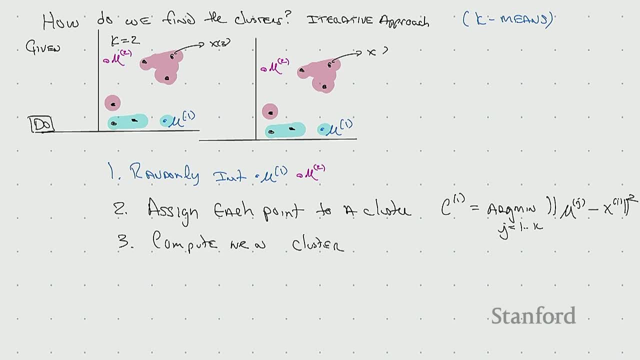 What does that mean? Cluster centers? So I'm gonna move. I look at mu here. What's the new cluster center for that? Boom, boom. Well, it looks like it should be somewhere here. Alright, this is where mu one goes. 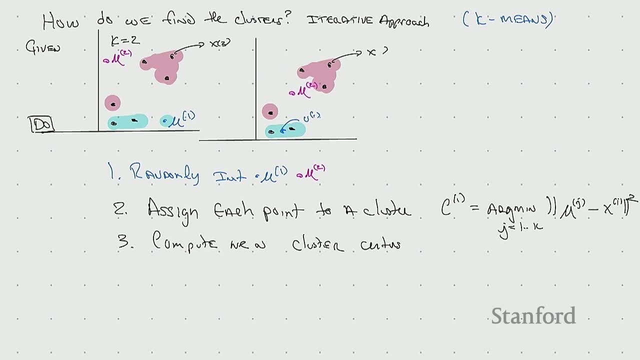 And where should mu two go? Well, probably somewhere right here, right, That's kind of the mean of them. Okay, So you can compute these things precisely, but I'm just drawing them just so you get an intuition, Okay, 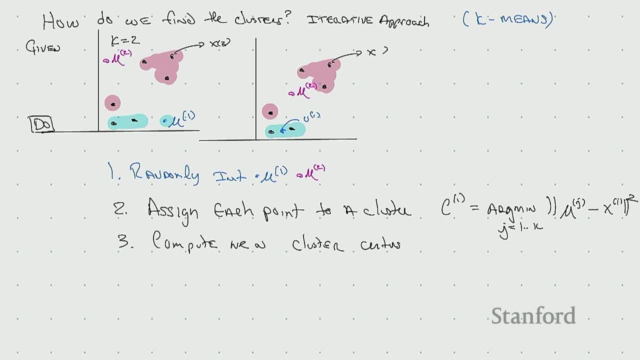 And I'll write this notation because there's more notation. So now I have new cluster centers. Now what's the next step? I repeat. So I go back and I assign every set that's closer to mu one or mu two. 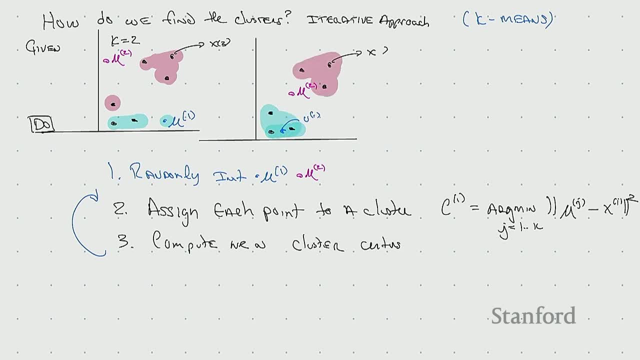 So now I have these characters and I have these characters there. Okay, that's what that's now doing. step two again. Okay, I repeat step three. What's gonna happen? They're gonna jump to the spot in the middle. 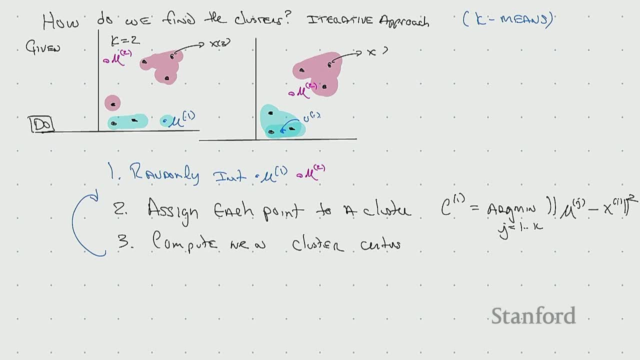 and the spot in the middle: Mu one's gonna be there, mu two, and then there's gonna be no more change. if I were to continue running the algorithm forever, Okay, So let me write that out mathematically while you digest that statement. 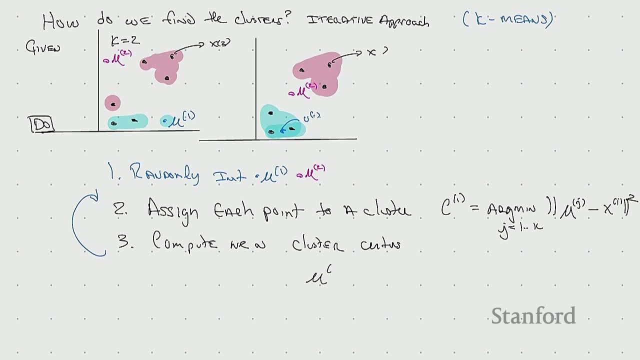 But that's the entire algorithm. Okay. So what does this mean? Mu j is gonna equal one over sigma j. It's gonna be some average over all the points in sigma j xi, such that sigma j is just the set of points. 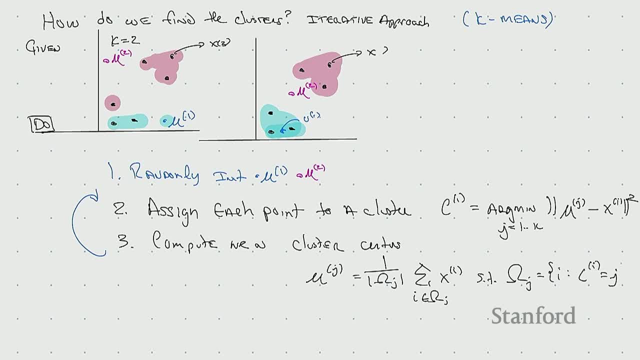 i such that ci equals j. Okay, This is just some notation that says these are all the points that are closest to the center j, And then I average over all of them. I just compute their mean, hence k means. Okay. 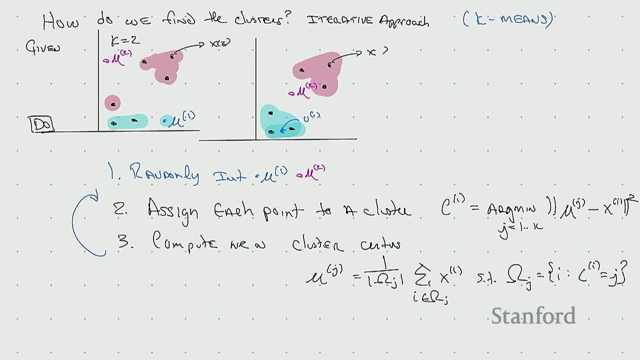 I iterate this thing and I repeat: until, until no assignments change, Until nothing changes. basically, Repeat: until nothing changes. Notice that if the labels don't change in step two, then the mean is not gonna change, because it's a function of the labels, right? 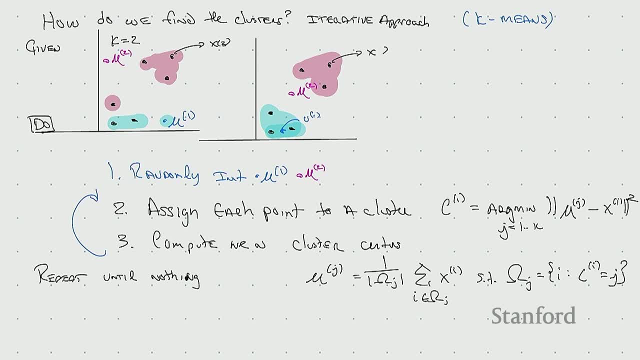 It's a function of what I guessed was in each cluster. It's always their mean. Any questions about that. Nothing changes. No, Yeah, Please, Yeah, In many, many and different ways. So let's talk about a couple of things that go right. 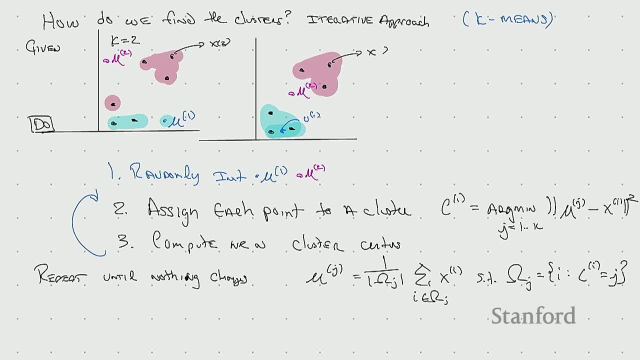 and then we'll talk about what goes wrong. So the first way it could go wrong is: does it terminate, right? So if you imagine it was in some, you know it's not obvious like I'm doing this kind of jumping around. 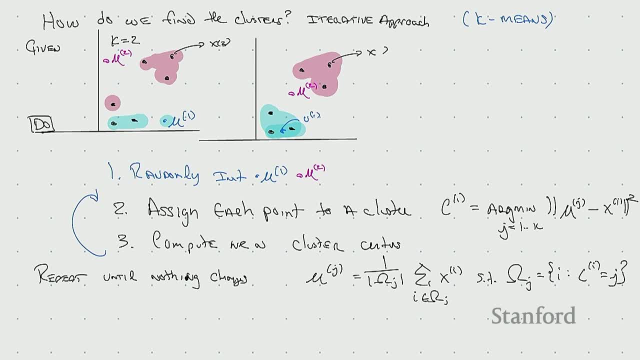 It could oscillate wildly right, Like there's nothing that like prevents it- at least at a high level, when you're thinking about this- of going like: oh, one switch from red to blue, then it switched back from blue to red. 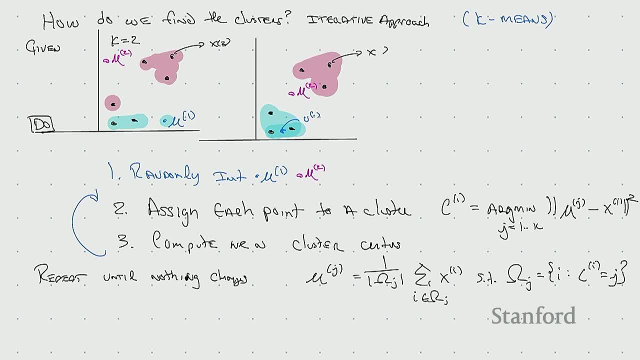 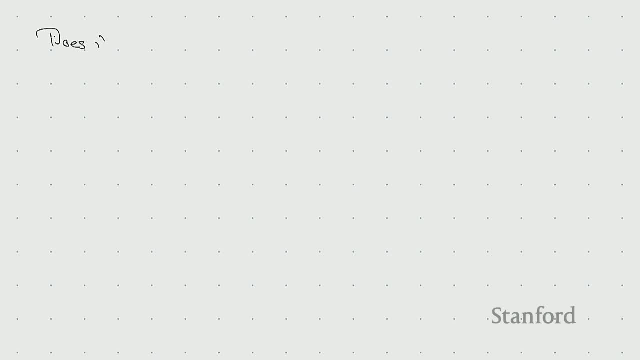 and then the cluster centers are like jumping around and they're in some unstable kind of equilibrium. So that's something that potentially could be bad. that happens. So that's the first question: does it terminate? Does it terminate? All right, And it turns out, this is great. 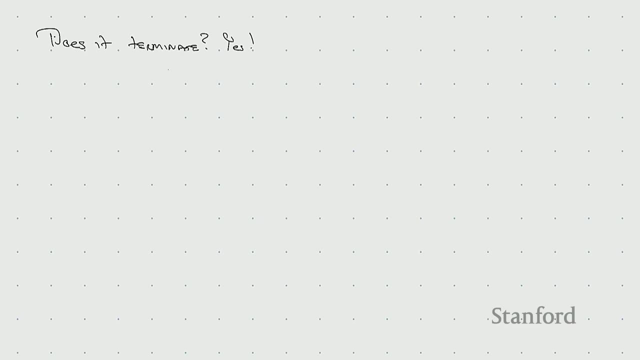 Yes, it does. Now, why does it? The reason is that this functional, underneath the covers one to n xi minus mu ci, that is, the distance between a point and its cluster center- is actually monotonically decreasing. Okay, it's not increasing. 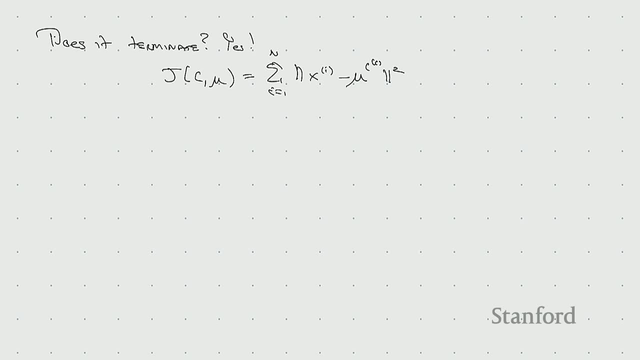 So that oscillation can't happen. basically, And you can basically view the algorithm underneath this k-means. if you really want to be kind of super abstract, you can view it as basically doing gradient descent on this object in a particular way. 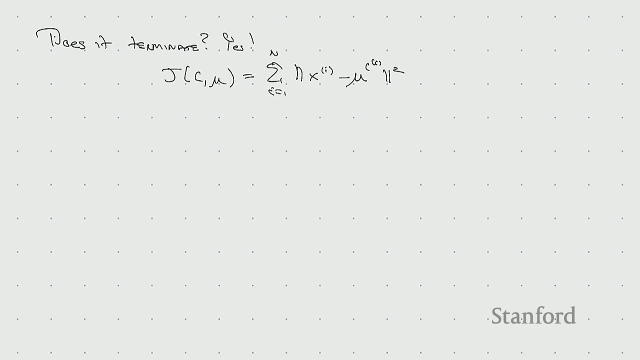 See the nodes for actually the convergence. So it converges to something. okay, Now, in unsupervised learning, that converges to something is about, as is kind of what we can hope for In particular. you may also ask: well, okay, it converges to something. 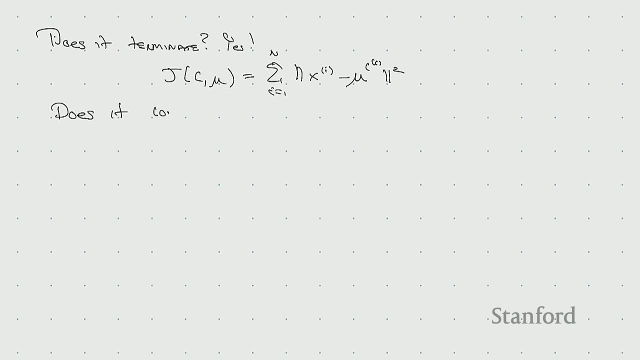 Does it converge to a global minimizer? Does it converge? Does it converge to global minimizer? And if I did my job setting this up, your intuition should say no, No, not necessarily. Now you may look at this and say: well, not necessarily. 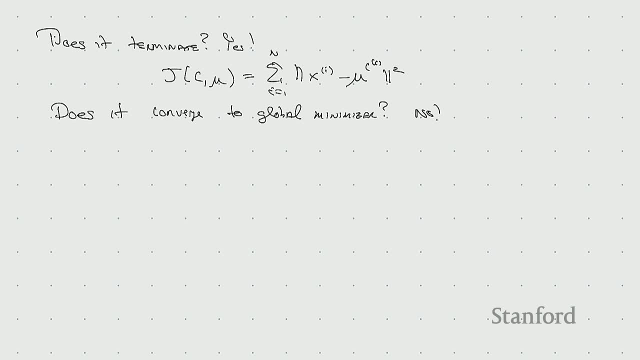 Maybe there's a better algorithm out there that, given this setup of problem, you just you know why did you pick this algorithm? It's a bad algorithm. you should show me a better one. There isn't a better one because it's actually NP-hard. 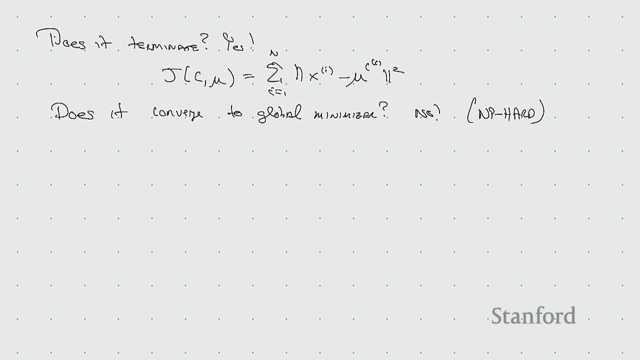 If you don't know what that means, don't worry. There's no hardness proofs in this class Does not really matter. It just means we don't know, like humanity does not know, a better algorithm for this that runs in polynomial time. 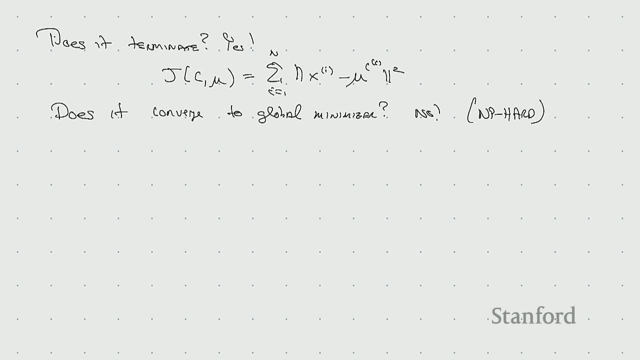 Okay, and we have reason to suspect there isn't one. Okay, all right. So this is this algorithm, as I said, like it's gonna run, but sometimes it can end up doing things that are, like you know, quite bad. 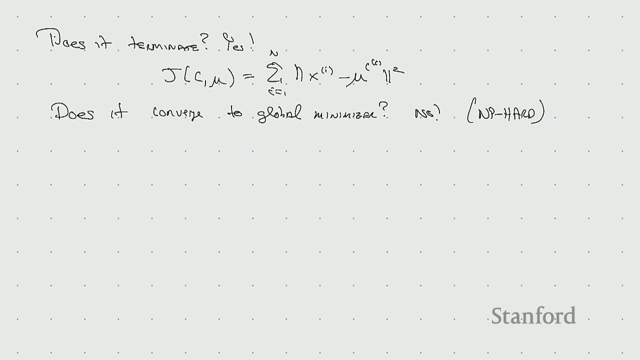 In particular, it gets stuck by, like getting a cluster over in a region where it should have never been. and if it like, had you know more carefully searched, potentially it could have gotten a lower cost solution. All right, clear enough. Clear enough on its properties. 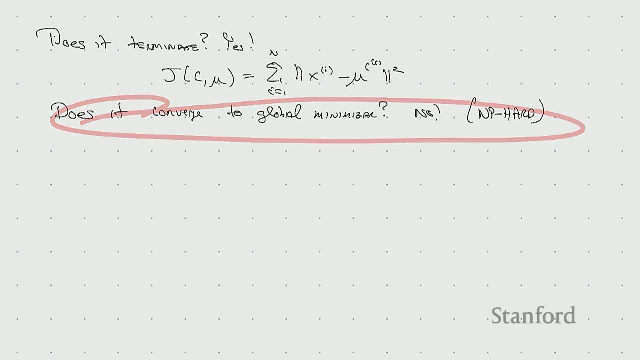 Now this: this is gonna be a hallmark of what we do over the next couple of lectures. Almost everything we do, with the exception of one algorithm that we'll talk about, has this property: that it doesn't necessarily converge to a global optimized solution. 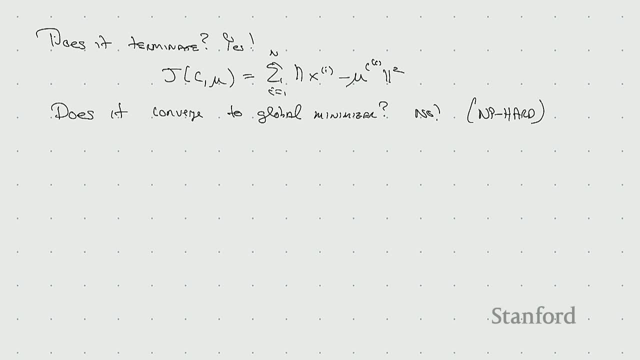 And, as I said, this used to be much more disturbing to people, but now most of AI is in that mode, so people don't seem to care as much. okay, Used to be quite disturbing. When I started, it was quite disturbing. 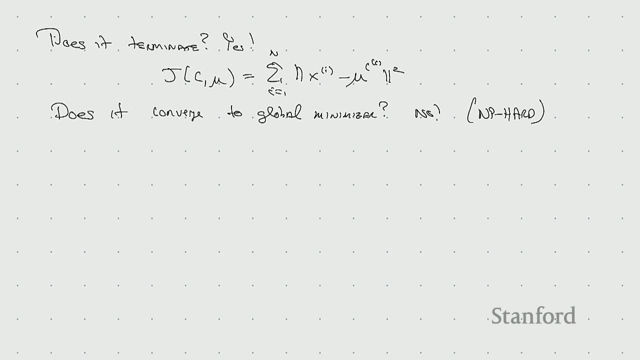 Now no one cares. You guys, you folks are old hats at this. Go ahead, What happens in that situation? So you can imagine situations. for example, imagine there are points that are really far away and then some other cluster of points here. 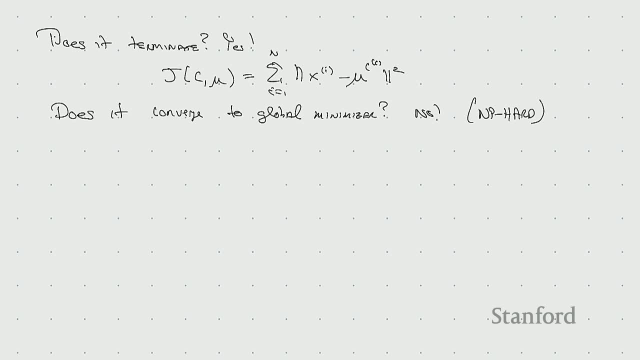 and that really there's enough kind of things in the middle that the optimal is actually closer to the line, Then what you'll see is that you could end up with some kind of local minimum where you pick a center way way over here and a center in the middle of this. 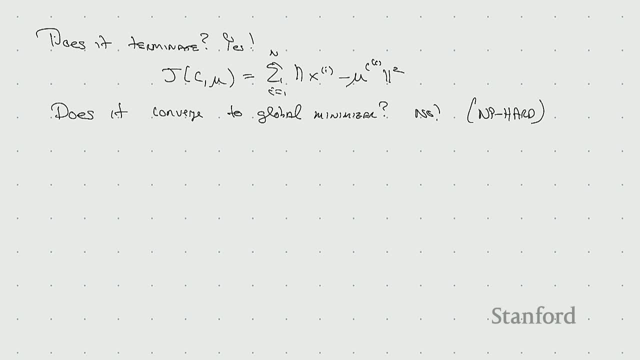 but you should have. there was kind of a better one closer, So that's very hand wavy. I can post some examples where you can actually run through and convince yourself All that I really care to get across in this lecture and I couldn't think of how to get good examples. 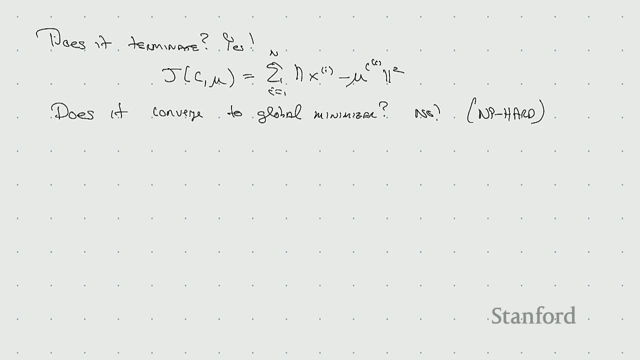 to look at there is that this is a possibility. You shouldn't expect it to get you a global minimizer, and we have some theoretical reason why we don't believe such an algorithm could exist even in this simple case. Yeah, wonderful. 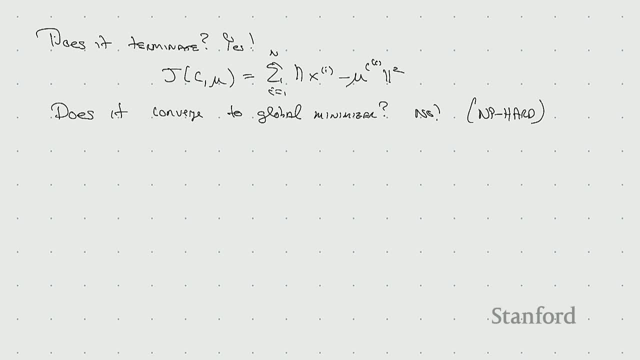 Okay, now couple of side notes. So these questions already came up, so these are really great. So they're not even side notes, They're just responding. they're just being responsive, but I was gonna talk about them, no matter what. 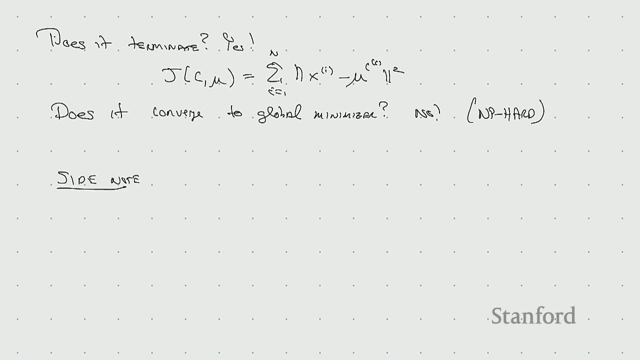 The question was asked: how did you initialize right? How did you pick these points? And from my argument, as I just talked about, even very intuitively and informally, the initialization matters quite a bit right If you initialize way, way in crazy ways. 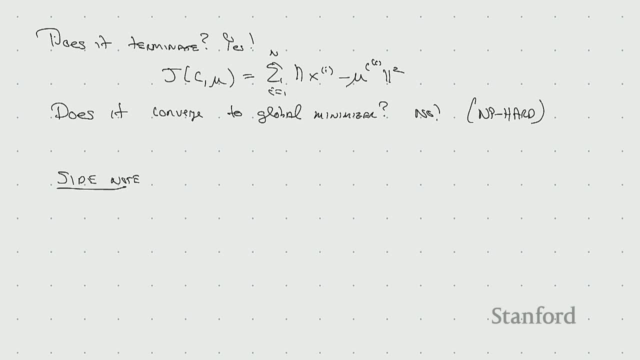 then you force K-mean to kind of jump back and maybe there's only one point, Like imagine there's a cluster of point and you throw one of your centers way across the room. it's gonna potentially pick off nothing and then it's gonna have to kind of crawl its way back. 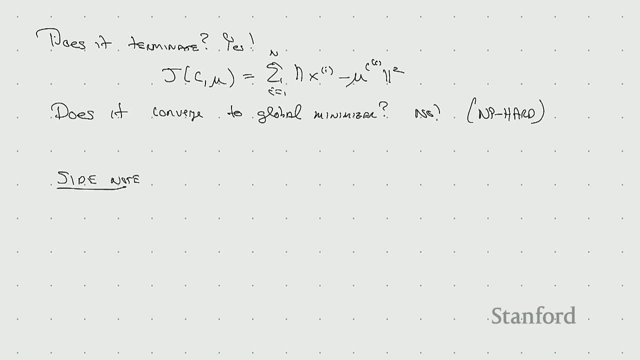 in some sense. So the point that I care about you getting is: how does the how does initialization matter? And I won't go into too much detail, but I wanna tell you that there's one algorithm that was developed by smart Stanford students a while ago. 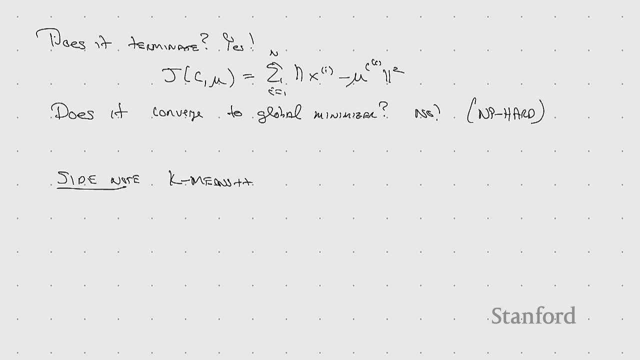 maybe 12 years ago, I don't know, 12,, 15 years ago, maybe even called K-means plus plus. And I'll just tell you what they did from great Stanford students And basically what they decided to do is that they, where they compute kind of a density estimation. 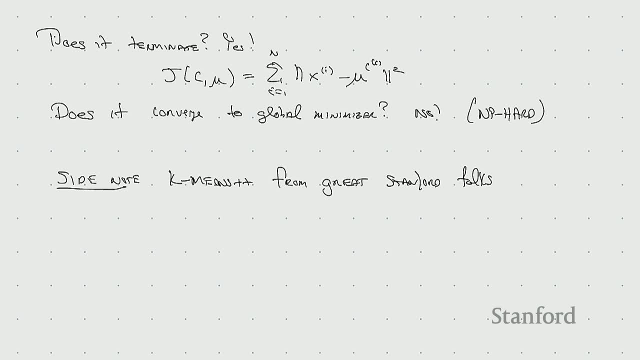 and then they place their centers with respect to the density, to kind of spread them out in a nice way in K-means plus plus, And without going too much into the details, what ends up happening is they get an improved approximation ratio. So if you don't care about this kind of theory stuff, 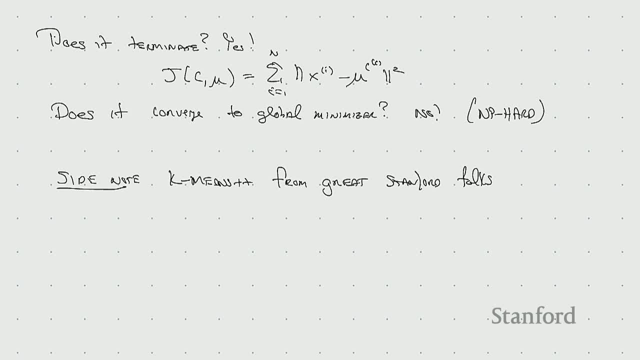 don't worry. But they're able to show that if you initialize in this way, even though it's NP-hard to find the exact solution, they can find kind of a low-cost approximate algorithm to it provably. So this is actually. 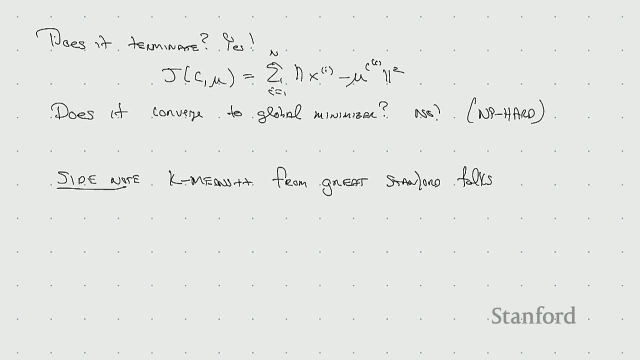 when we're talking about what could go wrong. this is something that can go wrong, And what people do in K-means is they used to just kind of run it many times. but if you run with this initialization, it's still a random initialization. 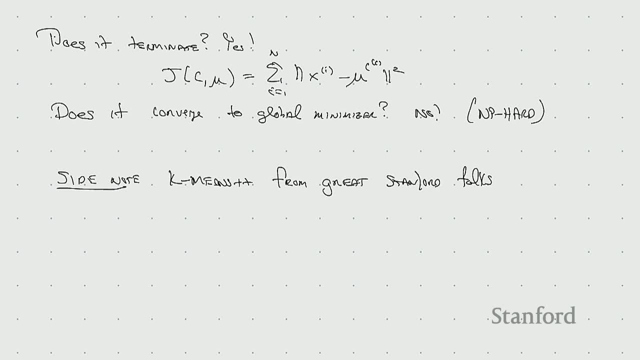 but if you run it a couple of times you're gonna get a pretty good solution. And because you're already kind of looking for an ill-defined kind of objective, that turns out to be about okay Now, weirdly enough, like I used to, as I said, 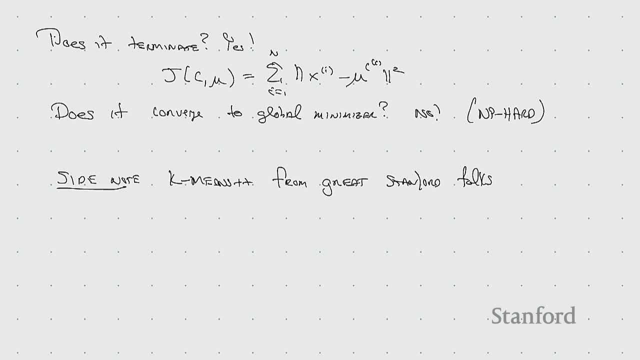 I didn't really like this stuff, but I wrote a paper about using some of it inside some of making these machine learning models robust, maybe a year or two ago, So it is something that I've actually used and care about Like it does work. 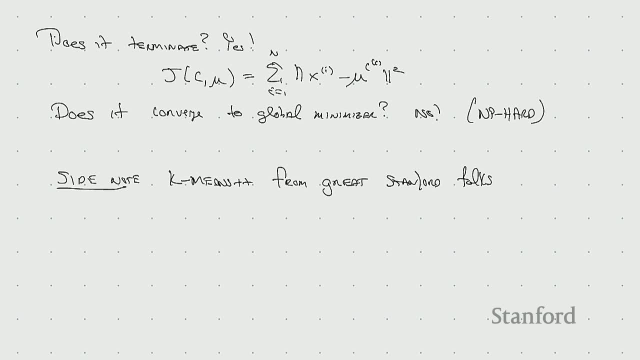 And you use it as a way to inspect your data. often, Like you don't, you look at your data set and you kind of do your K-means clustering. then you can use that to figure out, like you know, what are the different groups that are inside. 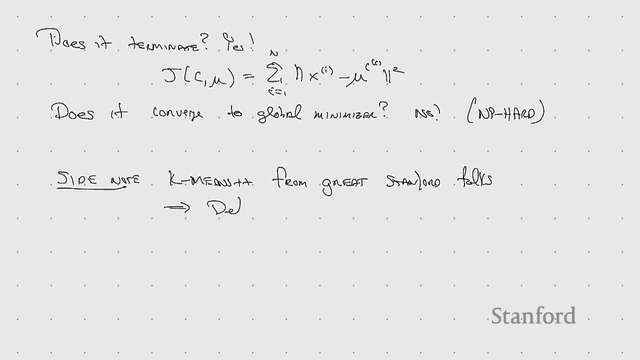 Okay, All right. this thing here became the default in scikit-learn and sklearn. So these folks wrote this beautiful paper. They proved this nice result. And now, if you run a scikit-learn and run the K-means algorithm, 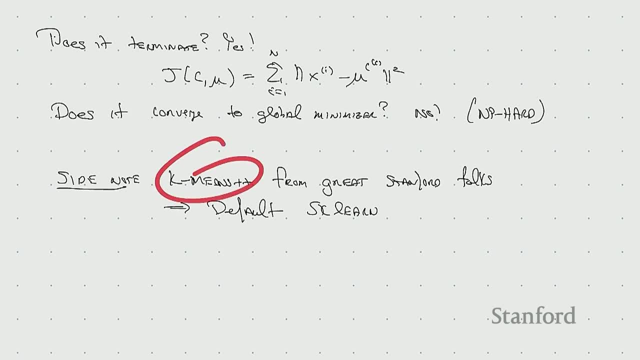 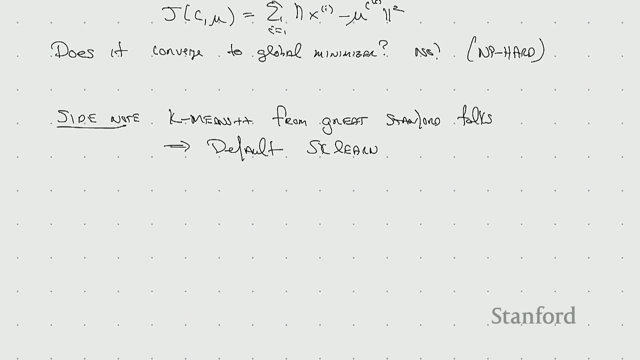 it defaults to using the- excuse me, defaults to using the K-means++ initialization. Okay, so pretty fun, Sergey and folks did that. Anyway, all right. So now there was another question, which was okay. how do you choose K? 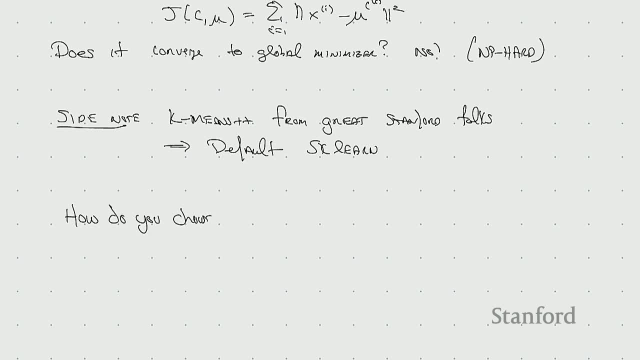 Right, this came up both in the ed thread and it came up in the lecture hall itself. How do you choose K? And here's the problem with choosing K: There's no one right answer. We'll see other unsupervised algorithms which do give a right answer. 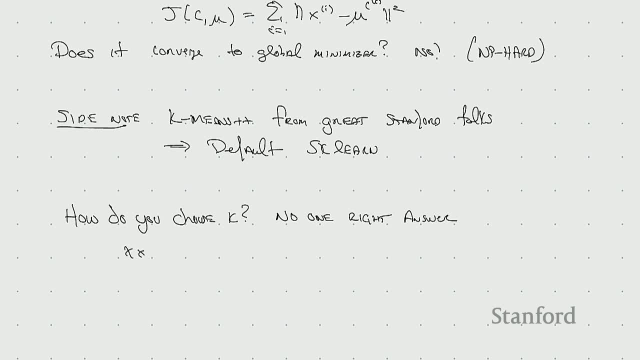 But let me just illustrate this for you for one second. Suppose I give you this, Let me just illustrate this for you for one second: Data set, Okay. Okay, there's two copies of it. One reasonable clustering is this: Two clusters. 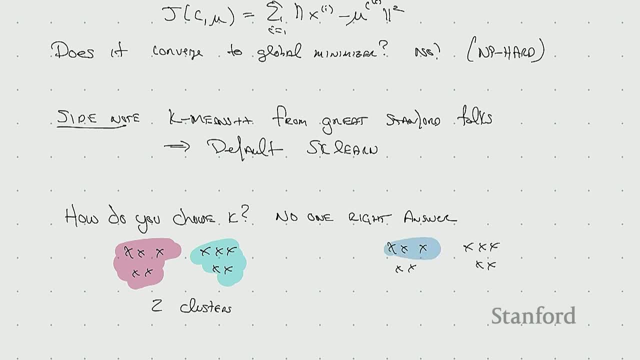 Equally reasonable, excuse me, is this one Four clusters. Now, if you think about the algorithm as giving you the right answer of what structure is inside your data, then you really don't like this answer. Say, well, what's the right K. 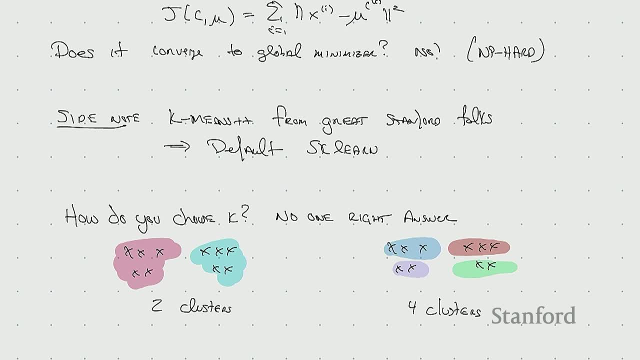 Well, it's not the right way to think about it. maybe The right way to think about it is: given that you have a K, can you use this as a tool to find the clusters that are in there of different sizes? So, if you're looking for five clusters, 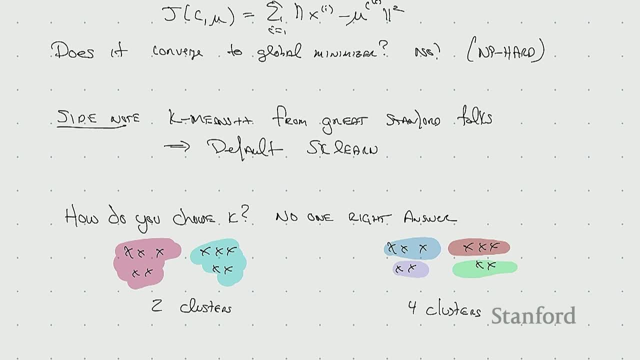 and you really only found. you know you look at the five cluster and the four cluster map. you have to make some judgment about kind of which one is better underneath the covers, And that's why unsupervised learning is kind of squishy. 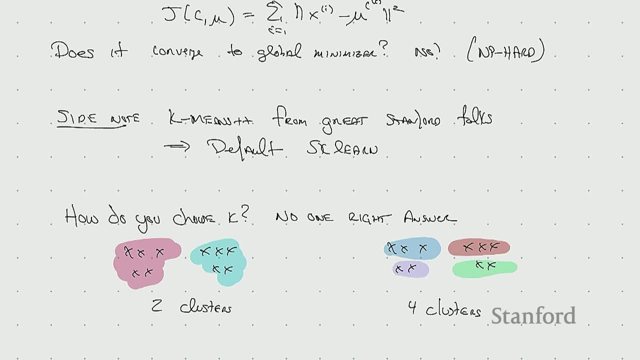 but it also turns out to be tremendously powerful. So we can automate the loop of finding the clusters, but you know which one is good or bad? you're gonna have to use domain knowledge for that in most situations. Okay, All right, so this is really another way of saying. 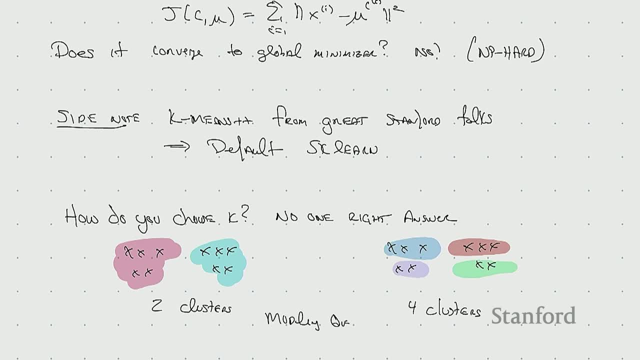 this is a modeling question, So the one part you know, even when I didn't really care for. I don't know if I'm telling you the history of how I feel about lecture 11, but, like you know, you're getting it. so 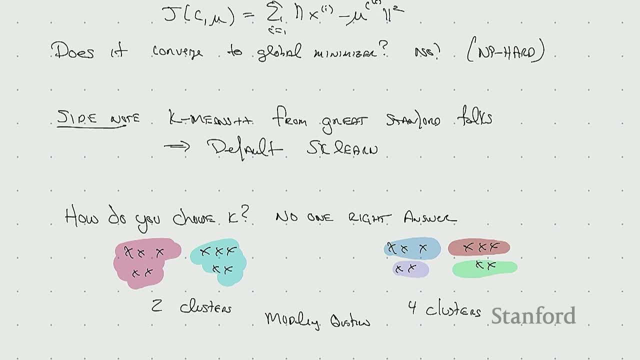 But, like one of the things that I did like about this lecture always, or this part of the course, is that it forced machine learning folks to move out of the comfort zone of like there's a right answer and optimization will find it, which was very disturbing to me. 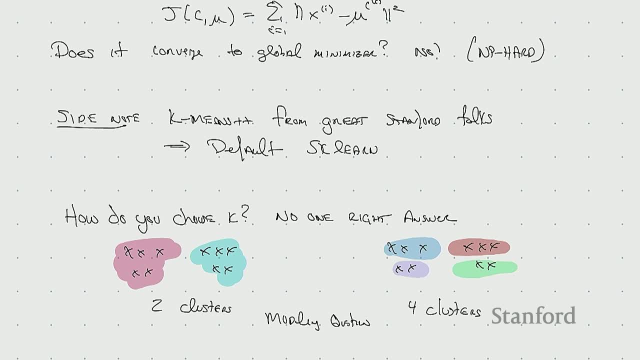 because that's not at all how machine learning works. in what you're doing, You're constantly in this regime where you're checking if your model works or breaks or does things. I don't know how much Tegnew subjected you to my crazy slides. 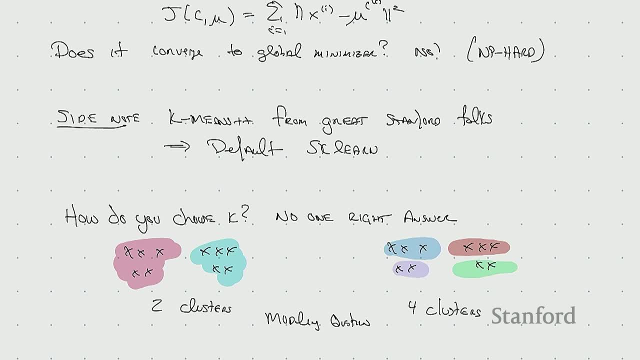 but like that is the way that you live when you're building these kind of ML systems. Like you build a model, you have no idea if it worked. You have to check it, you have to look at it, you have to inspect it, you have to measure it. 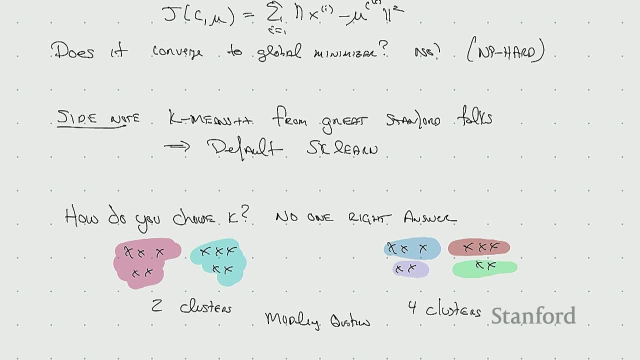 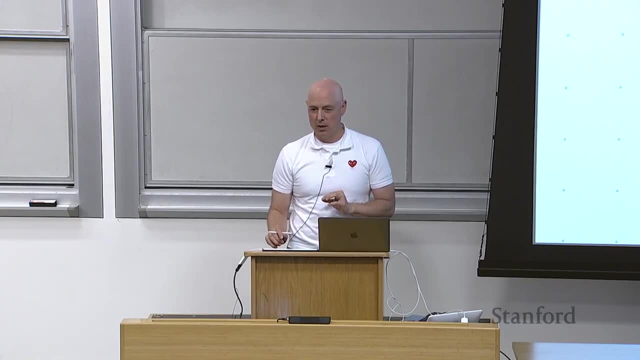 So this is kind of natural and at least forces you to do that. Okay, that's all I wanted to say about key means. I want to jump to the next algorithm, which is building towards this larger theory of what we did. 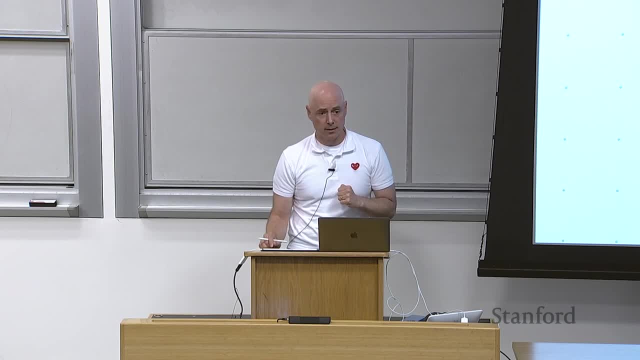 And if you can kind of squint, you'll see that it parallels how we taught the supervised learning case. But any questions before I move on? Awesome, Please. Is this something you might use if you're doing supervised learning but with labels that you're unsure about? 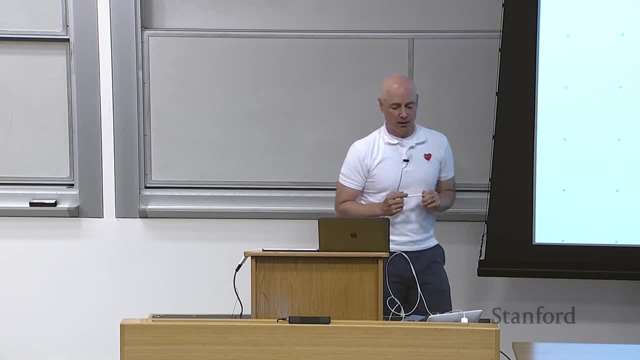 Oh, awesome, Yeah, great question. So let's say that you're unsupervised. So the way we were actually using it is exactly in that way, in this paper, What we were looking for. I'll just to be really concrete. 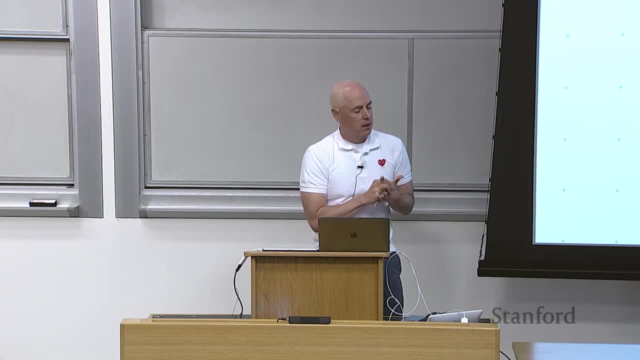 is. we were looking for what are called hidden stratification. So these are times when a machine learning model- let's say that it's classifying birds that are on the land versus birds that are in the water. I have more elaborate examples than this. 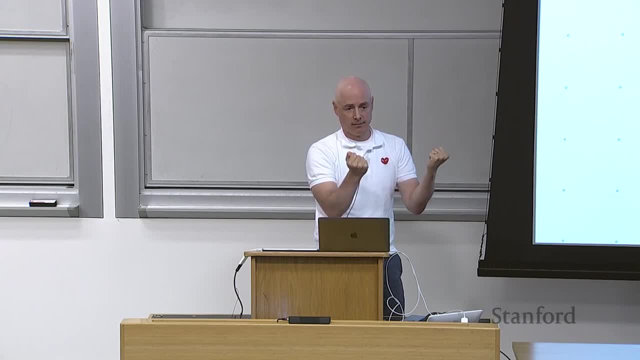 And it turns out that the model sometimes gets confused by the background, And so what you want to do is you want to cluster some notion of those feature descriptors underneath the covers of background descriptors that the neural net has learned, to try and find a group which kind of looks: 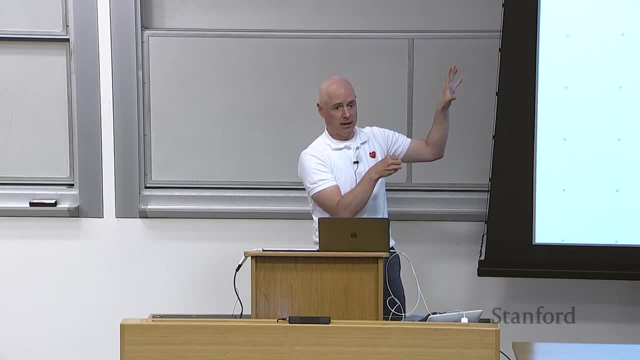 like an oddball from the rest. So it's like: oh, here's all the land birds on land backgrounds. I got them all right, And there's this other weird cluster there that I labeled as land birds but actually are water birds. 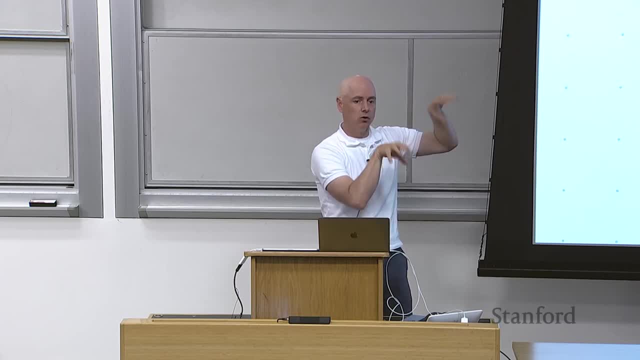 that happen to be walking on land right, And so that's the kind of thing. you look into your labels, or your pseudo labels, or your predictions and try and find those. They can either be labels that are given to you by a human or a neural net. 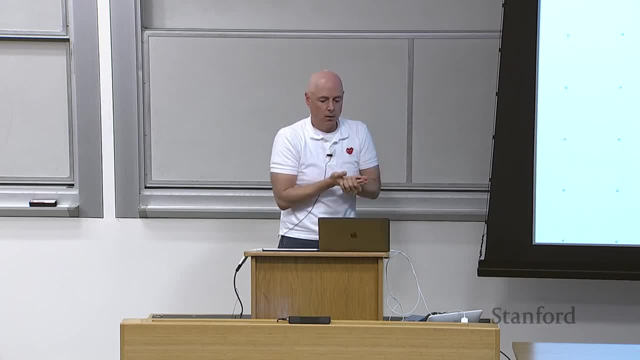 And that is like that was the use case that I had is exactly what you thought about. Yeah, so that's one of them. You'll typically also run this when you have- honestly, when you have- data you don't really understand. 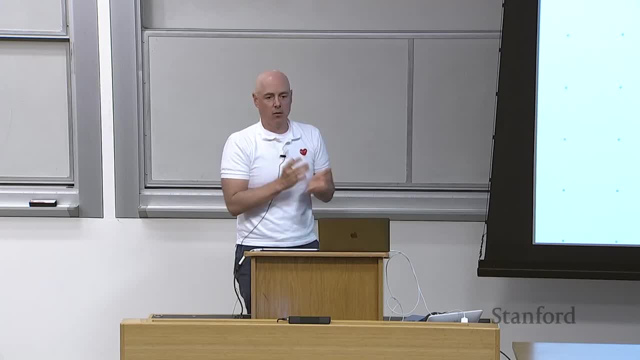 So you run an experiment with search traffic or ad traffic or something and you're like: what the heck are people asking about in this segment? And then you run kind of a clustering to figure it out and say, oh, this looks like a topic. 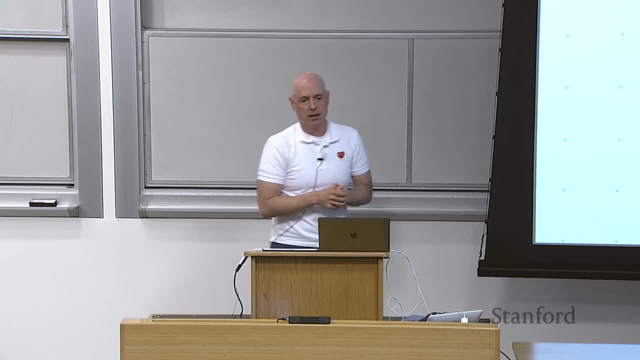 that people are talking about X, Y or Z, right? So those are the other times that you use it. But noisy labels is a good thing and that will be a theme for next week's lectures. Great question, Thank you. 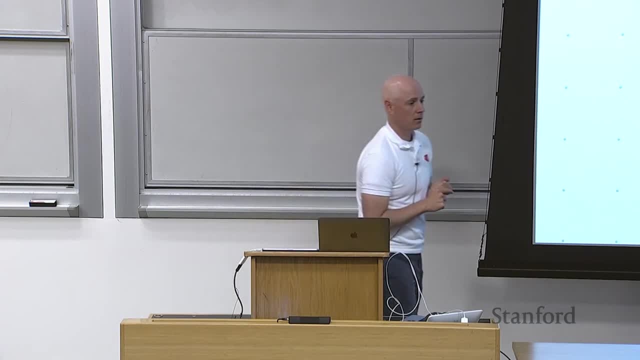 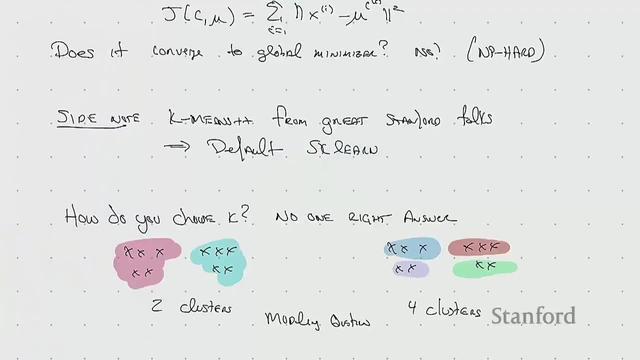 Please. Yeah, so the question is, if you pick a larger number of clusters, then, like if we go to this example here, the problem is how descriptive does it get? So in four and two you could kind of eyeball the two and the four and link them up. 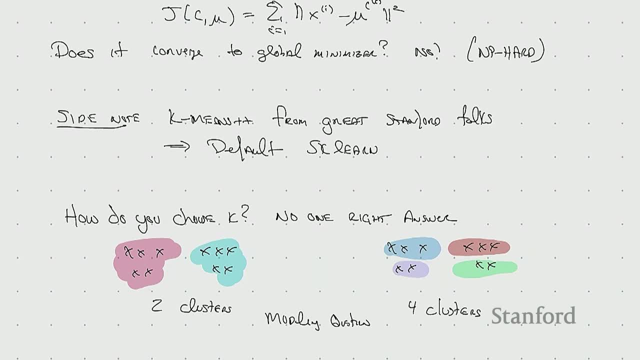 But if you start to really jack K up to like 1,000, then it like is like kind of at the brink of what does it mean to find meaningful concepts, right? So if you're looking for 10 things- and you know there are 10 things- 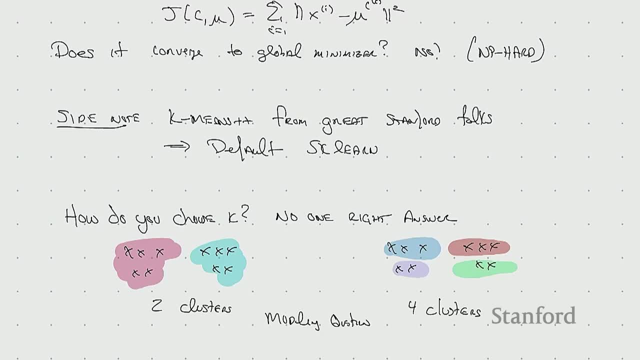 you want to find those 10 best groups. If you start to jack it up to 1,000,, 10,000, it no longer becomes like human digestible. So that's where the modeling thing comes in. It's kind of like the bandwidth. 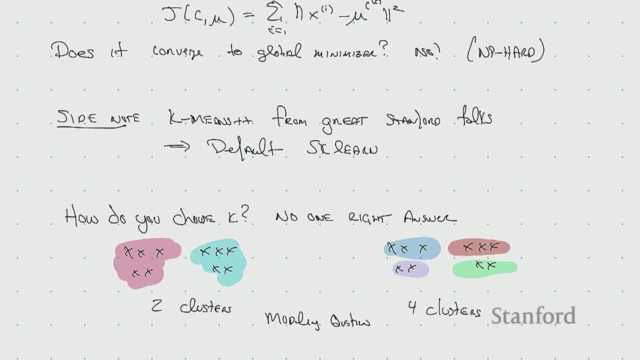 of what you can look at and do this And traditionally K-means was not used in an automated loop. It was traditionally used as, like, a way to browse your data. If the consumer of that is some neural net in the discussion we were talking about. 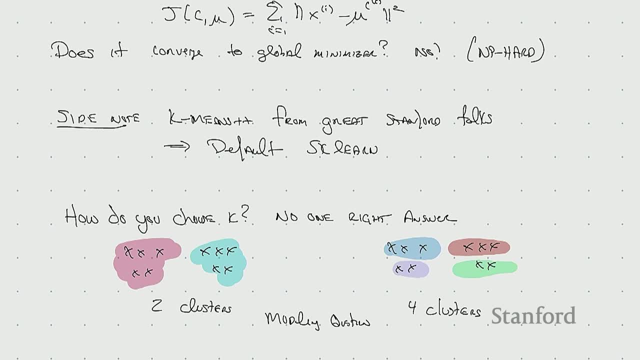 then it kind of doesn't matter. You can jack it up a little bit more. The advantage of doing so, the advantage of doing that- is if you put too many centers, they may be too close together And sometimes what people do is they'll just do. 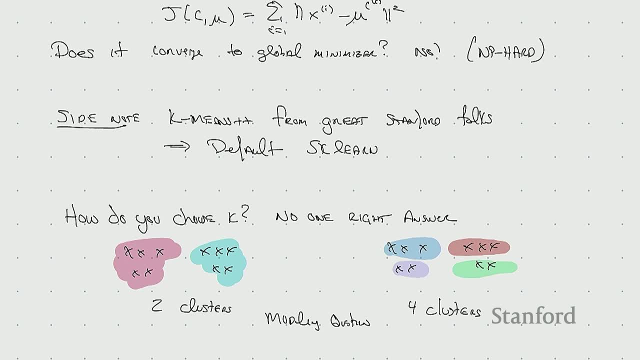 a kind of a follow-on path where they merge some cluster, Some clusters that look like they're kind of not informative, a pruning heuristic at the end. So your intuition is dead on And like that's the side you want to err on. 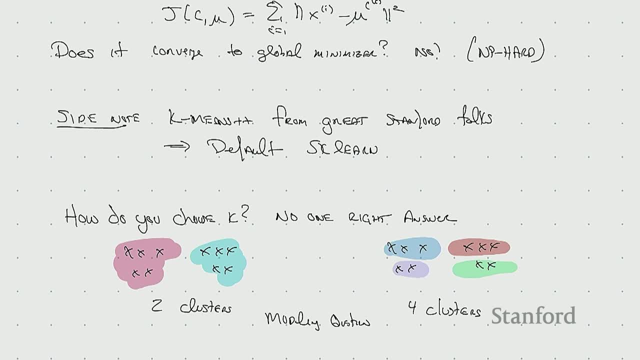 If you err on the side of two small clusters, what happens? You lump two things together that you could have distinguished and then you could get like a weird cluster in the center. So clearly you're right. The over-provision setting is much nicer. 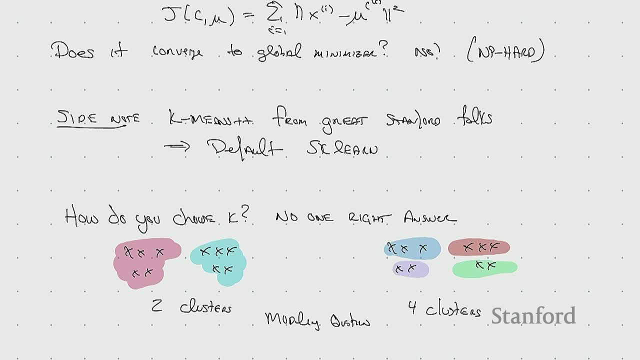 than the under-provision setting. Awesome, Sounds like folks got it, Please. Yeah, so I wish there was one algorithm. So this is something that, like, people are writing, still writing research papers on. We had an iClear paper on. 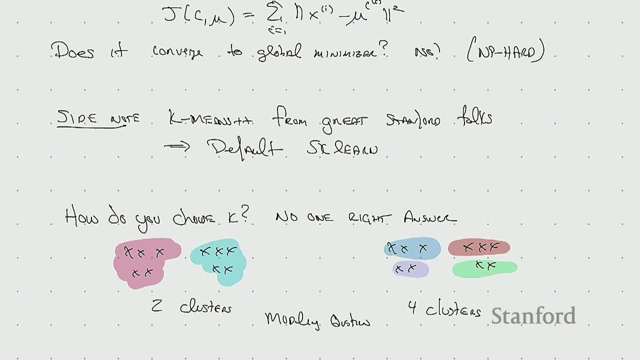 There's another one coming out from some other, from another group, which is great that we're reading right now. Basically, what people try to do in these things is that data point. So this is kind of an impoverished setting right. We have data points that are just in Rd. 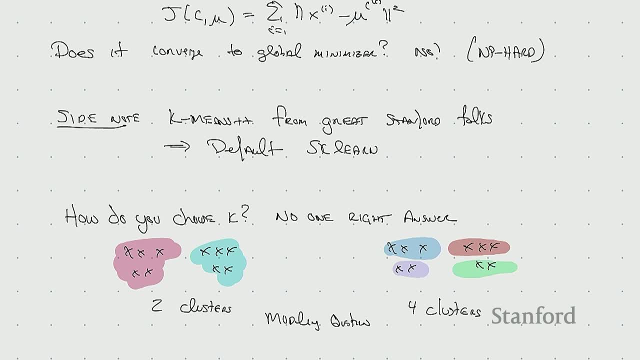 that are in a vector space, But those data points usually correspond to something real, Like there's an image or text. And so the more modern ways that people do with this diagnosis, like what Sabree, and and, and, and and. 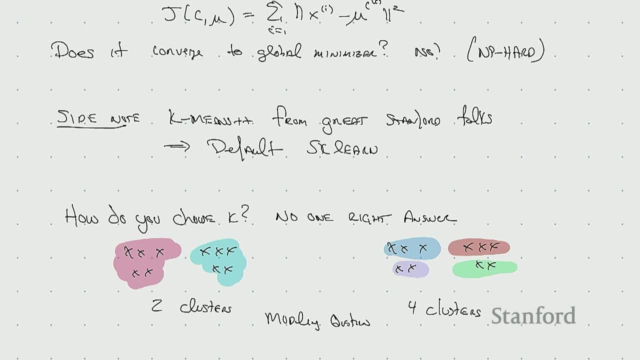 and folks did in and Maya did in in Domino is. they said, oh, we took those points and we embedded the text that's associated with an image and the image itself And we start to like do kind of search queries on top. 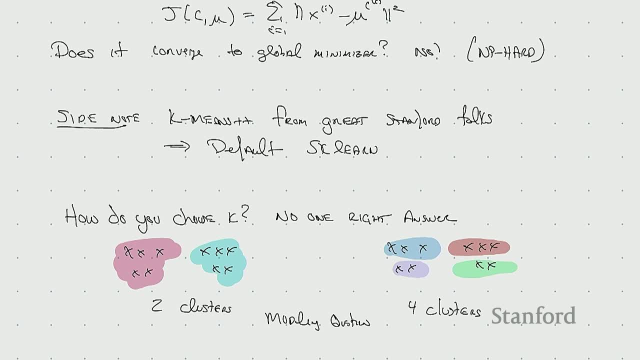 to find the slices that are underneath the covers. So this is the purest setting where you're just like I have data from in a vector space. But, of course, like with modern methods, like there's an underlying object, It's a transaction or an image and a caption. 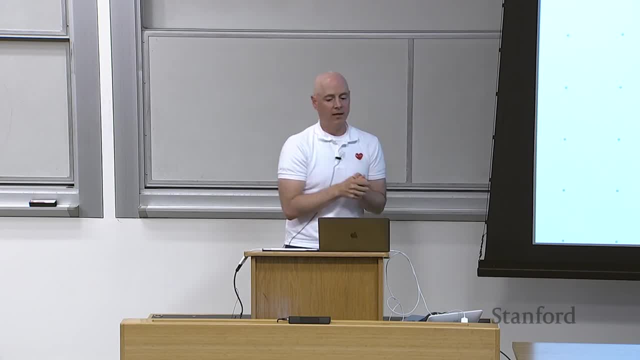 And then you start to use some of the more modern techniques to search through it, And then, of course, you visualize it or monitor it, And there are a number of tools that are out there to do this. I wouldn't say it's solved. 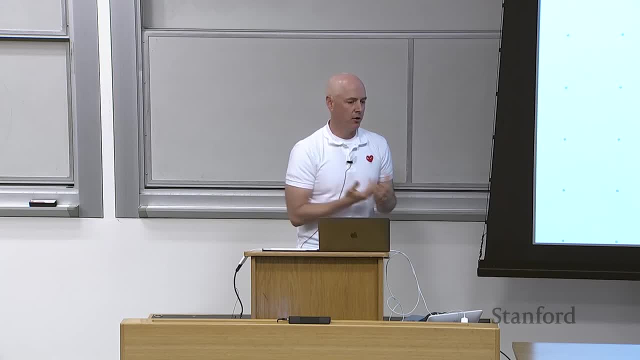 Like, oh, you just use X and you're done. But you know there are a number of tools, But yeah, you do have to look at your data. Like there's nothing that really obviates that. Awesome questions. 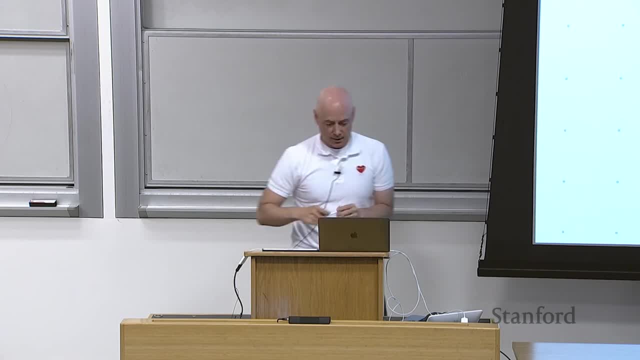 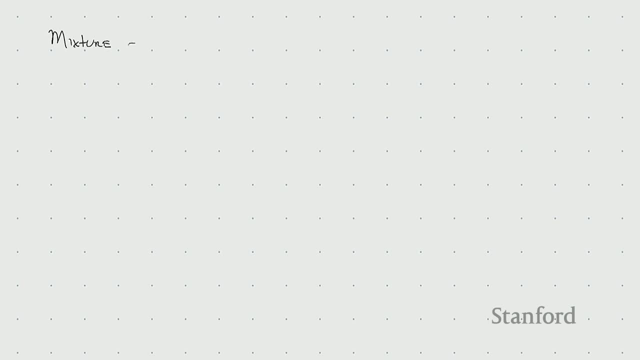 All right, all right. So let's talk about a slight, what appears at first to be a slight generalization. Hopefully it feels like we just relax one little thing, but it gets us closer to a more fancy model that will allow us to do some really fun stuff, okay. 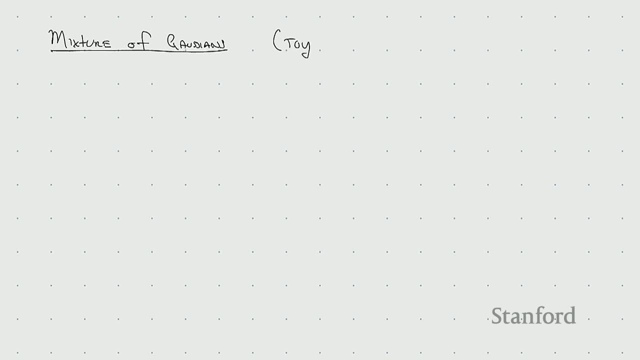 And this is actually pretty fun. So this is a toy example from astronomy, And if you know about astronomy, please don't humiliate me too badly. Feel free to correct me. I have no idea what I'm talking about, But I read the paper and I understood the math. 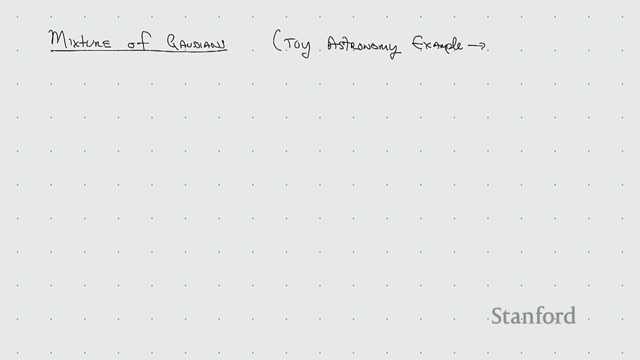 So who cares? So it's a toy example, okay, And it's from a paper from the University of Washington, So I can find the paper again if people are there, okay. So here's the general setup of what they're doing. 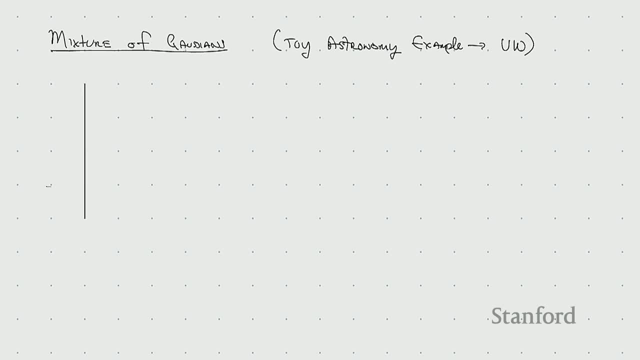 They have this light detector, this photon counting thing And they're looking in the sky at various different things, And what they wanna do is they have in this simplified model, there's kind of two celestial objects that could be out there. It could be like a regular star and a quasar. okay, 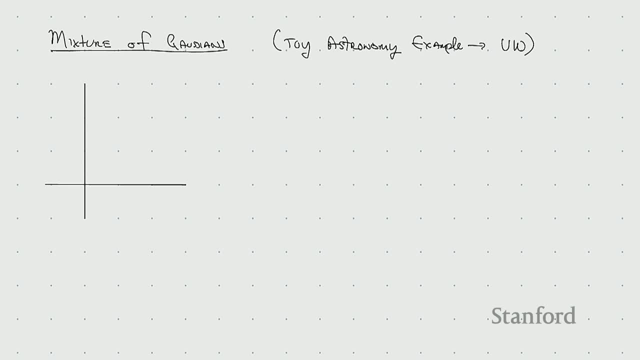 And one of them is gonna take the light and it's gonna spread kind of evenly in all directions, And another is gonna send out relatively concentrated pulses, okay, And what happens is, unfortunately, when those photons come to Earth, they don't come with labels. 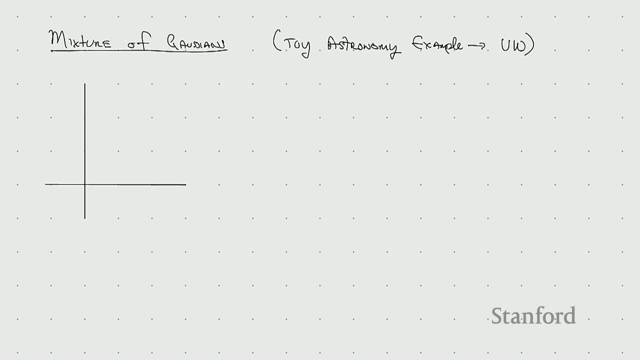 No one gets to affix a metadata packet to every photon that hits us. We have to see the photons and figure out, like, where the hell do they come from? okay, So what happens? we get some data that looks like this: 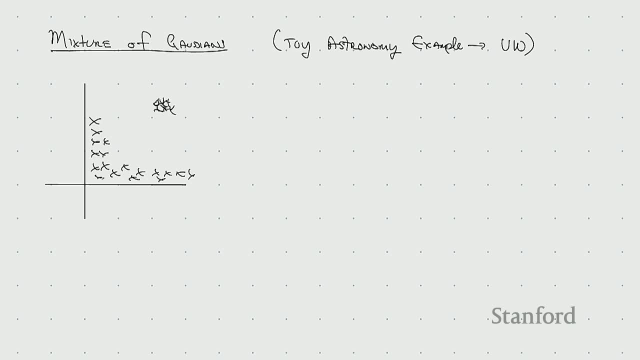 Maybe like this: Okay, And these are all our little photons that are there, okay, So you know quasars and stars, Now, okay, and both of these things emit light, but all we get to observe are these photon hits. 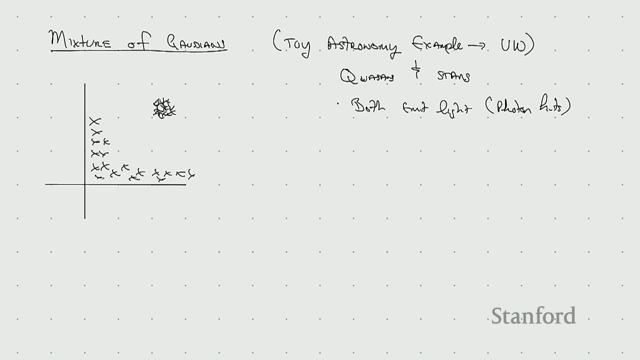 Okay, all right. So now what we're going to do in our oh, please, go ahead. Oh wait, No, we don't have to assume a linear decision boundary. We just have to assume that it's close in distance, right? 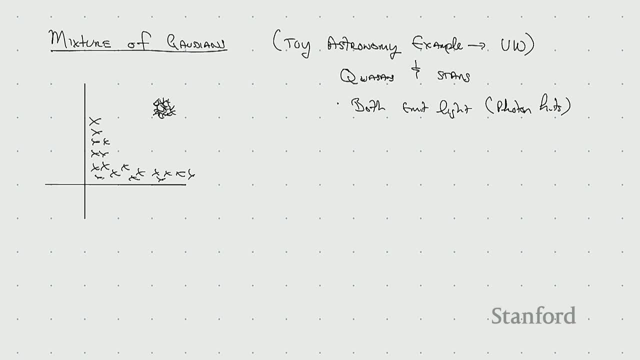 You can get nonlinear Right. there's no notion of a decision boundary in particular. anyway, Like you can draw like a little Voronoi diagram, but we didn't talk about that. Yeah, very nice question Awesome. 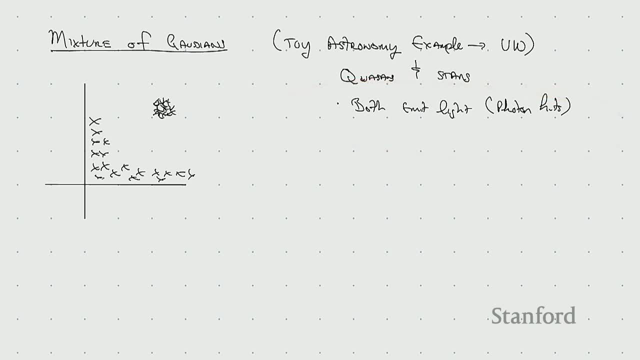 Awesome. So we get these photon hits, okay. So what we want to do is kind of figure out. you know what these different sources look like, And so what we're given this is what we're given. What we're gonna do is try and find a soft assignment. 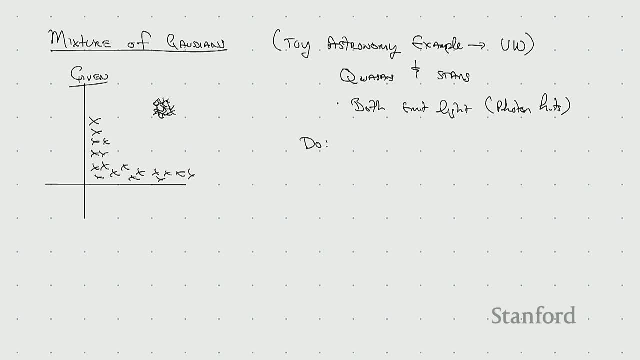 of these things into Gaussians. So remember what Gaussians look like, right. They basically, to high probability, they look like ovals. right. They can be circles, Right. That's what a two-dimensional Gaussian looks like, right. 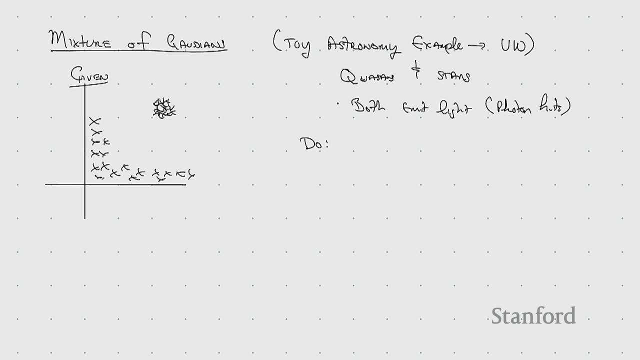 And the variance tells you how stretched it is in each dimension. okay, So like, maybe there's a cluster here, cluster here and this is a tight cluster. okay, Right, so we'll talk about that in more detail in one second. 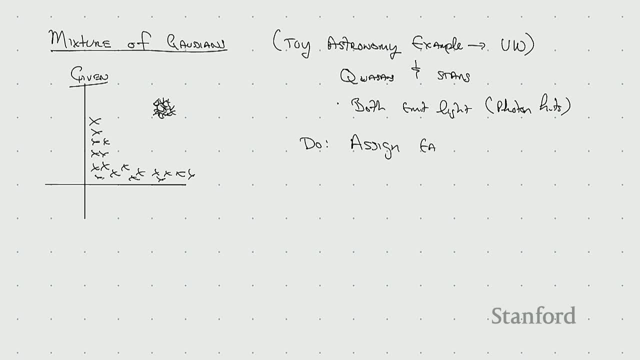 But what we have to do is we want to assign each photon to a light source, But of course we don't actually, in this case, we don't have exactly. we don't have perfect information of the light sources either. 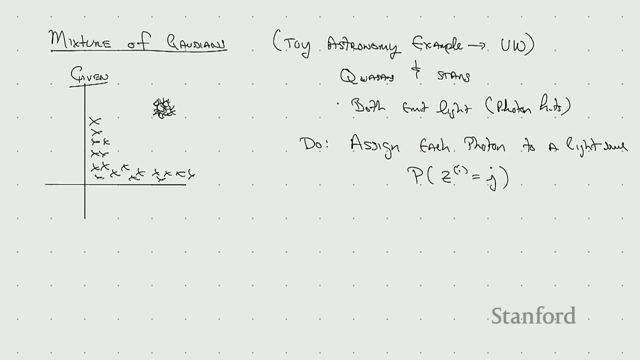 And so we're gonna settle for what we call a soft assignment, okay, So this is the probability. prob that point. i goes to cluster, goes to source j, okay, And this is our soft assignment. This is called a soft assignment, okay. 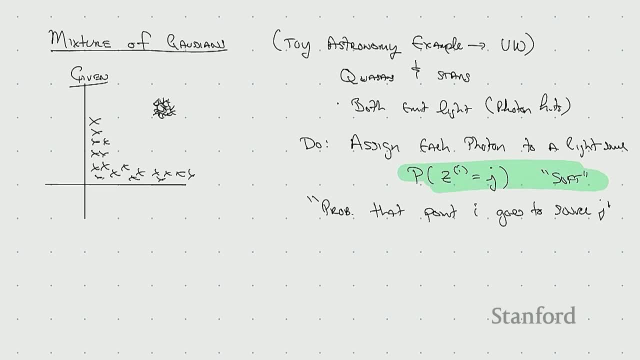 Why is it soft? Because we didn't remember. in k-means we said: you must be in this setting. Here we have some probability distribution over it. okay, Right, so just compare that with k-means. All right, so what are the challenges here? 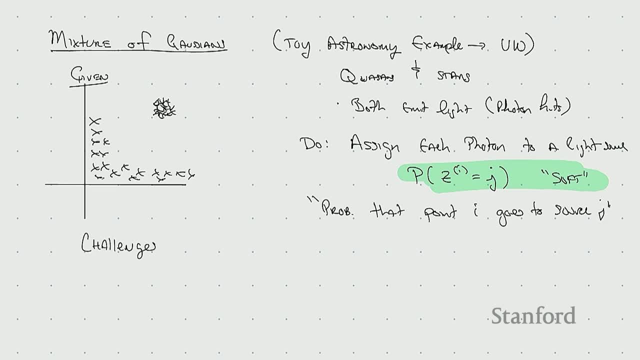 The challenges that we're gonna deal with here potentially are: there are many sources. right, If there were just one source, life would be easy. We would kind of fit the Gaussian. You know how to do that from GDA. You take the mean, you find the variance, you're done okay. 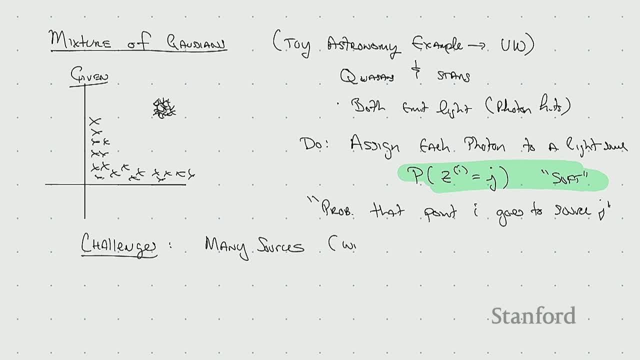 There are many sources here, but for now we're gonna assume we know the source is k. We know k, which is the number of sources. okay, Let's solve the problem in that setting. okay, And also the other problem is: 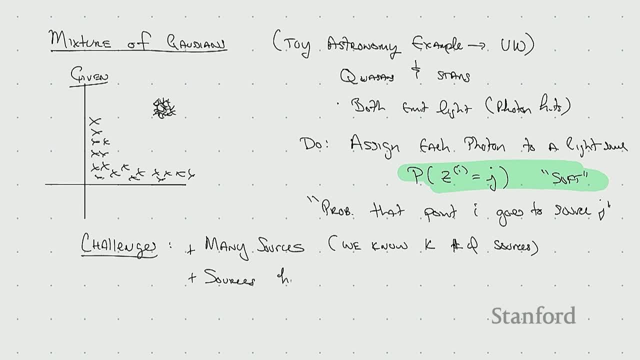 the sources have different intensities and shapes. Intensities and shapes, okay. So when I was wildly drawing those ovals, the reason was: oh, maybe there's a Gaussian that looks like this, maybe there's a tight Gaussian. 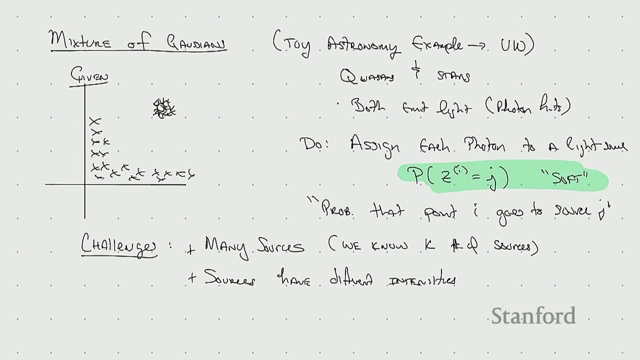 I don't assume I know that ahead of time. I just know that they're somehow well-described by Gaussians. Please, I guess K is still going to be just 4,000 stars over 2,000.. Oh no. 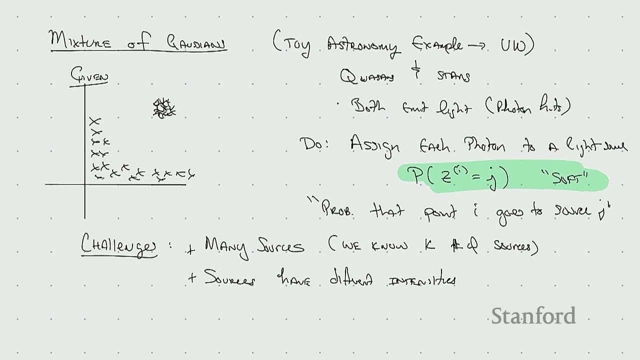 Great question. So those are the two types of things I need. the number of celestial bodies So like one reasonable thing would be three: There's one here, one here and one here. But K is still going to be picked by a modeling assumption. 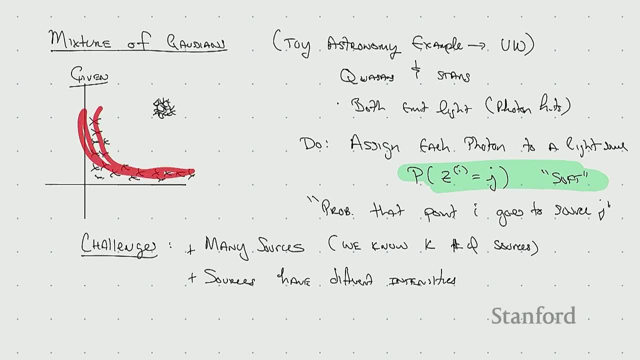 Right, So this curve is hard to generate with a Gaussian in our current setup. Right, So there's probably not. there's probably more than one on that side, But that's just intuition. There could be four there or five there. 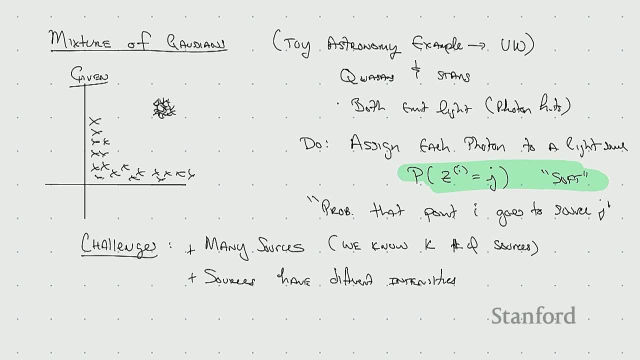 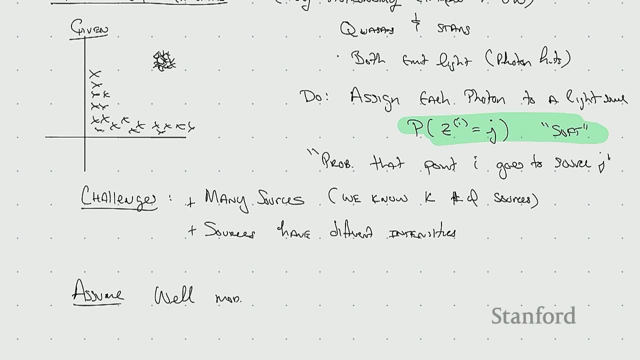 I don't know. Okay, So let me talk about the assumptions. Okay, So we're going to assume it's well-modeled And here we're in. you know, most of what I'm going to do is going to be in one dimension. 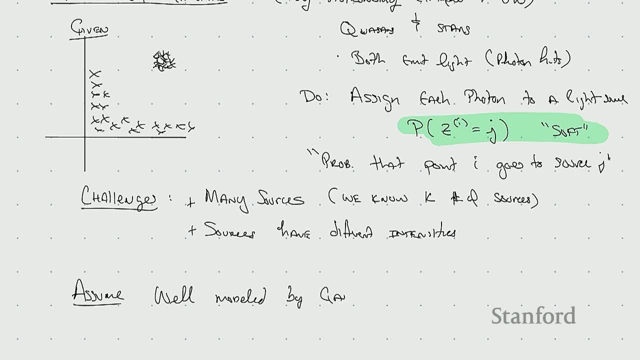 So I'm still just going to introduce the notation in one dimension by Gaussian Right, And you remember that a Gaussian means mu j, sigma j squared. Okay, So we're just one dimension to make our lives similar in a second. But we do not assume 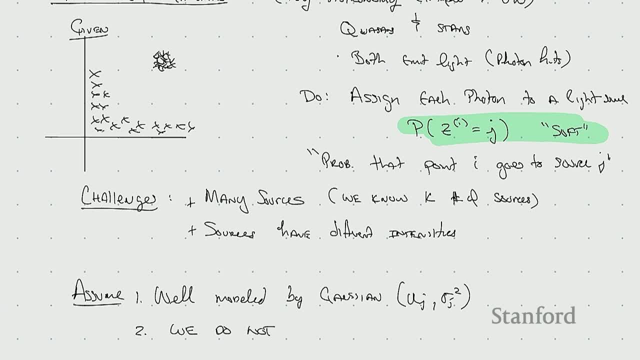 that we know how many points, that there's an equal number of points. Number of points is equal. Okay, Now the reason is in our setup. the physical reason is, like you know, some point sources are really concentrated. 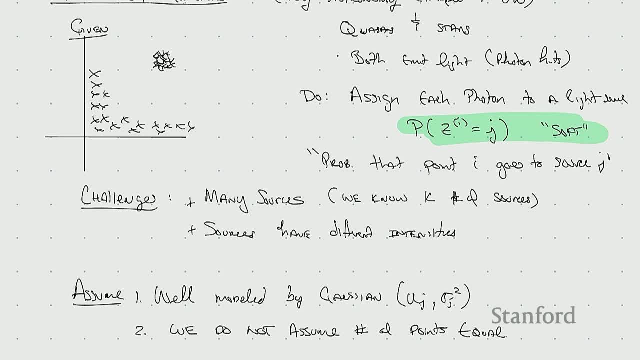 and strong and they shoot out tons of photons. And in other cases they'll shoot out. you know, diffuse photons over a region. They may be farther, closer away, different energy levels, whatever, Mathematically. what I mean is: 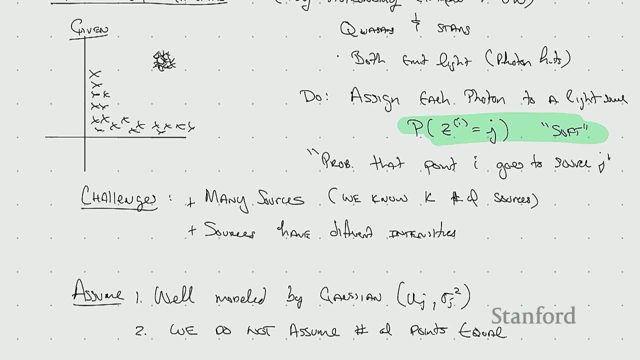 we don't know when we're going to talk about these Gaussians. The shape may be a Gaussian, but it's only. it's only sampled infrequently for source one and it's sampled 90% of the time for source two. 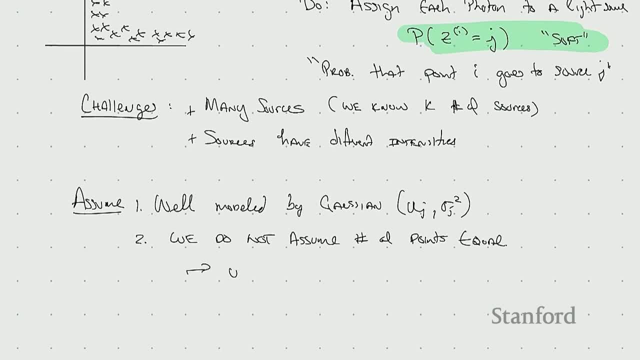 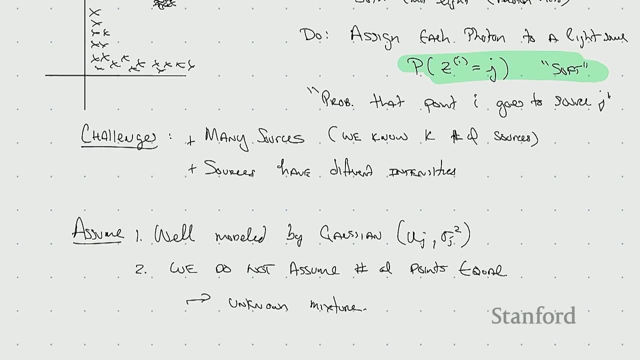 Okay, This is formally known as an unknown mixture. Okay, Now, one thing that's nice about this problem in the physics setting is once I get the values out. so what are the what's the do here I have to get out. 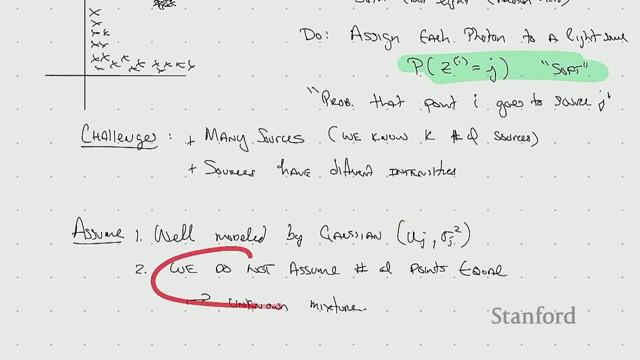 these cluster centers that we talked about before and these probabilities- which I haven't given you notation for but they're going to be called phi in a second I can check that- of how physically plausible that clustering is Right. So in the K. 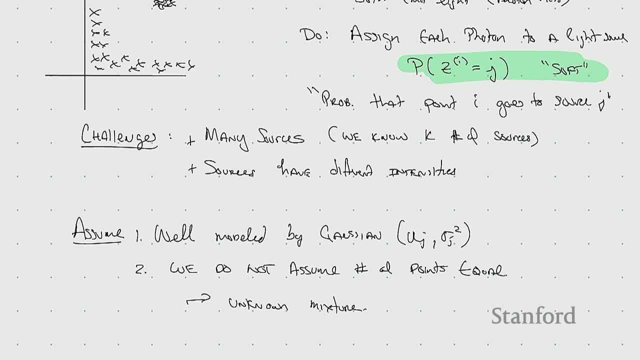 the reason I like this example is in: the K means you kind of have to eyeball it, but here, if I have a physics model, I can compute how likely is one clustering versus another, given the data sources that I'm seeing. 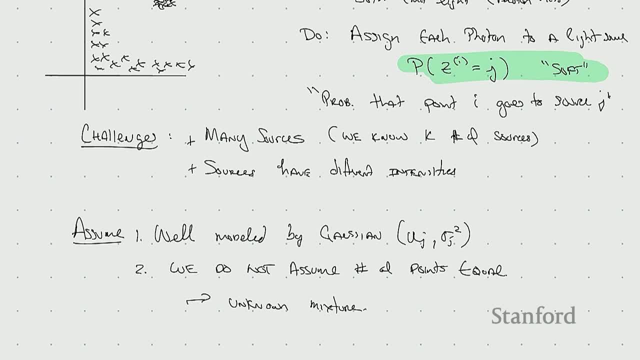 Maybe you have auxiliary information about what celestial objects are in the sky in that particular region, and so I can. I can check this information, Okay, And the physicist in this example could actually check the information. Okay, Please, What's the range of G? 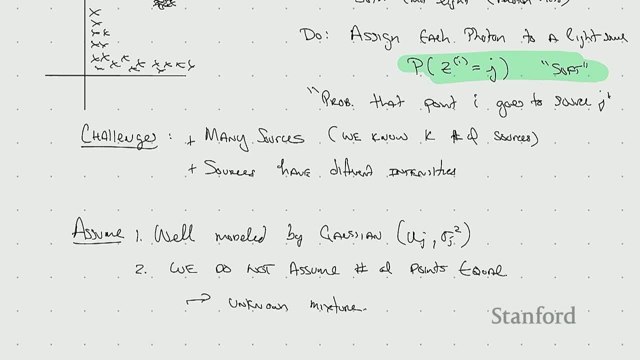 The range of what J, Oh J is going to range. the same is going to range over each number of sources. So we're going to assume that we have this K number of sources here, So J will range over K, just like it did in. K means 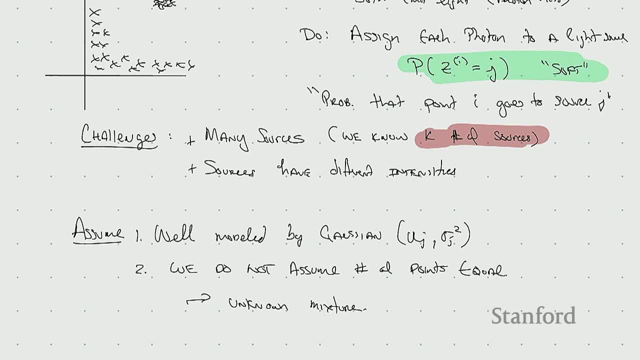 So that's fixed. That's a parameter of the problem. Someone's going to tell me. basically what someone's going to tell me is: there are K sources. I don't tell you what their means are. I don't tell you what their variances are. 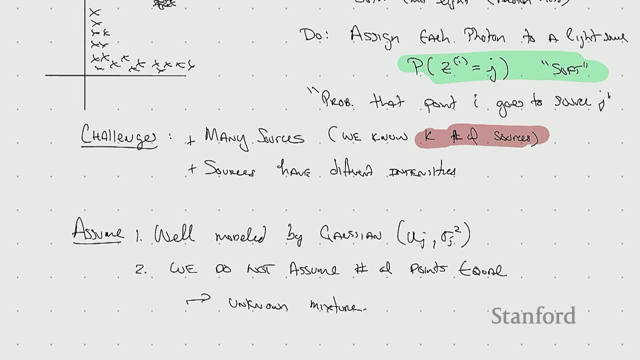 So that's for each one of them, And I don't tell you how often That's this mixture. They emit light. So what percentage Of the points go to source A versus source B, Please? So, for example, let's imagine that we had 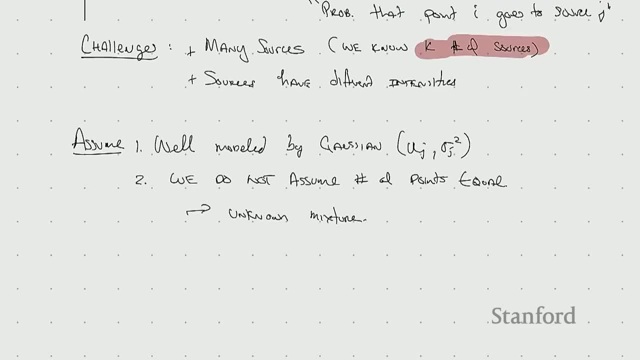 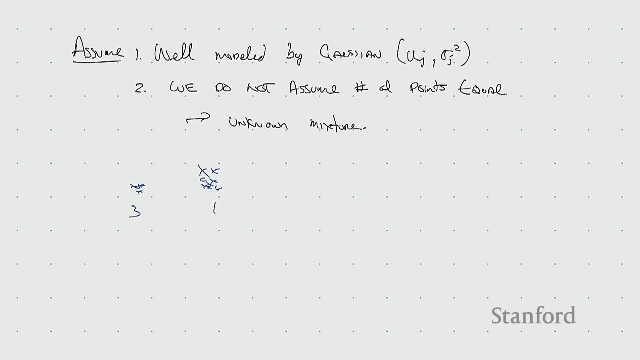 a situation like: let me just draw it. So let's say that we had, you know, three points here, and then I'm not going to draw them all, but like a thousand points here. So there are three points here and a thousand. 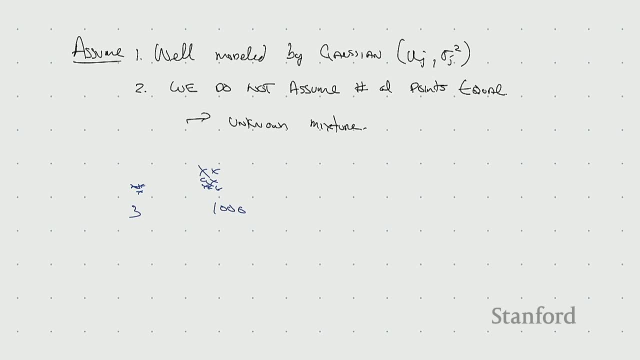 and a thousand points here, Right? So the clustering that I would want out is one cluster here and one cluster here, But I don't get to see the three and one thousand. I'm assuming that they're of unequal sizes, So you could, for example, 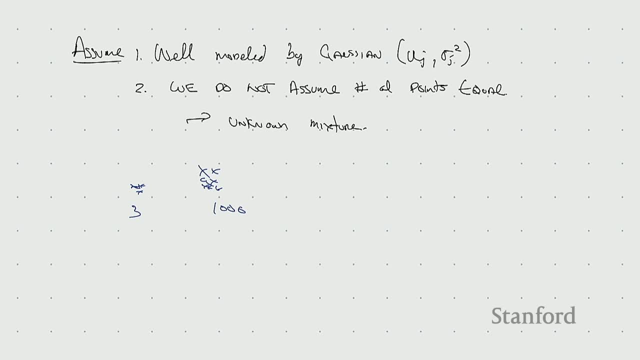 assume that all the clusters are equal sizes. I'm trying to, and that would be wrong and that's not the way we'd have the model. That's a fair assumption if you knew that right, But that would make your life a lot easier. 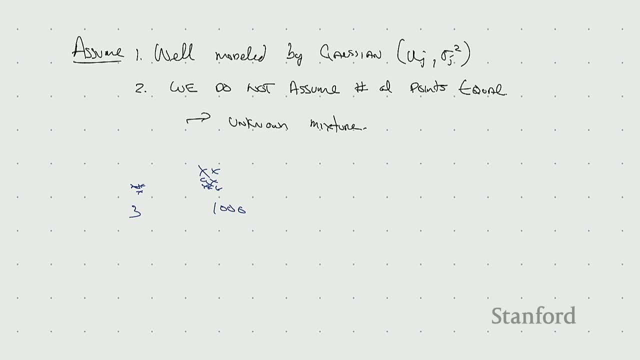 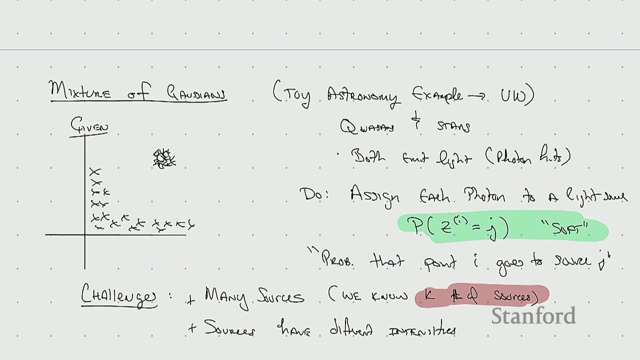 It doesn't make you have to solve both of these two things. Okay, Awesome question, All right, please. Yeah, we make that assumption kind of implicitly, because we don't say how often, like there's no probabilistic model, but we do allow K. 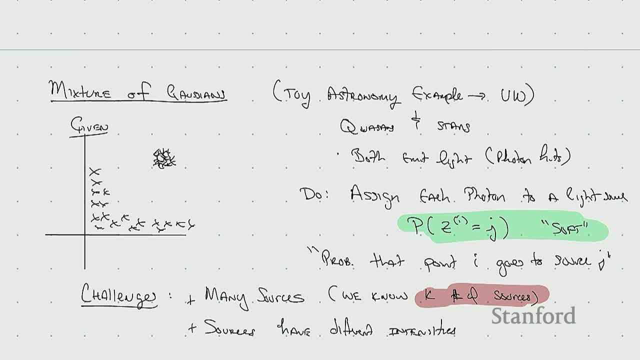 to have like five neighbors and 500 neighbors. right Center cluster. one could have five neighbors, another one could have 500. So it does parallel K-means. so in that sense it's the same assumption I'm calling it out here. 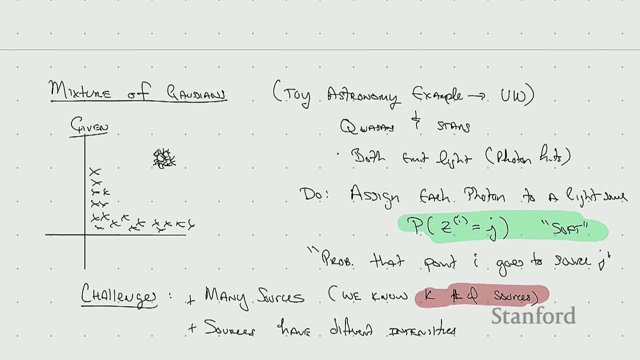 as an extra parameter that we didn't have to think about last time. Right, Awesome questions. Okay, let's see some 1D mixture of Gaussians. Mixture of Gaussians is like a very fun and famous problem, by the way. 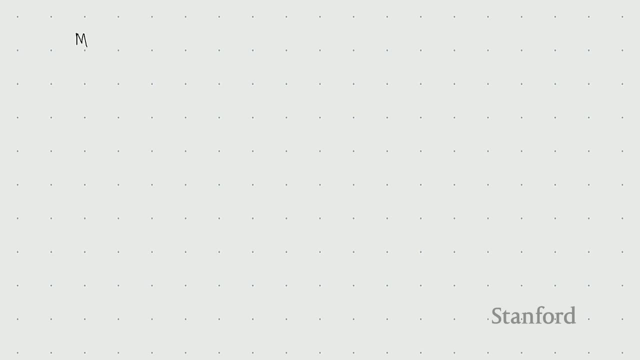 People like work on like which ones you can solve In theory. still, it's like a fun. it's actually a fun and interesting problem. We won't do that, All right, So I'm going to be in 1D for simplicity here. 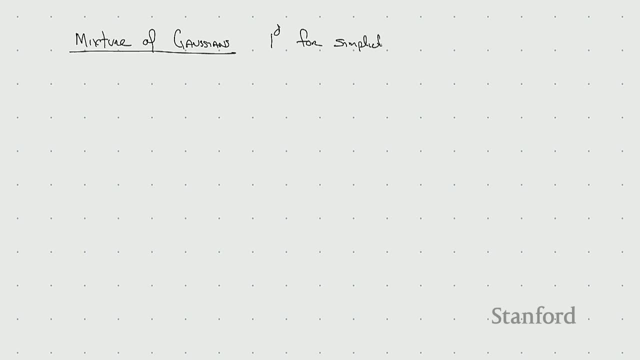 because it just makes my notation and drawing easier, because I have to draw distributions right. So just make sure it's super clear what we're doing. I think folks sound like they have it. So we have 1D. This is going to be. 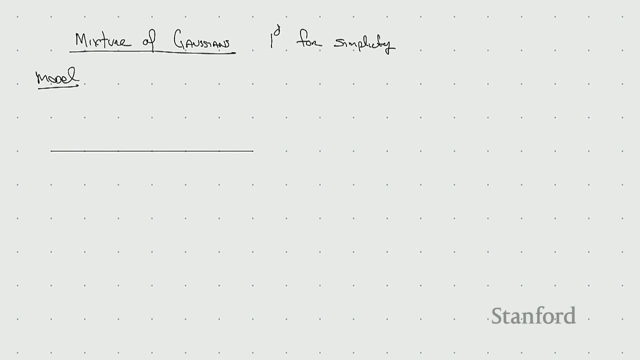 the place where our points live. And then imagine there were two Gaussians that were generating data. Okay, Now, when I say this is generating data, this is the piece like when I talked about. we were going to talk. we're going to allow ourselves. 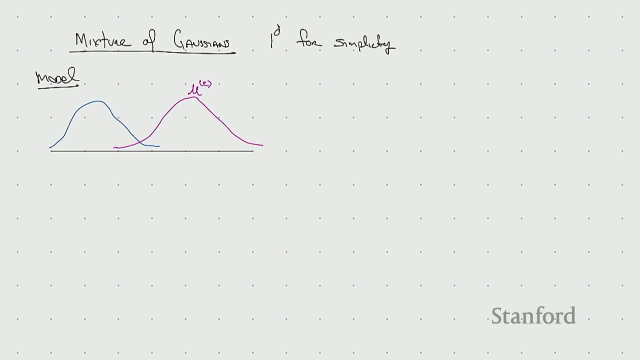 to talk about models. we're going to imagine that there's really a model that's underneath our data that's generating it. Okay, This is quite a powerful technique. Okay, So how does it work? What we're going to do? our idea for the model is: 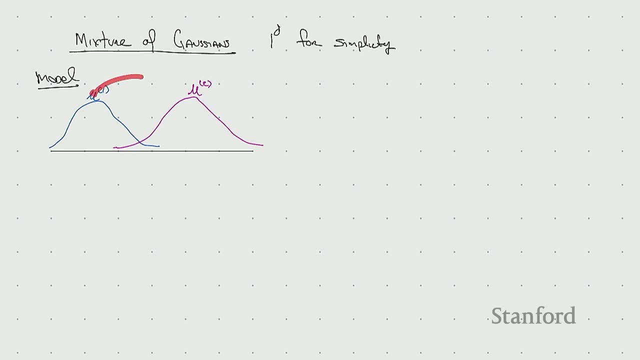 we're going to pick, you know, cluster one with some probability- let's call it P- or cluster two, with probability one minus P, We pick cluster one. we then sample a point. Oops, let me get a thicker thing, All right? 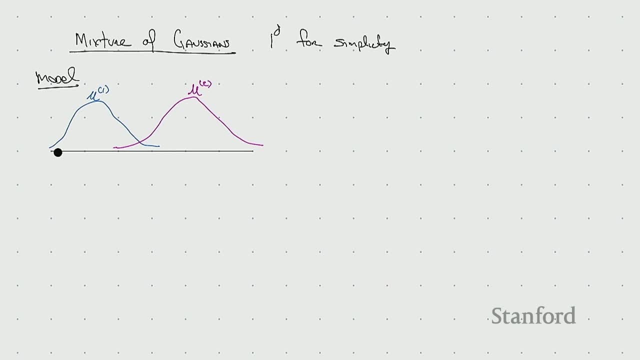 Oops, that's probably too thick And we get a series of points. Okay, That's the thought process that we're going through. right, If we only knew those parameters, we could sample from our model, If we knew the probability to pick cluster one. 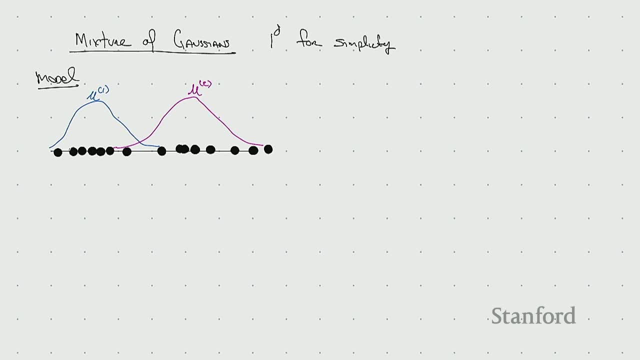 versus cluster two, and then we would sample from it, And there's many different parameters given that model that could have generated our data and we're interested in recovering the ones that are most likely that most likely generated our data. Okay, Now what we see. 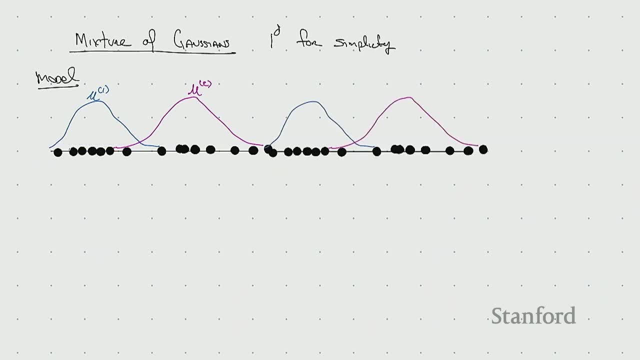 unfortunately, is just this, Just the points, Okay. So this is the model over here. This is what we observe. Oops got to switch back. Just the points in R. Okay, These are the XIs. Now one thing. 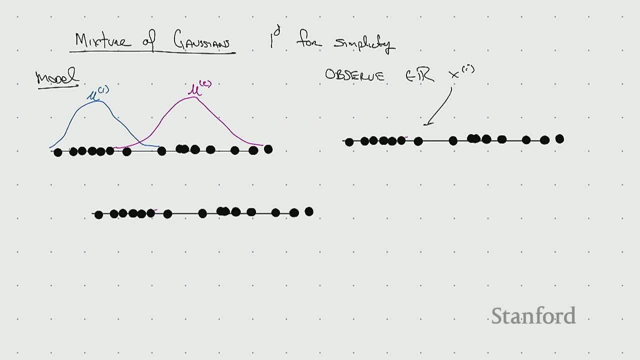 and this is going to seem like a trivial piece, but it actually makes our life kind of interesting. What if we knew these points all came from cluster one and these points came from cluster two? Okay, this is our first observation. Well, if we knew the cluster labels? 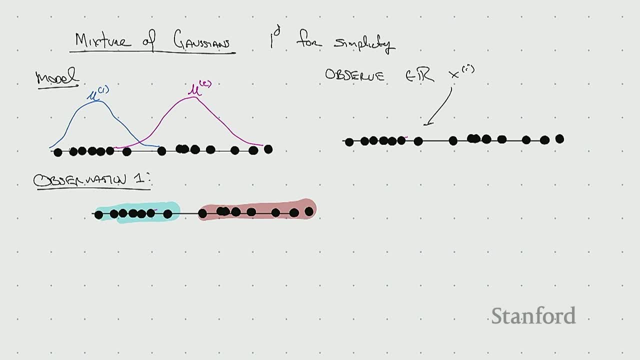 what algorithm would we run? We just run something like GDA. we would just fit Gaussians to this. We'd be done right. So if we knew this, we could just solve this instantly. Solve and fit Gaussians. Solve and fit Gaussians. 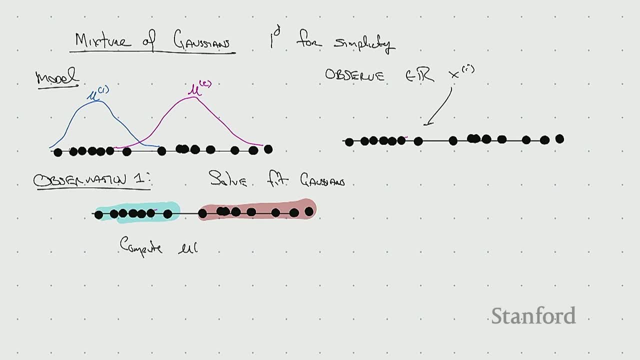 So we compute mui, mu1,, mu2.. How do we do that? Well, we would just average up all the things in here. Average up all the things in here, That would be our mus, And we could even compute the sigmas. 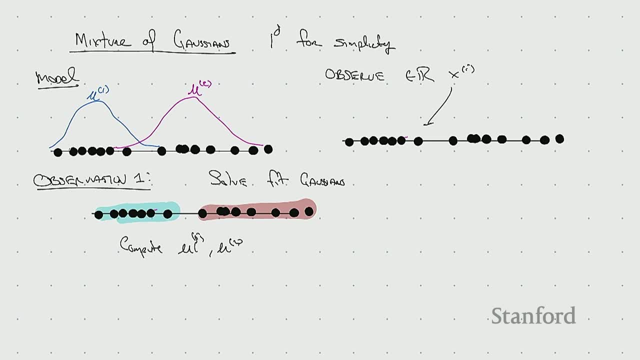 and be done. The challenge is: we don't get to see them. We don't get those labels. Challenge: We only see this thing. Okay, This is our first example of a latent model. There's something hidden that we don't observe. 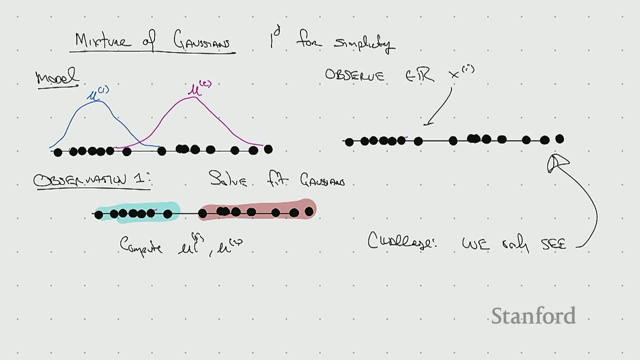 and we're trying to estimate the parameters of that latent model And that will be a theme for the next couple lectures. Please, In the previous, when you look at the data, you said you only more than two values Because of the 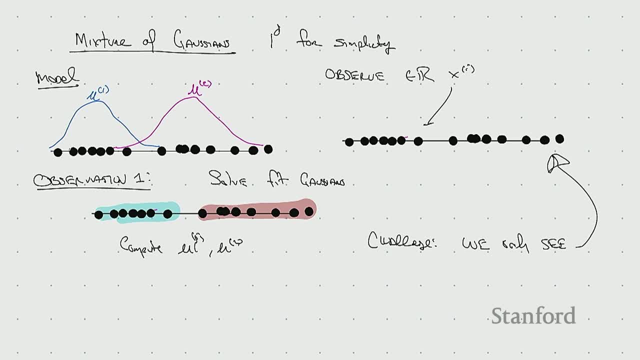 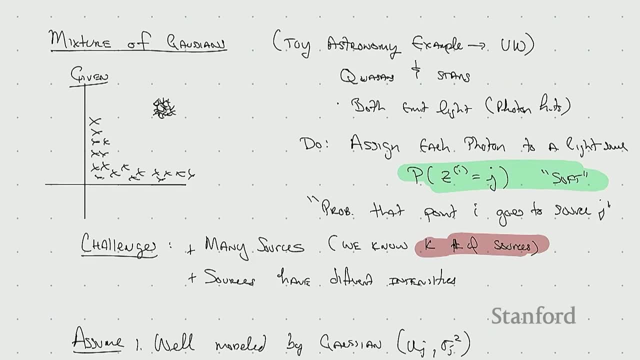 Sure, yeah. So should the data be more than the two, Or is this? No? oh so this is yeah. so this was an example to motivate, like, hey, this is like a nice picture to look at and kind of get you thinking. 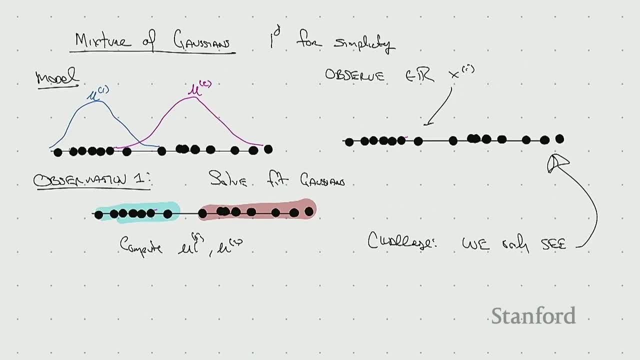 empirically about what happens. I'm going to walk through most of these things in 1D because it makes my notation a lot easier, And so there's really no relationship between like these points and the points I showed you before. Yeah, great question. 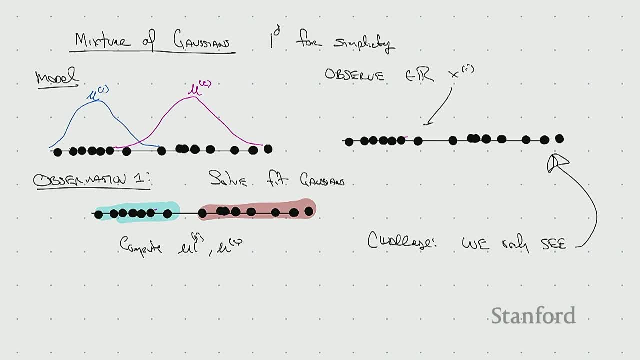 Awesome, All right. So why am I doing it in this kind of like piecemeal way? It's because when I show you the definition, then you know it has a bunch of notation in it And I want to show you. 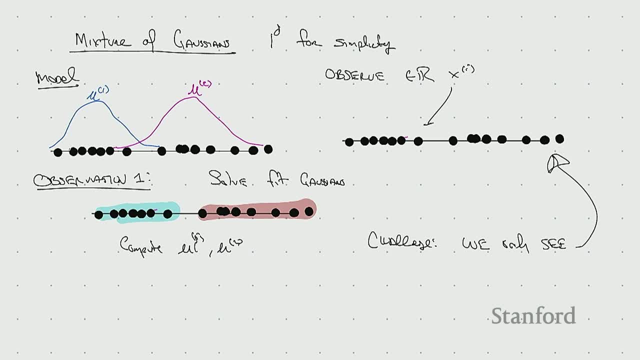 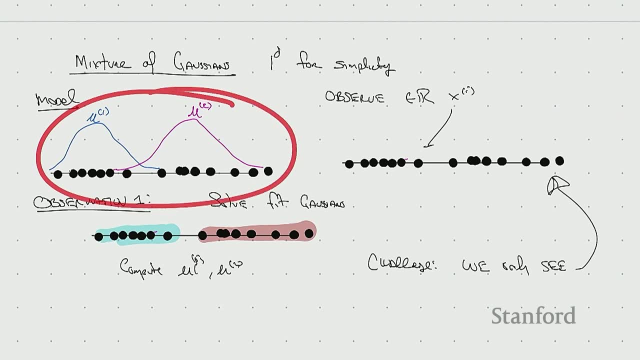 the simplest version, so that then you can generalize it and and do all that fun stuff on your own. Okay, All right, But is it clear what the what goes on here? There's this notion I've introduced and kind of sneaked into you. 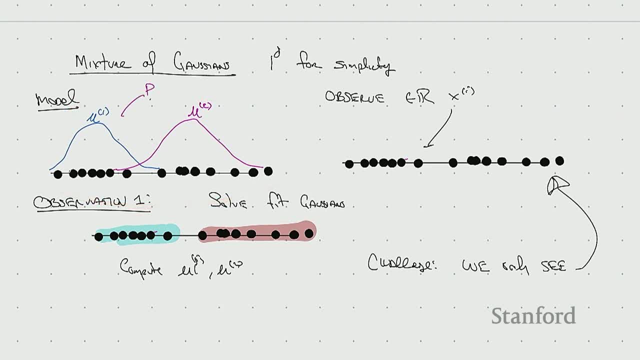 which is a model right. There's some parameter P here that picks this side or this side right. It's going to be called theta, theta one and theta two. hinting later, I pick something and then I sample from it. 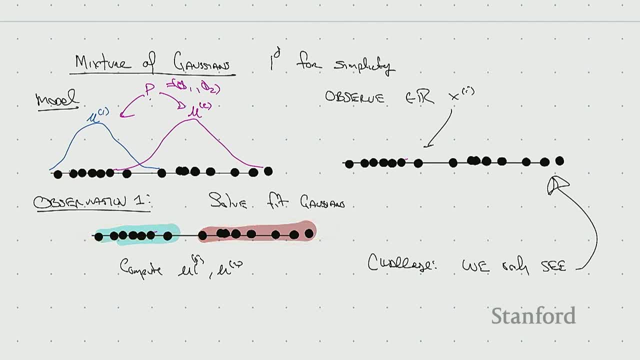 If I knew where the points came from, I could just solve it, But the problem is I have this hidden. how often is everything sampled? I don't know how many points should be in each cluster And I don't know which points are in the cluster. 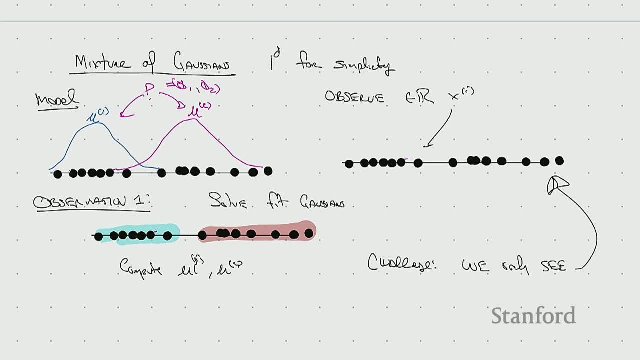 Not only do I not, you know, I don't know either of those facts, So we have to estimate them somehow from data. That's what we're going to do. Okay, So let's see some notation. We can come back to this example. 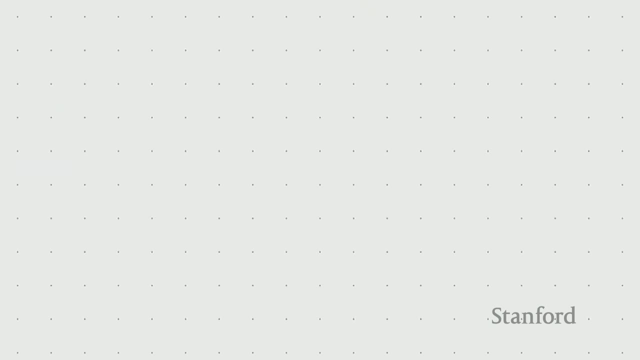 if, if there are more questions about it, Okay. So let me be a little bit more precise. So we're given X one, X N, element of R, Okay, And a positive integer, K And K, you know, positive integer. 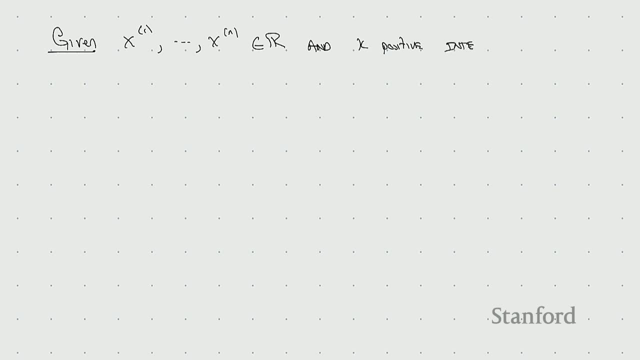 Our number of sources And our do what we're given. what we have to do is we need to find that probability function, Find P such that for I equals one to N, J equals one to K, the clusters. This is the data. 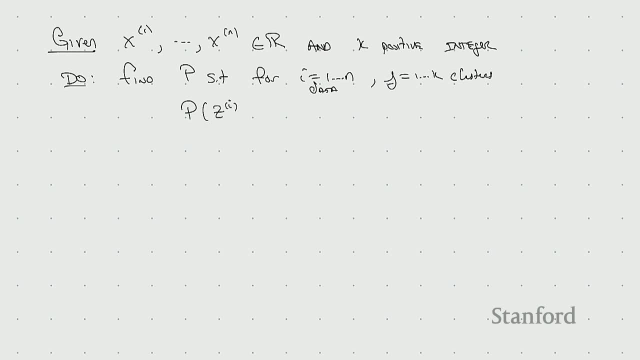 We have an estimate of P0, ZI equals J. This is our notion of soft assignment. Okay, So that's what we're responsible. Okay, And this is, although it's a function, it's discrete, so I can write it down. 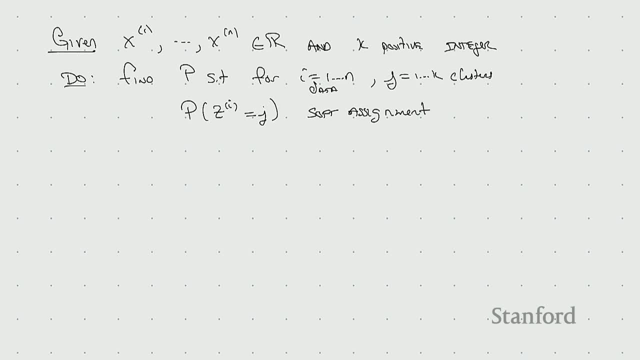 Right, I can just write down the probabilities in a table. We'll later worry about cases. that's not the case, but for now we do Make sense. No, So J is a cluster index and K is the number of clusters. So 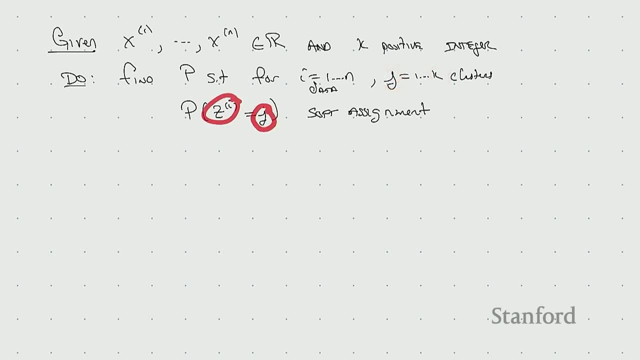 J here says this: says: the ith point belongs to cluster J. with some probability J ranges over one to K. So they are K clusters. No K was equal. we never actually were precise about what K is. We had rough intuition that K should be at least three. 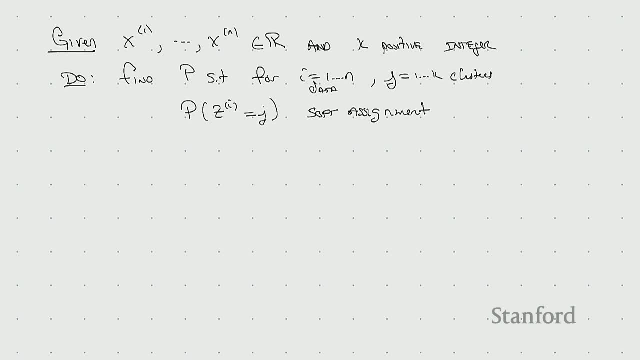 and I don't think we actually used J or if I did, I meant and scribbled it incorrectly and I apologize. Probably was a wayward. I I don't see it in my notes, but apologies for that. Sorry for the confusion. 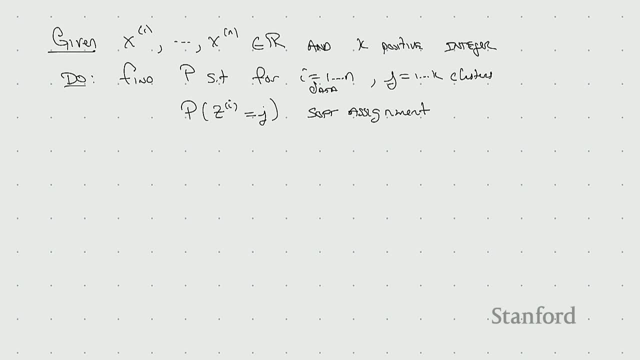 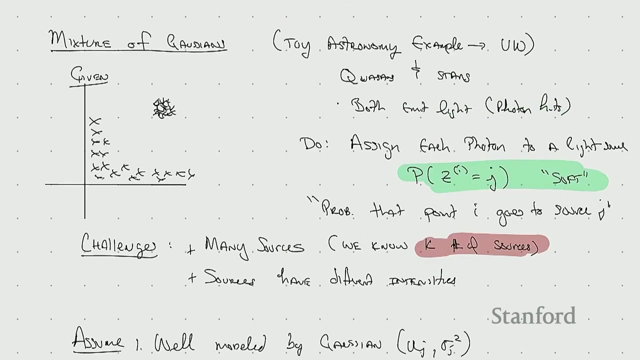 Please. Z of I means that the sample I belongs to, cluster Z Belongs or comes from Yeah, so I'll copy from here. It's this sentence: Probability, that point I belongs to. I think it should be. I think is what I meant to write. 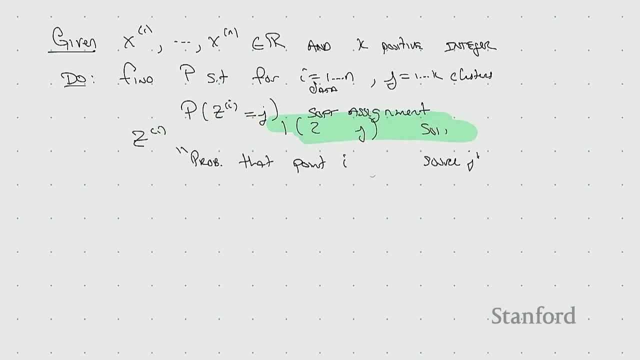 I think that's better. Probably that point. I comes from source. That makes more sense in English: From source J. yeah, Yeah, source J is the particular source, Always the particular source. So I is always the data. J is always the label for the cluster. 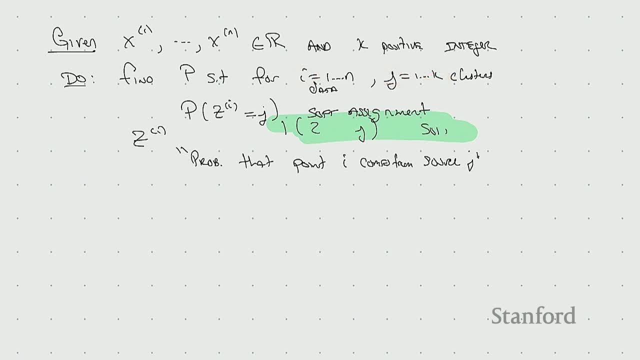 and K is always the number of clusters, Please. So is that an X or a Z? Is that an X? That an X? Oh, you mean from the. Is that an X? on what script? No, So yeah, so ZI is the assignment. 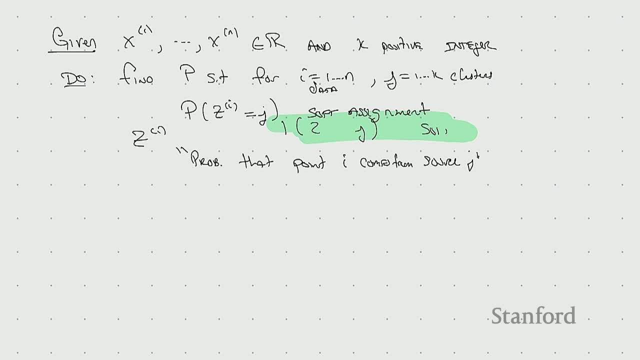 So ZI is the soft assignment itself, XI is the data point. Yeah, sorry for the overloading the notation, So the ZI's will always be the hidden piece that says the. so let me write the next sentence, the next piece. 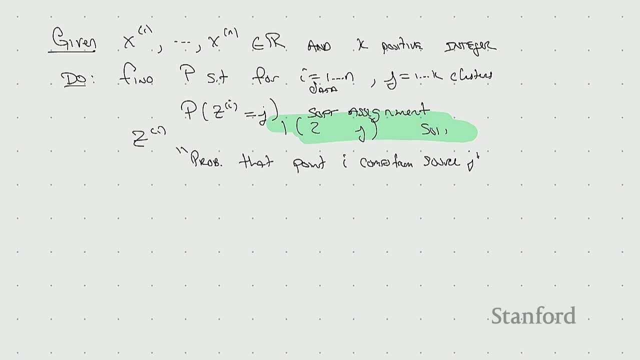 and then we'll come right back to your question. I can see why you'd be confused by that, So let me write the GMM model and you'll see why these two things are being used according to the GMM model. So ZI is just the. 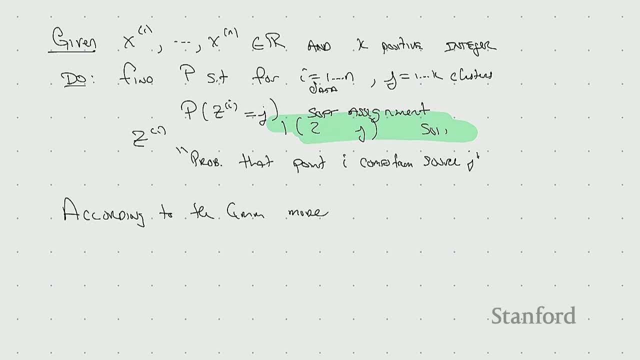 ZI is the random variable that this probability, that point belongs to it. It's not the actual point itself. It's not the actual point itself. So then, for example, we can talk about the probability of XI and ZI. This is the probability that, given this point, 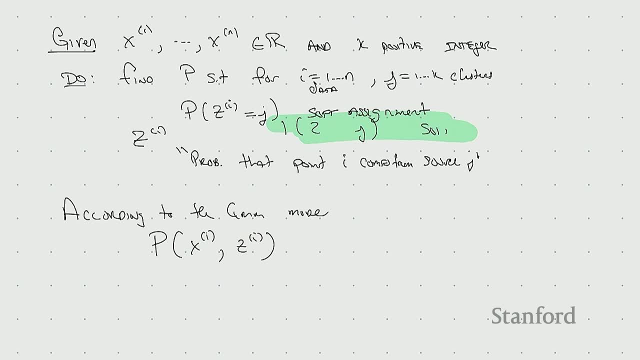 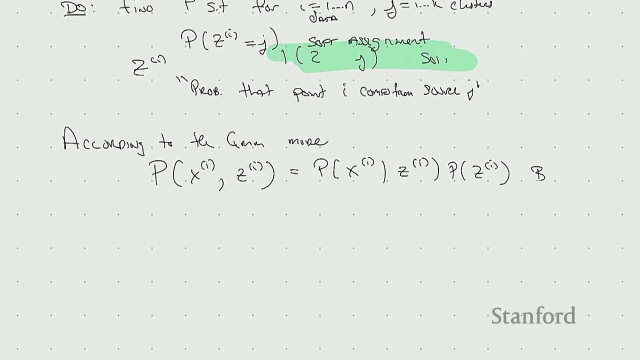 and the ZI is that it belongs to a particular cluster, And we'll write down the model in one second. So let me write down the model and then it'll be clear what this notation means. Okay, All right, This is just Bayes' rule. 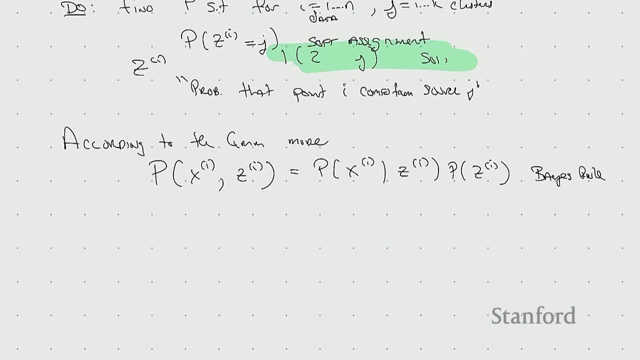 Nothing fancy here. I said nothing. There's no content. Okay, But I'll use it Now. ZI is going to be distributed as a multinomial according to some parameter that we'll call phi, And phi as a multinomial says that some phi j. 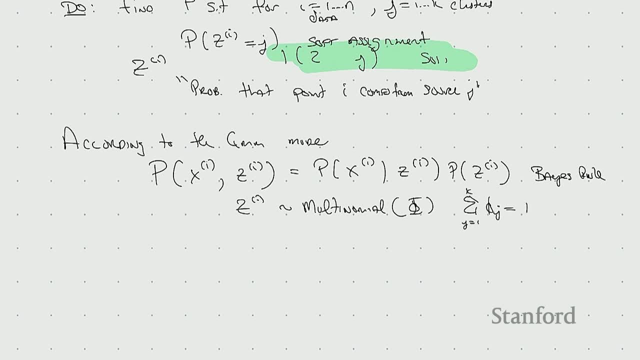 j goes from 1 to k equals 1, and phi j is greater than or equal to 0.. Okay, So ZJ, if you like, is that sampling probability, Like it's the likelihood that this particular point came from that point? 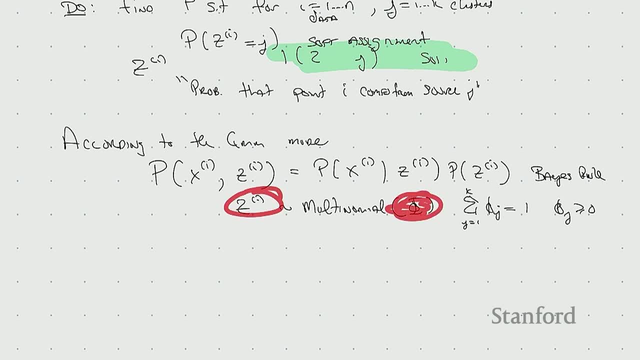 It's the likelihood that it came from that place And ZI is going to be picked with this background probability that we were calling p before. So in our earlier example there was like p and 1 minus p were the chance that I sampled from cluster 1. 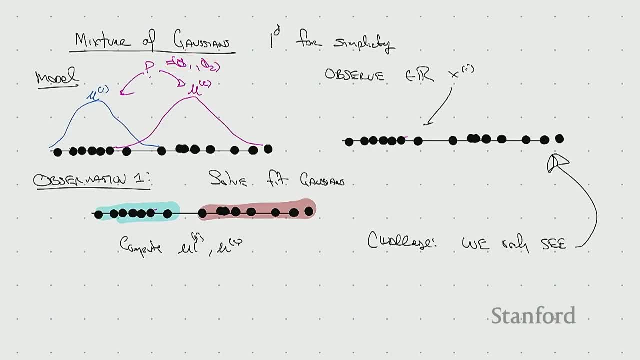 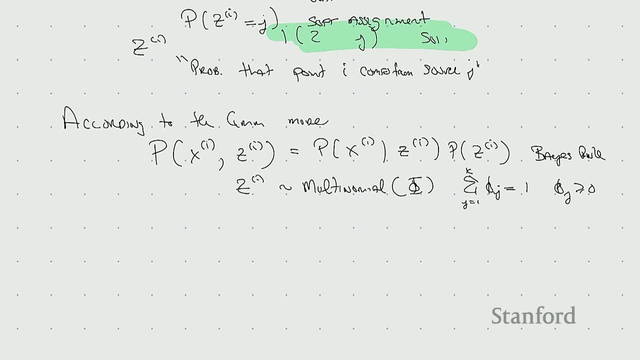 or cluster 2 above here. Okay, These were phi 1 and phi 2.. That's what I was hinting at. Okay, And remember, in our model, like I picked ZI, That told me where I was sampling. 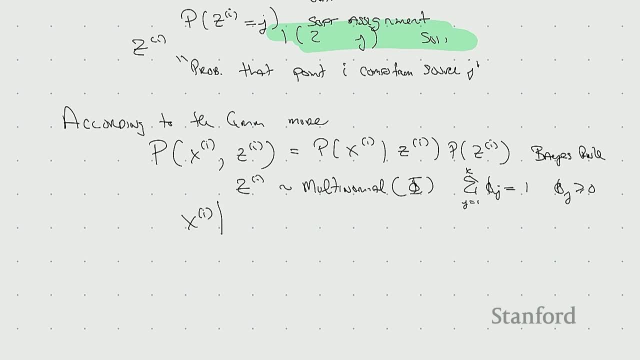 And then, once I knew ZI xi- given that ZI equals j, that means, given that it was in cluster j- this is going to be distributed like a Gaussian: Mu j sigma j square. Okay, So these are all Gaussians. 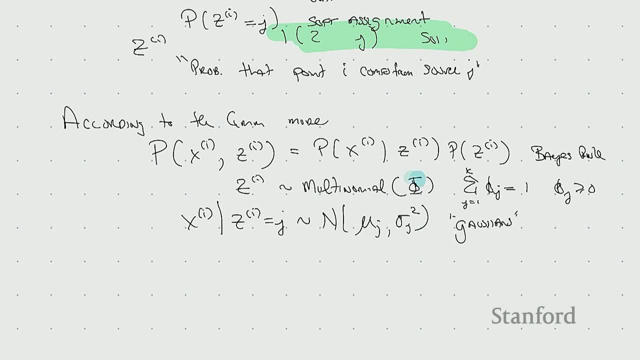 Okay, Now let me highlight for you the parameters we have to estimate. Highlighted parameters: Okay, This thing, Or this thing? Okay, All right, These are the same color. So what's going on here? This is formalizing the model that we talked about earlier. 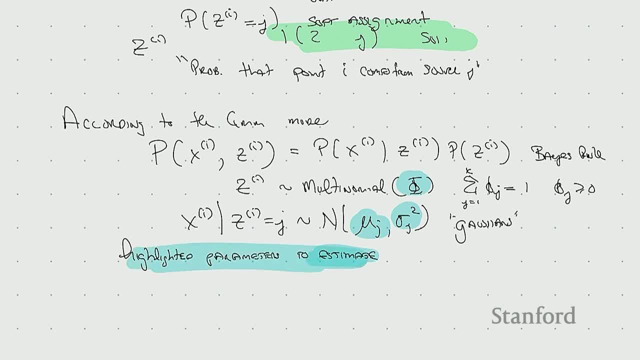 It's our first kind of hidden model. We never see ZI, We don't observe it in data, We don't get to see the labels. You know the deity or whoever is generating this data, generates a ZI and picks it up from cluster 1 to cluster 2.. 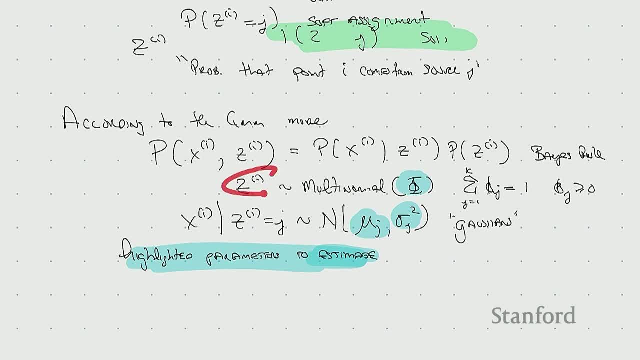 And then it's like: okay, I'm going to pick this one, I'm going to pick this one, I'm going to pick this one. And then it picks one of the clusters. That's its sample for this point. 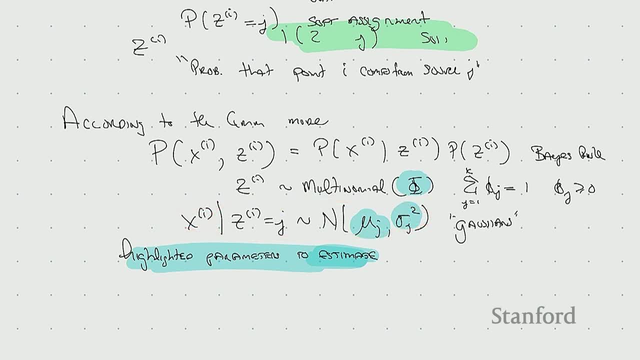 And then it samples from this normal distribution to generate XI And, if you like, the data we think about as being the remnants of this process. We don't get to see this process run. It gets run ahead of time And then the data is dropped there. 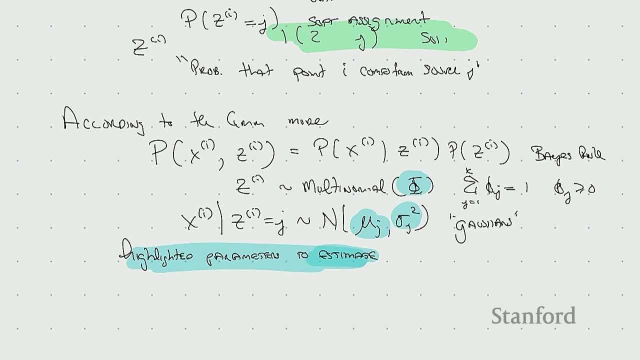 And the reason we're thinking about this model is we say, okay, assuming that the model were like this, could we recover the parameters? Okay. And so that's the sense in which we're assuming there's some structure And it's pretty reasonable. 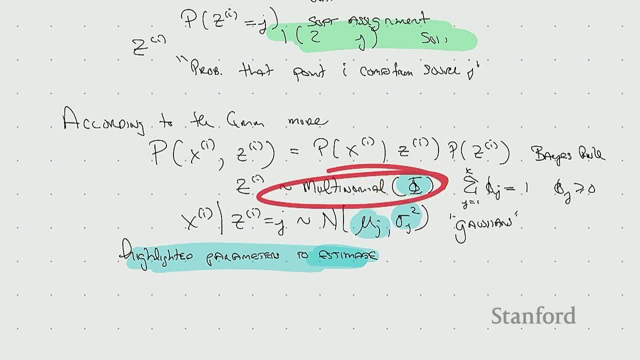 What it's saying is: look, I don't know how many points come from every cluster. That's because I have a multinomial And two. I know that the clusters that I have they're Gaussian shaped, But I don't know if they're circles or ovals. 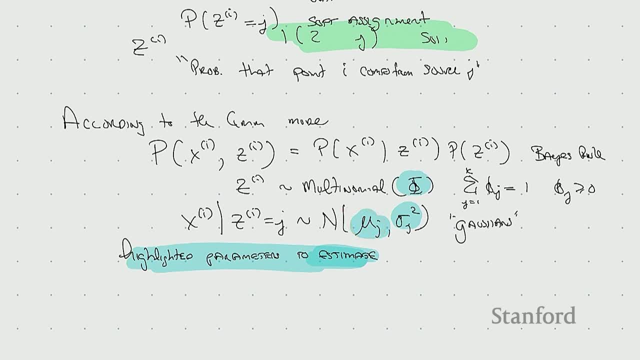 And I don't know where their centers are, And I'm assuming nothing else about my structure. Can you find it for me? That's your job. Does that make sense? You have to come up with, we have to come up with these parameters. 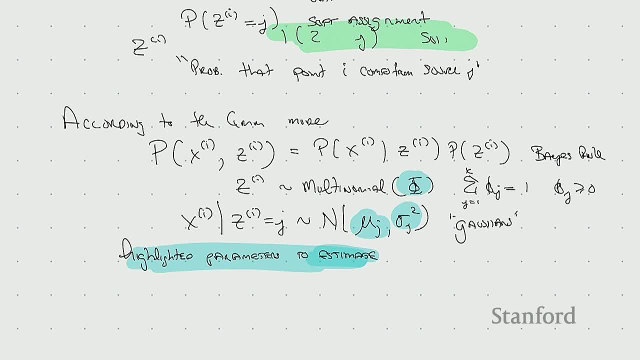 We have to find the cluster centers and the probabilities that each are sampled from observing the data. Clearly, if I pick one clustering, the data's going to be very unlikely to have been generated with those centers. If I go back here and I pick the center over here, 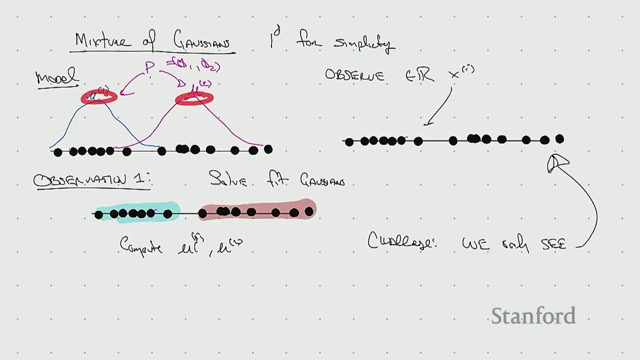 and the center over here. that's less likely than if I put the center here and the center here. It would just explain the data less well. We'll be able to formalize that with maximum likelihood, But I hope that intuition is clear. 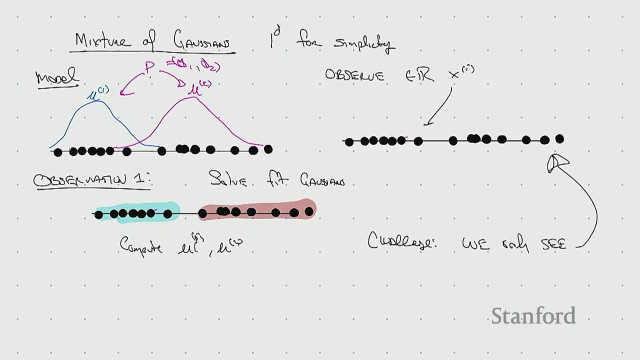 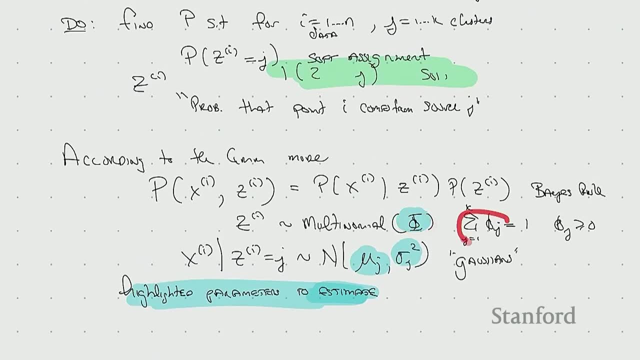 If it's not, please go ahead ask me a question. I'm super happy to answer. Can you explain the variable phi without intuition? Ah, So phi It's basically just a bunch of numbers that sum to 1. It's a multinomial. 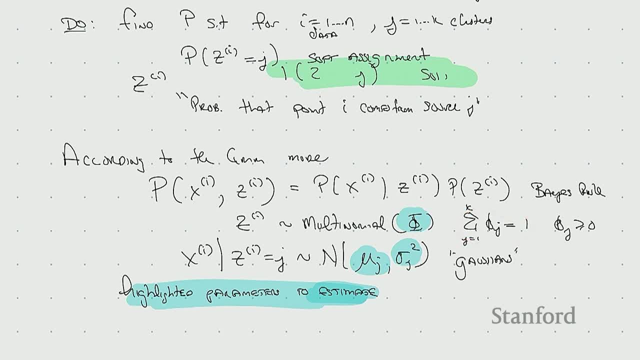 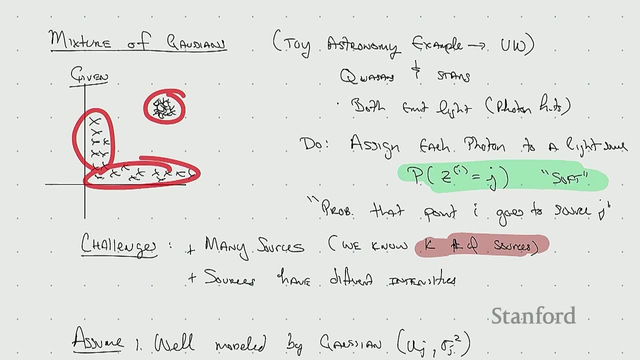 So this is a probability If I have cluster 1, so let's say this is going back here. Let's say this is cluster 1,, cluster 2,, cluster 3, or source 1,, 2, and 3.. 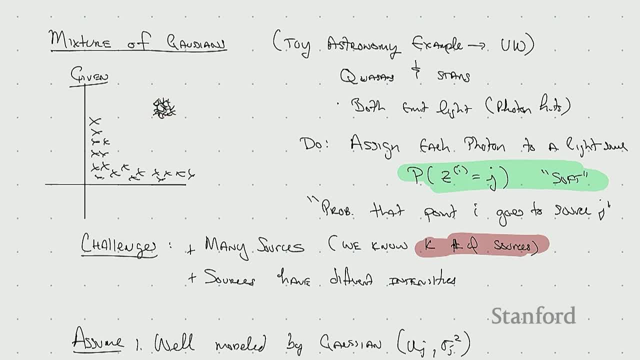 And lots of points are in source 1.. So then maybe phi 1 would be like 0.7, because 70% of the data is there And 10% of the data is here and 20% of the data is here. 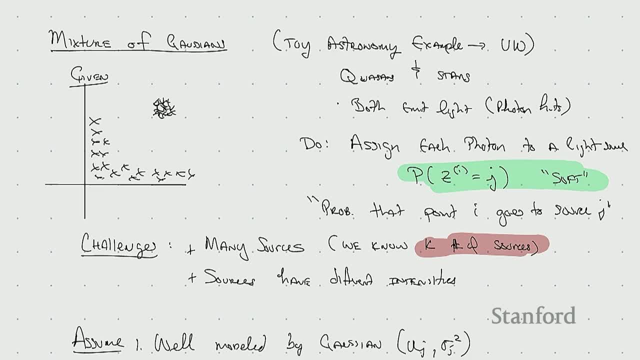 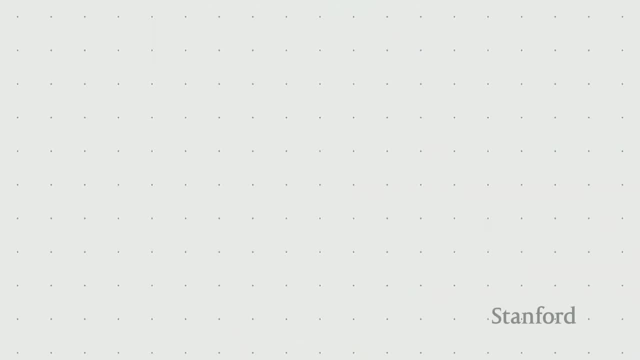 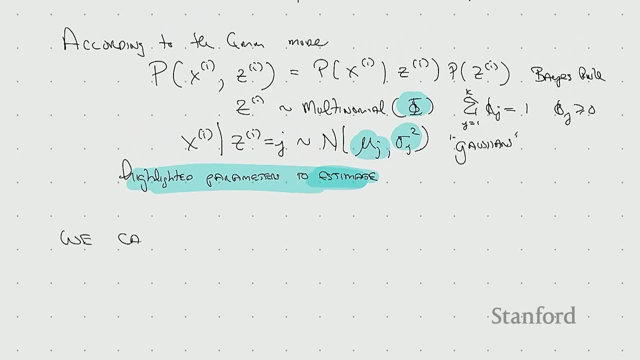 Then the numbers would be 0.7,, 0.1,, 0.2, roughly. Does that make sense? Awesome, All right, All right, All right. so let me, let's do one example. I just want to, I'm trying, let me see. 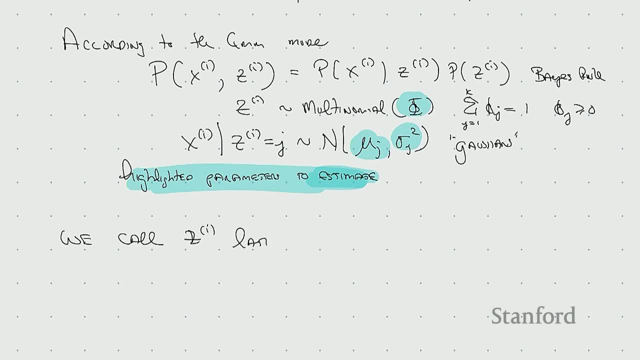 call the zi latent because we don't observe it. We didn't get to see it right, We just got to see the points. We didn't get to see which was assigned to which cluster, because it's not directly observable, This concept which seems at this point kind of strange. 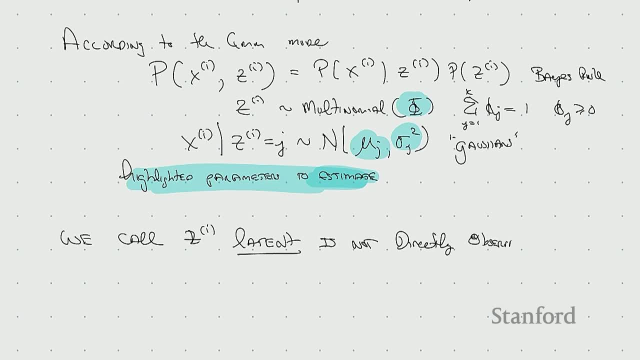 I would think about. So let's take a bunch and we'll see it again and again. This is what we mean by structure. We're like: well, there's some wild collection of points, but there exists a small number of clusters. 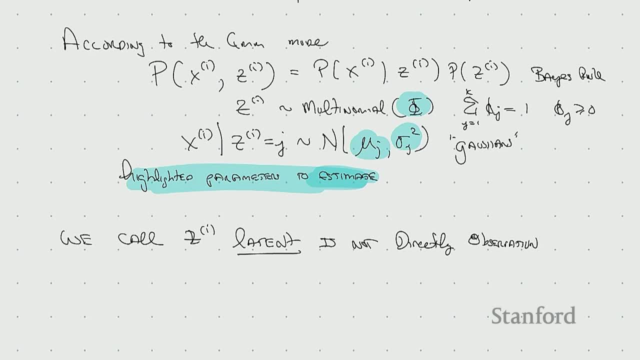 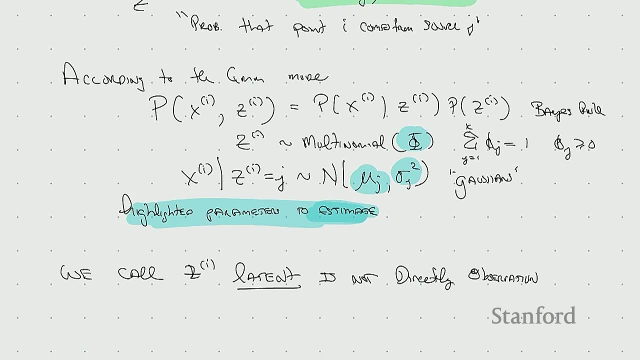 that are generating them. That's the mathematical embodiment of what this thing is, the mathematical embodiment of that intuition. That's all it is. And we say, if that's the case, then we should be able to recover it. okay, We should be able to recover those clusters. 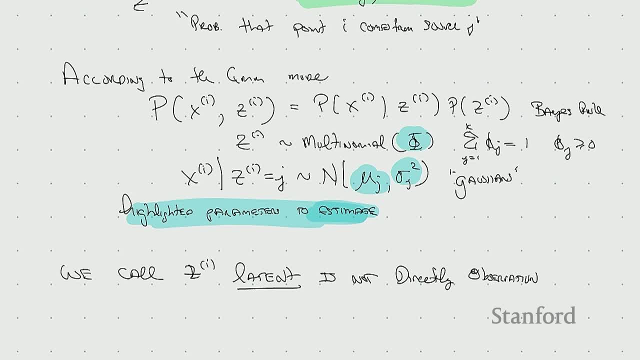 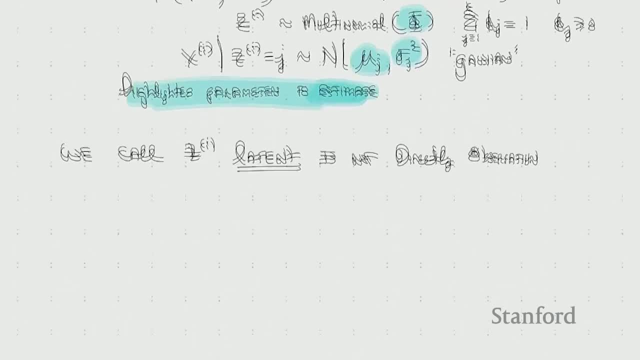 in those situations And in the physical situation of light sources. that seems pretty plausible, right? Like you know, they have different intensities, different types, so on, all right. So let me give you one more example, just to make sure. 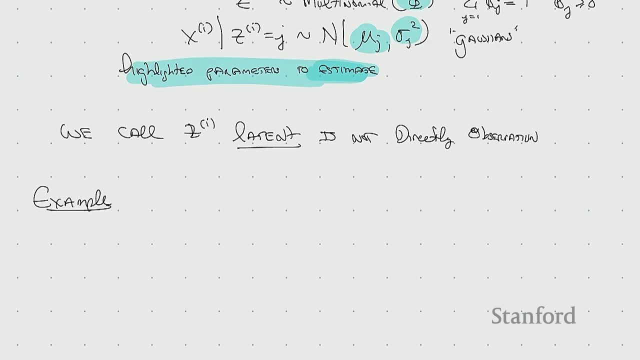 that all these terms are. this notation is there And I want you to think in sampling And let me just walk through, so hopefully these things make sense. So phi one is going to be 0.7, phi two is going to be 0.3.. 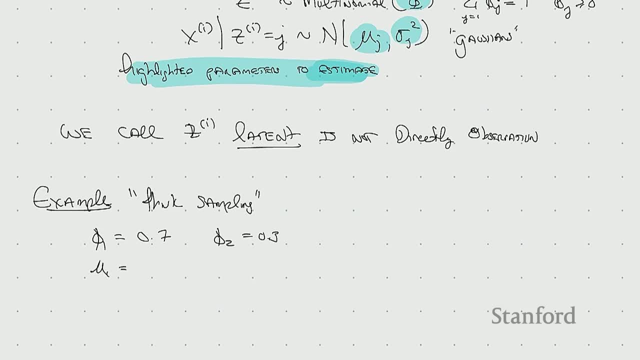 Why are those the numbers? Because I'm making them up. that's why I don't have another reason: Phi one is going to be mu one is going to be one, mu two is going to be two and I'm going to set sigma one. 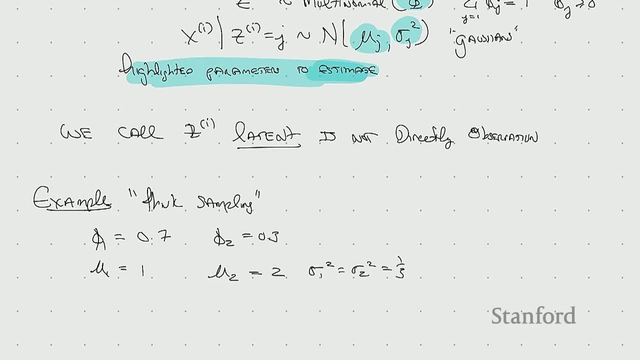 sigma two is going to be one and I'm going to set sigma two So we can see that sigma one equals sigma two. squared is about a third, roughly okay. So what does that picture look like? Here we go: There's one, there's two. 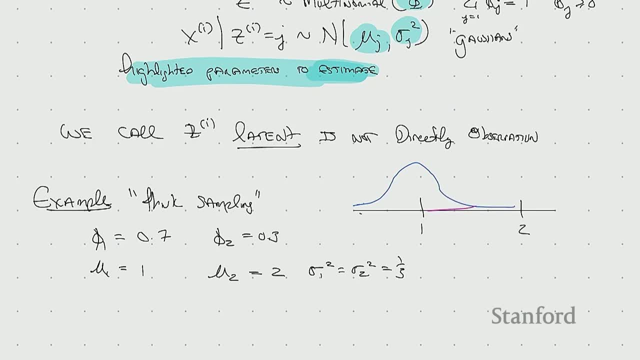 There's one thing here: if I draw it pretty well, Maybe my drawing is off, but hopefully you get the point. This thing should be about a third. this distance should be about a third. The fact that they're uneven is because I'm a bad artist. 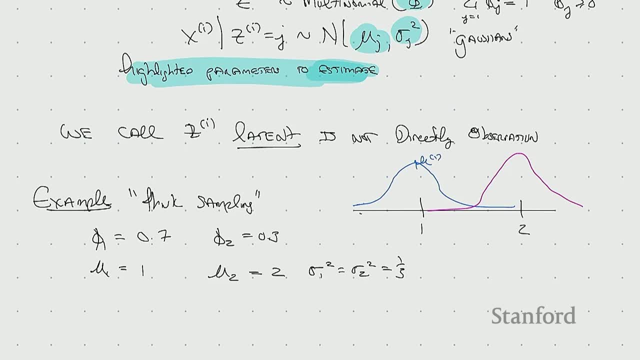 not, because that's the intention of the thing. This is mu one, this is mu two and this distance here should be about a third, the 65% standard deviation. Okay, How do I sample from it? First, I pick a cluster. pick one, either one or two. one of my clusters. 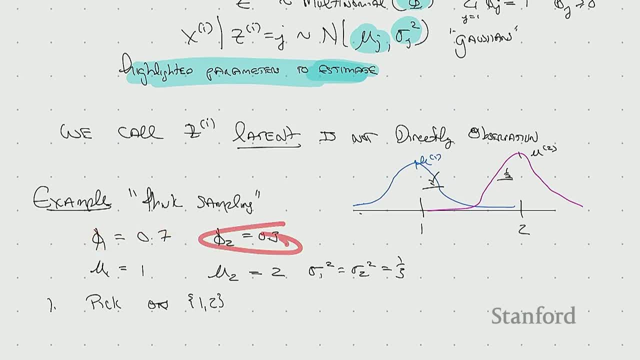 I pick the first cluster with probability 0.7, the second with 0.3, then I pick the relevant mean. So if I picked two, I will use mu two. I go over here, then I will sample from a Gaussian. 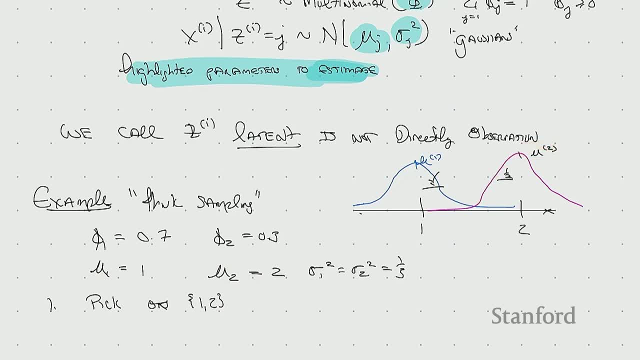 and generate myself a point. let me hear To use the appropriate Gaussian, okay, So imagine that this were the process that we're generating your data. you just get to see an instance of the data. your goal is to say what's the most likely process. that 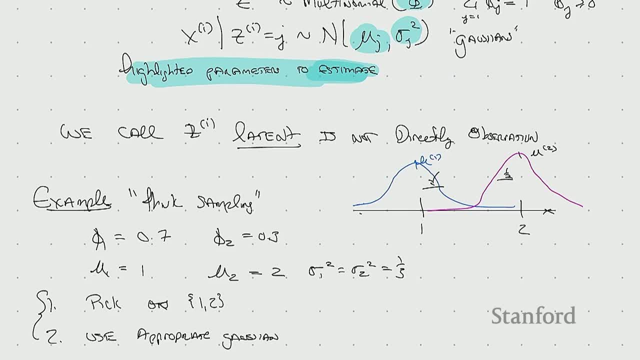 generated it. okay, And that corresponds to this intuition. like there exists some clusters, So far, so good. Oh, and then you repeat, Repeat: Yeah, please go ahead and ask questions. No, yeah, so that would be if I wrote their probability distributions entirely. 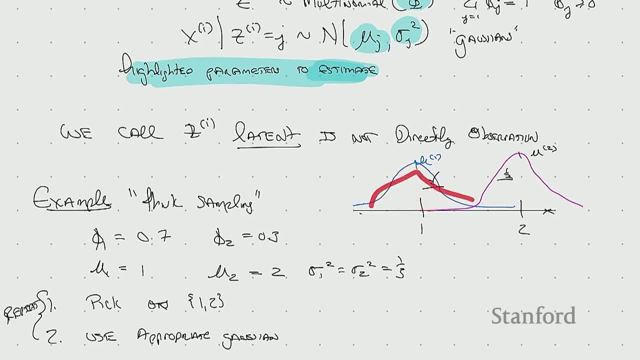 These are still unit normal Gaussians. this is a great question. I drew it as two Gaussians. I didn't draw the phi one and phi two. I incorporated them just in this first set. So I would pick, you know, phi one, I would pick one with probability 0.7.. 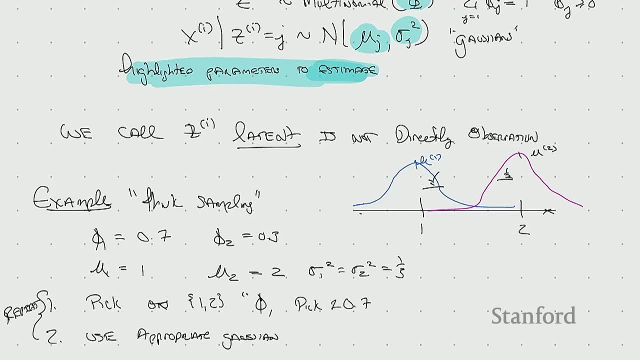 Pick one with 0.7, right, And you could imagine re-weighting them and normalizing them, but then it just gets a little confusing visually, and I'm not that good of an artist Because we don't know how many points come from every source. 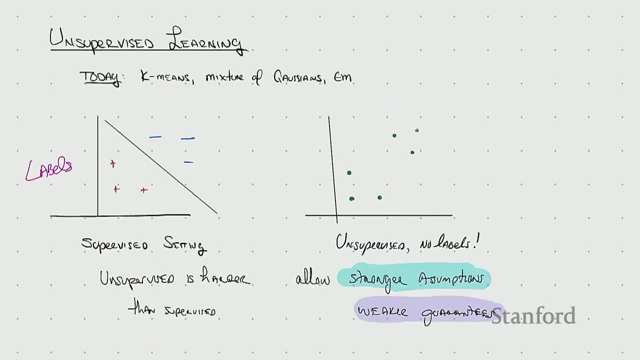 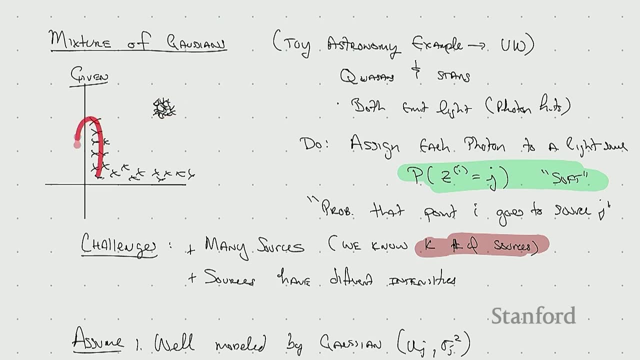 So remember going back to this one up here, We had like the oops, I went way too far back Here. we had lots of points from this one source and this point, you know, there's 70% coming from here, 30% coming from here. 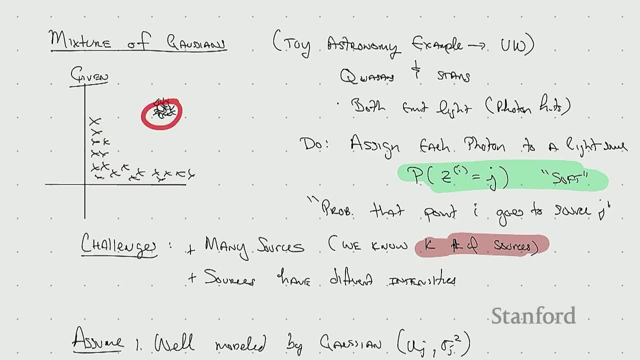 15 or 20%, 20% coming from there, And so they we can't. we're just not assuming that they have the same. If we force them all to have equally sized clusters, we would probably put two cluster centers here if this were 70% of the points. 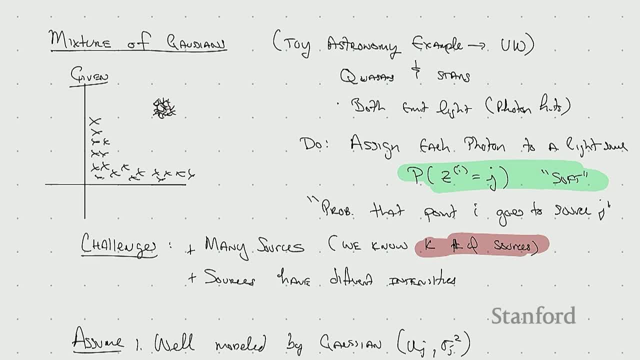 And we would use that to explain our data, and that would be, in this case, suboptimal. That's just our modeling choice. We know that the clusters have different number of points in our application, so that's why we fit them. 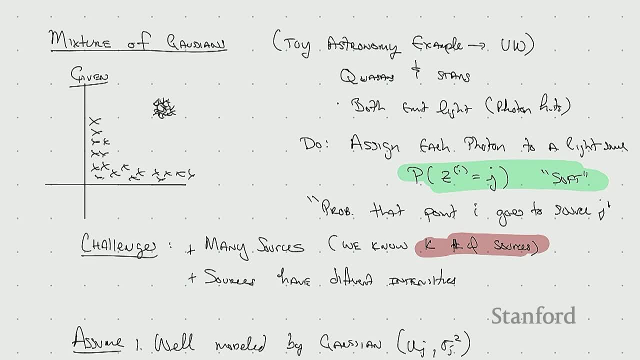 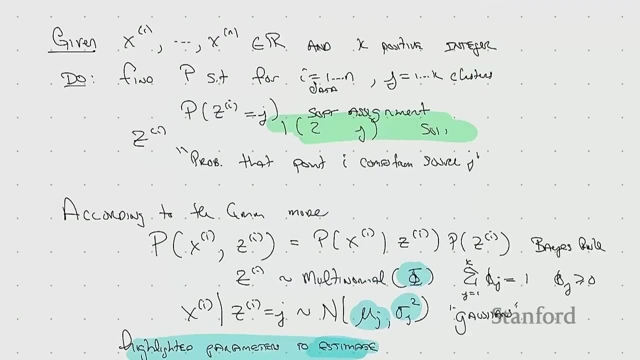 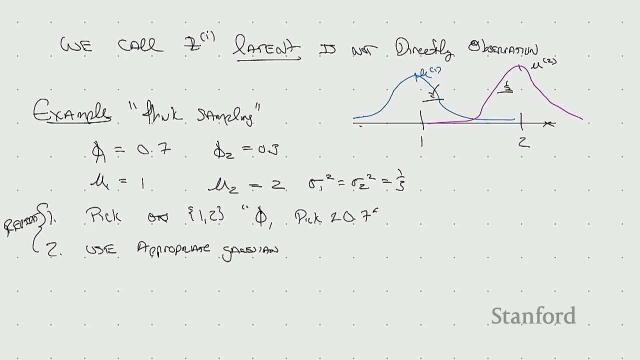 We can't assume they're the same. If we knew them perfectly, we knew the things. we could sneak them in there. but we'll talk about where we sneak them in later. And then the p represents the cluster sizes, and the m and v and then the mean at list. 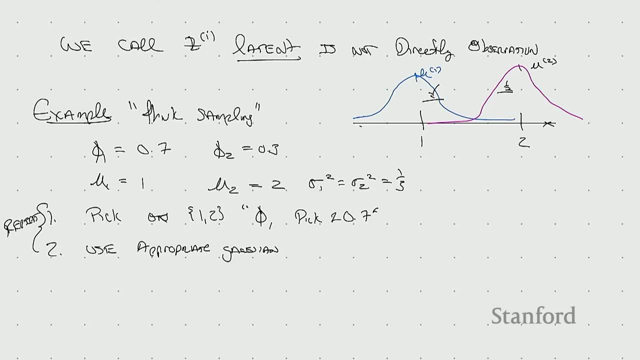 time duration, all the things, The shape, That exact distribution. They under, yeah, they understand, they're the shape, really Awesome, Sure. So basically, we have from p1, this pretty much, But why, like, the set of p is smaller than the present p? 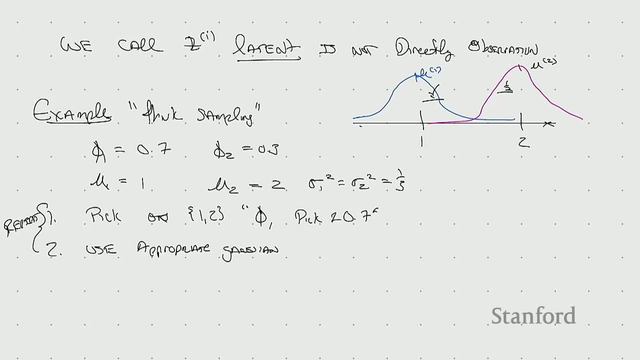 Yeah, yeah. So basically we have from p1, this pretty much the same, but why like the set of pieces smaller than the present p? I don't know, I don't know. Can you give me the answer? 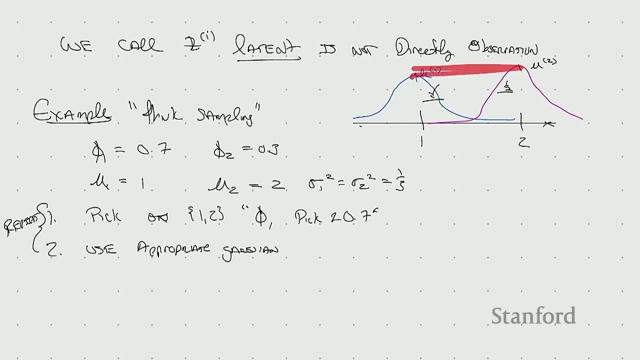 Because I'm a bad artist. that's kind of good. Yeah, that's a great question. So you could imagine for folding the Phi's in, to try and make them both probability, distribution density functions, where there was one Distribution density function, and then you would fold them in. I've drawn them. 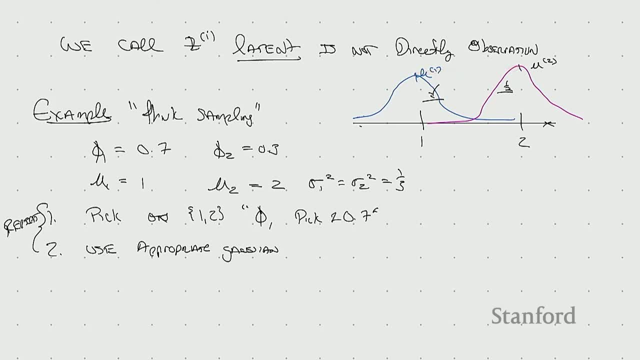 Crudely having the same height and putting the probability function up front to say these are the Gaussians, and then there's a height, But you've got it perfectly. Yeah, that's another way to visualize it, Which is, if this is beyond my archetype artistic abilities, like that's, legions beyond. So yeah, wonderful question. No, no, no. 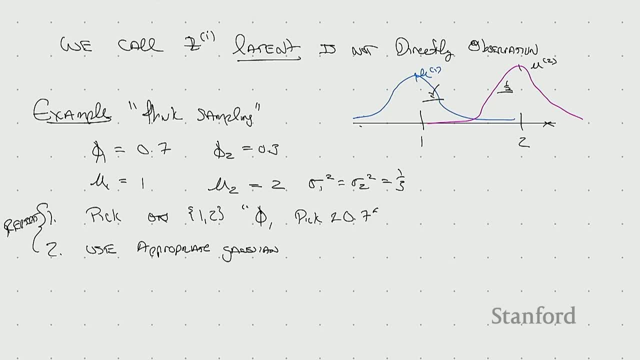 I did not have a lot of my ego tied up in that. Yeah, Yeah, awesome. So what's going on Here? the? the trick that we're gonna do is we're gonna assume like: okay, so every time you set one of these values, You give me a distribution. 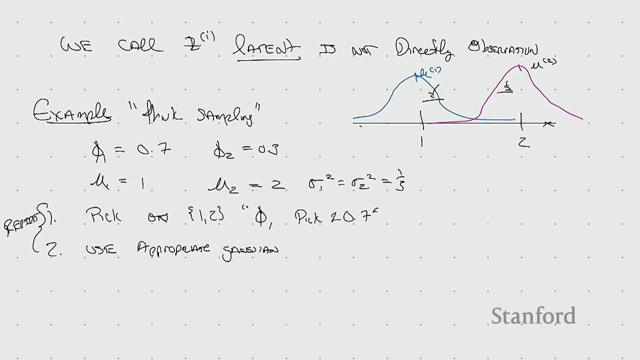 Right, that gives me a distribution. So now I have an infinite number of these things that are out there, with different settings of Phi, different cluster centers, different samplings. So now imagine your head like I grabbed one of them and then I did the sampling process and it generates some data. 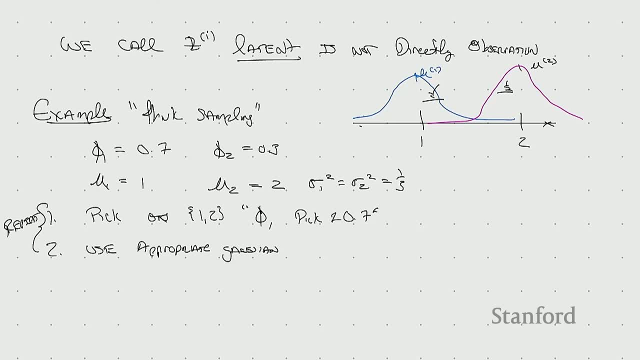 Okay, great, So we understand that piece. now I. what happens, though, in our problem is we're gonna invert that process, So we see some data just to excise themselves, And now we want to select among all of those infinite things that are out there. 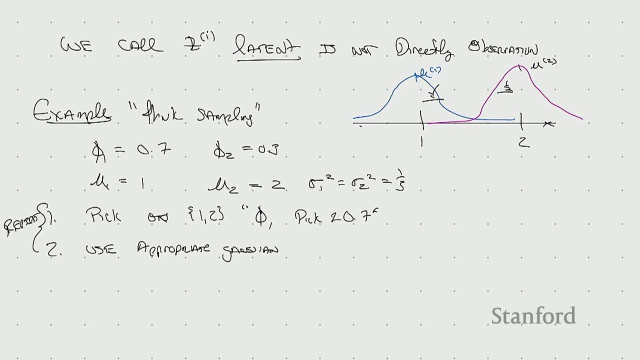 Which are parameterized now by these Phi's and mus and Sigma's, which one is most likely the one that generated our data? and intuitively We know, as I said, Like if the cluster centers are super far apart and our data is all in the middle, That one's probably less likely than one that has a cluster centers closer. 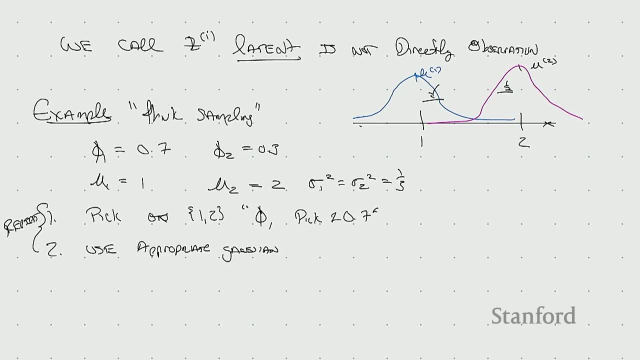 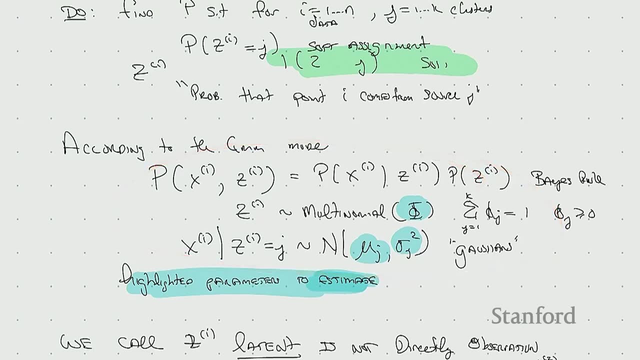 We're gonna be precise in a second about how we fit that, but you can kind of see where it's gonna come from. is This model? so, in the same way, we use maximum likelihood before we'll get there, We're gonna do a little bit more intuition. 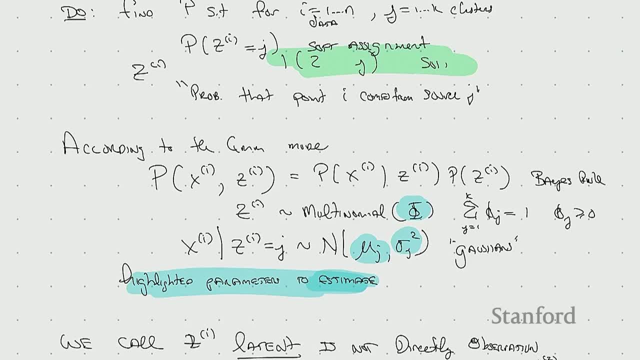 We're gonna say that the parameters that generated our data are the most likely ones after we've seen the data. So we'll condition on the data and try to invert it to find it. So this, this thinking of like the latent forward process, is super weird, right. 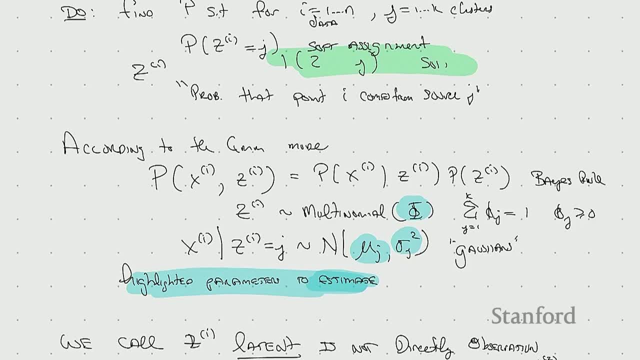 And so, yeah, you're exactly right. Does that make sense, though? We think about the process and then we're like, oh, if we inverted it, That's kind of what it must have been. Right, this, yeah, Exactly right. The thing is is we want to be exactly right. 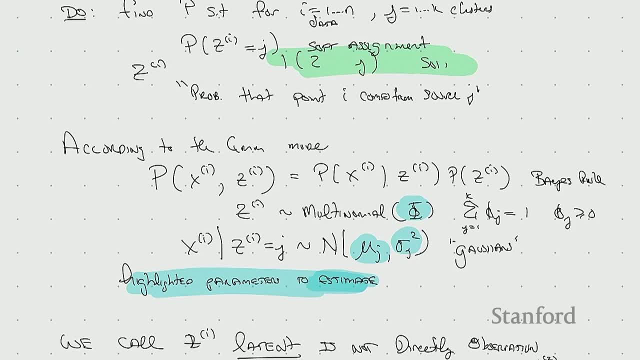 We could just guess all the parameters or try all them. promise There's infinitely many. So the question is: can we solve them and find them faster than that? Right, but if we could, just in theory? you know, There's well a theory is a weird statement, because there's uncountably many of them. 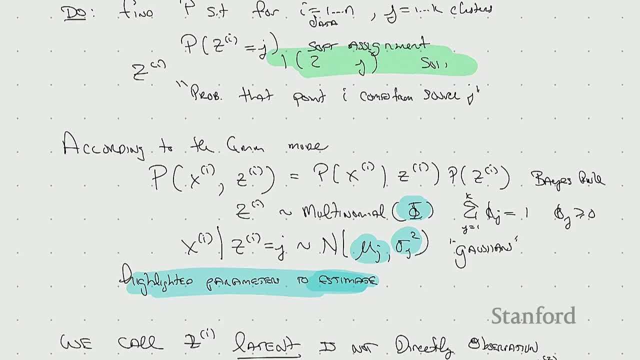 But like we could conceptually try all the parameters and then see which one was like closest in probability- You know How's the highest likelihood score- and we're gonna try and that's gonna be our gold standard of what we want to pull out. You got it perfectly. 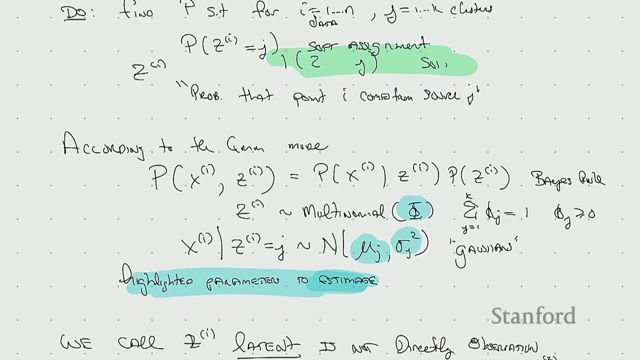 So I'm sorry I didn't catch the last piece. Yeah, in that case, if there's- only if there's only one value, then you know everything came from one source and you're just fitting a Gaussian. and the most likely estimate for a Gaussian is, if you saw, 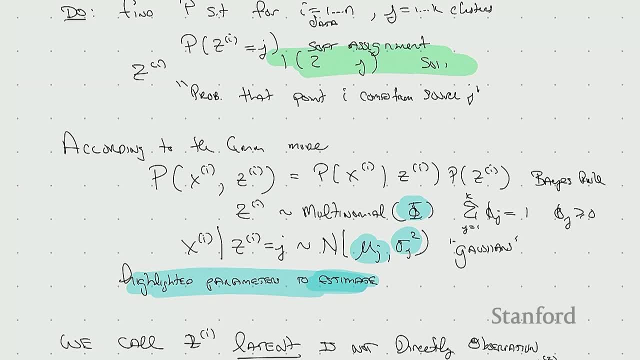 from GDA and everything else is Average your data to compute the mean, and then can compute the variance from that, and then you and then you have it Perfectly, wonderful, Awesome, we got this All right. so let's see the algorithm that does this, because it mirrors our friend k-means. Okay, 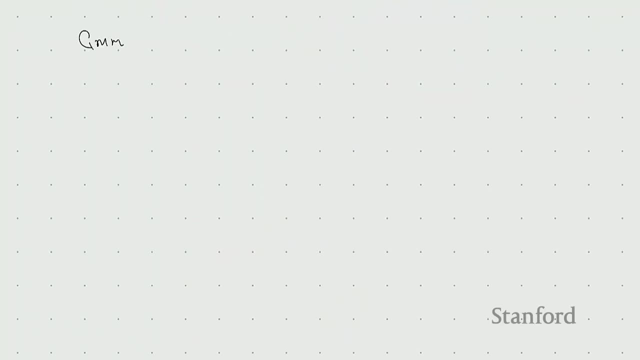 Okay, We're also studying this, by the way, because this same pattern will repeat itself in our next lecture. It's a famous algorithm, So it's fun to know about And it's important pedagogically. I don't know if you actually have to do anything with it in the class, but and it mirrors k-means. 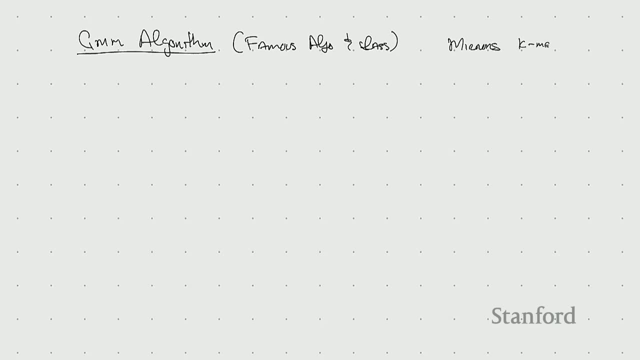 So like: why are we teaching These two things? they seem to differ in small ways and that difference, like k-means, seems a lot more intuitive than this whole Infinite number of models that we're selecting among. but we want to get to that worldview so that we want to relate the two. 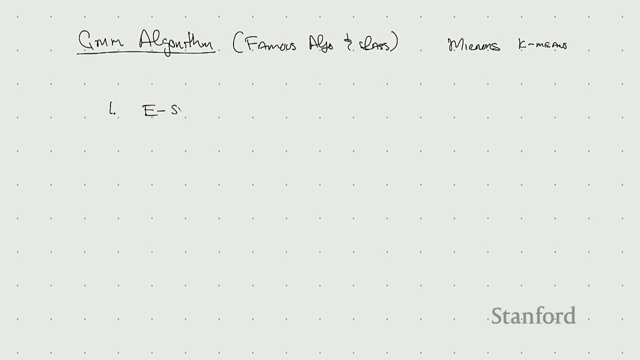 Okay, so one. There's an E step. Okay so this EM is very famous and we'll come back to that in a second. here We guess, just as you put it perfectly, we guess the latent values, Which, in this thing, are the values of the Z eyes. 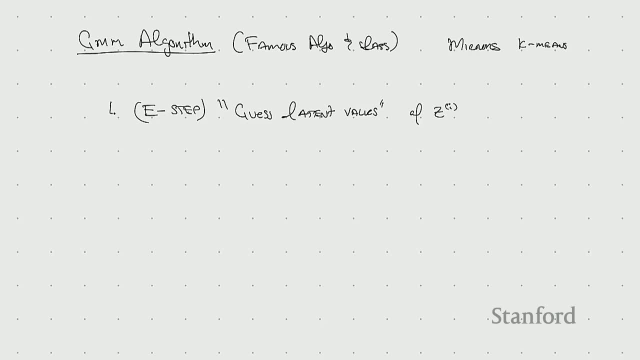 Okay, so we guess all of the cluster centers, their distributions. Okay, by hook or crook, We just figure it out. Okay, that's our first piece. We'll see how we do that in a more intuitive way. and then the M step: We update the other parameters. 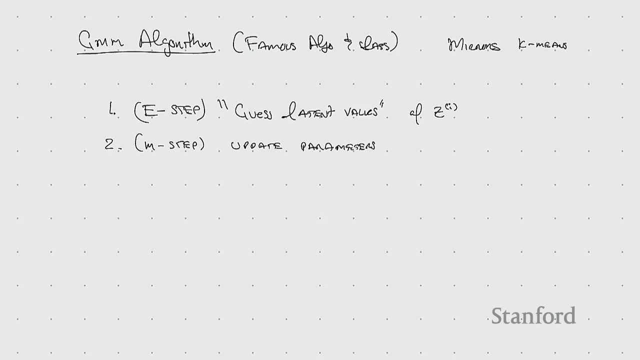 So if we knew the distributions, we knew my observation one. if we knew where every point came from, Then we could just run GDA on it. We could just run, you know, find which Gaussians are in each set. We just fit all of them. There's a slight twist that we're gonna not know where precisely every point is. 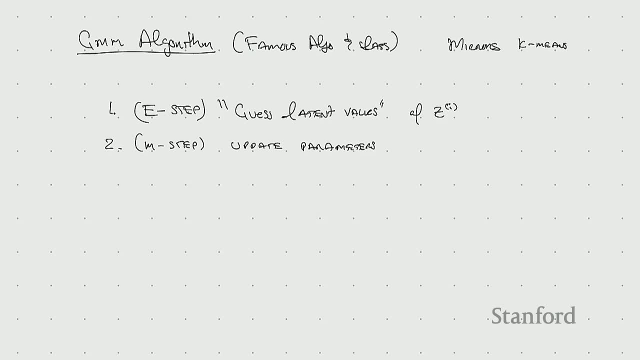 We're gonna know them a distribution. So we have to do something a little bit more complicated, but not too much more complicated. Okay, This is our first example of a very famous algorithm, First example of EM. EM is like a very, very famous algorithm that people like use for decades. I 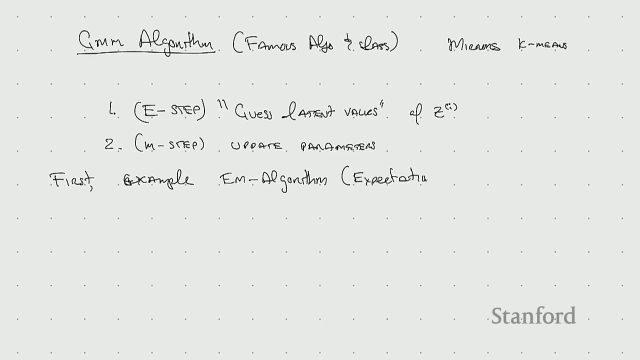 Don't want to oversell it. I have a colleague and friend who says you only Run it when you don't know what you're doing. and he's right in the sense He's kind of a curmudgeon. It's good, dude. 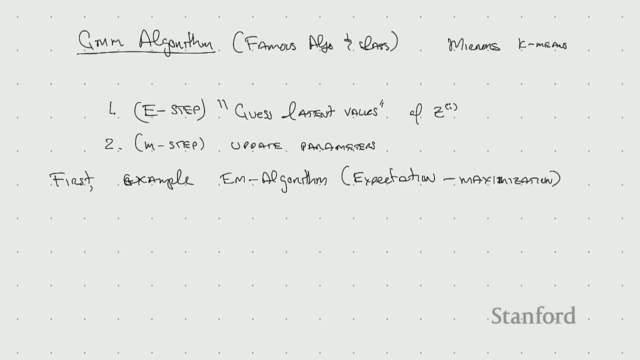 But he's right in the sense that, like if you knew exactly what you were looking for, you wouldn't run this algorithm. But that's precisely where it's interesting, because when you run these kind of EM algorithms, you know something about the setup. Okay, All right, So let's see mathematically what this looks like, and in your head you should be thinking: how do I? what did I? 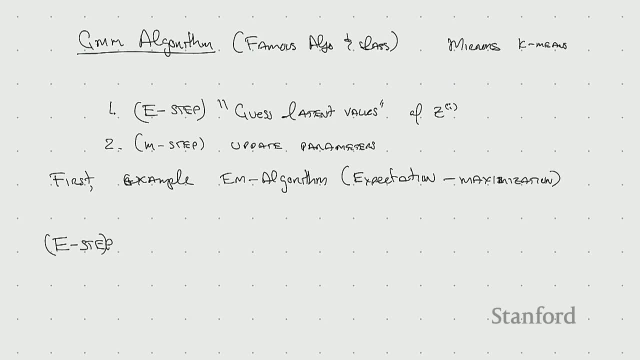 Do in. K means the E step. So here we're, given the data and Current values, which are guesses, for Phi mu, Sigma, blah, blah, blah, blah. all the stuff: Sigma 1, mu 1, mu 2, Whatever you want, all the parameters Okay, and our do is we have to. 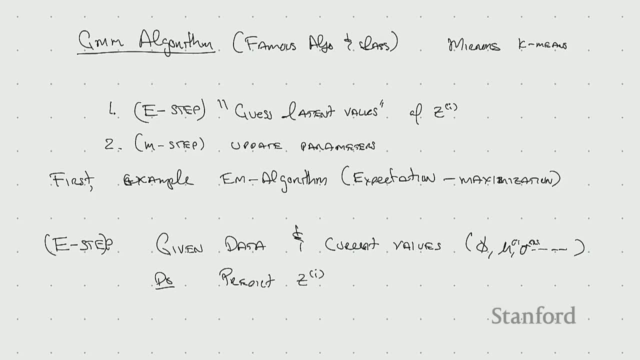 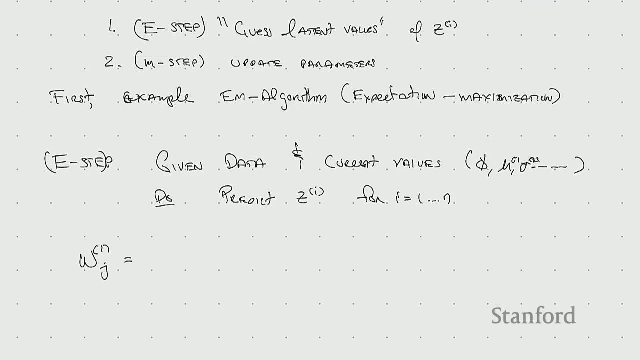 Predict Zi. Okay, for I equals 1 to n. All, right, now I'm going to introduce the notation here, following our notes: Given X i Phi mu Sigma. okay, So what's going on? Okay, This is our goal. Okay, so what? What do we want? 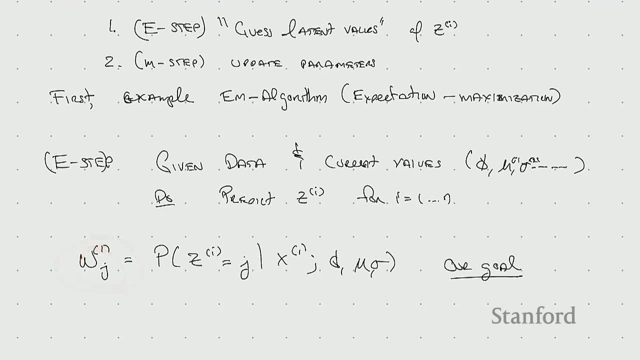 We want to compute these weights, which I'm just giving a new notation to, because Zs will be changing as we run and all the rest. We're given the data point conditioned on that. so we know the point we're looking at. We know all the rest of the parameters. 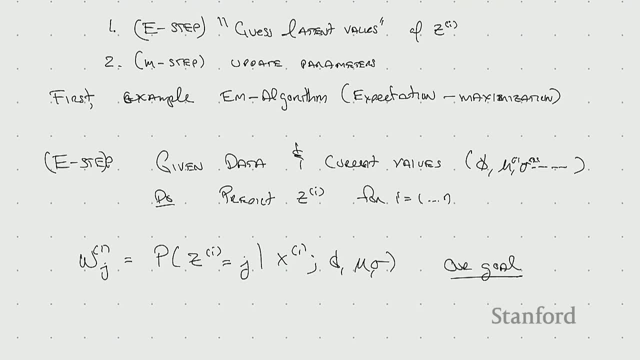 the likelihoods, the frequencies with which we're sampling from each one of them. We have our current guess. We have our current guess of how, where the center of every cluster source is, and it's variance. and now what we wanna do is we wanna compute how likely a particular point is. 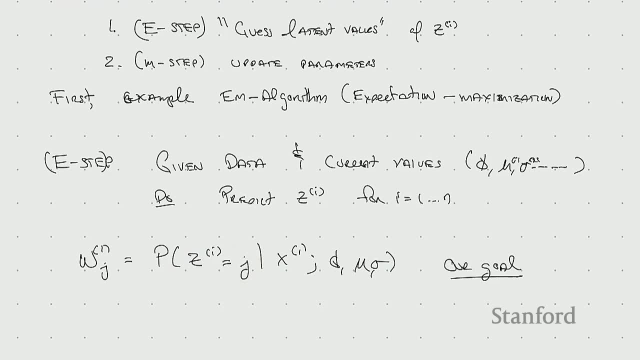 to belong to a cluster Intuitively. if it's really close, the probability should be high to the cluster center. If it's really far away, it should be close to zero. but it's continuous, it's not gonna be zero itself. 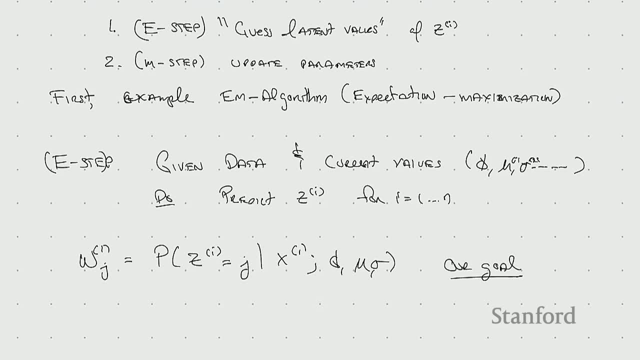 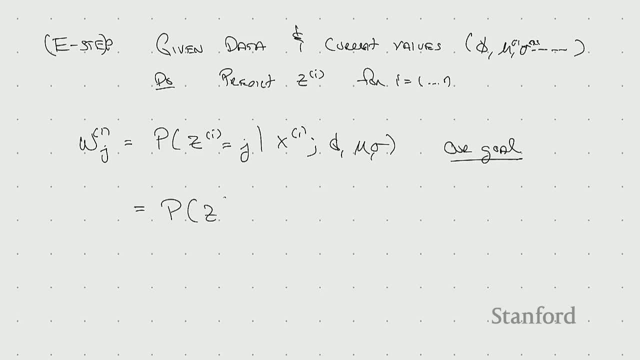 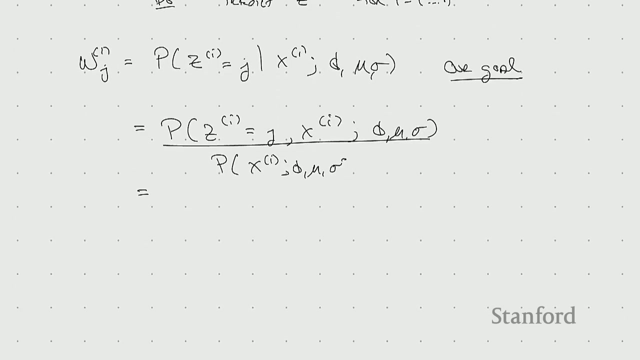 because the Gaussian doesn't go to zero anywhere. So how do we do this? Well, it's nothing more than Bayes' rules, Bayes' rule, Xi Oops, Sigma, Oops, over. all right, Oops, All right. 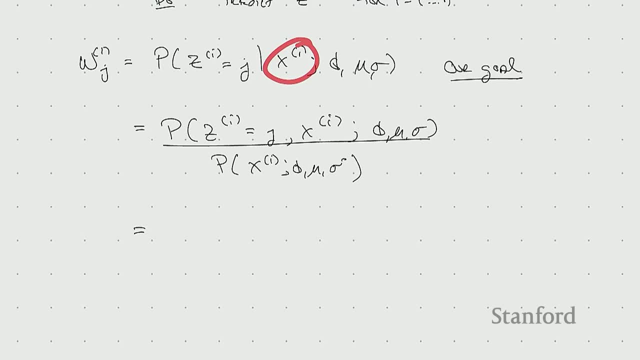 So all I've done here is something really simple. I've taken xi, which I've conditioned on it, and I've kind of divided it up. So this is like kind of the likelihood of the data being generated with this, which is a probability. 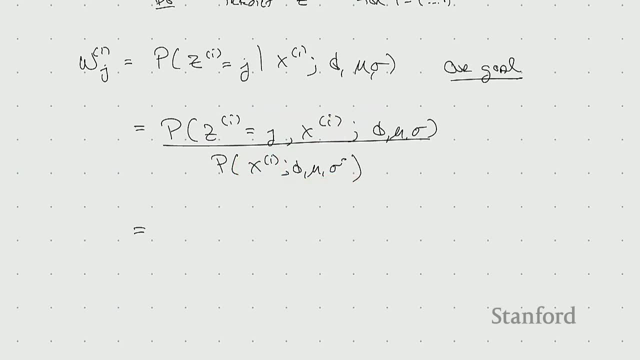 and then these two things being jointly done together, And then I'm gonna factor them out as I sum over all of the different probabilities. okay, So this is gonna be equal to probability of xi. okay, Oops, Probability of xi, zi, given j. 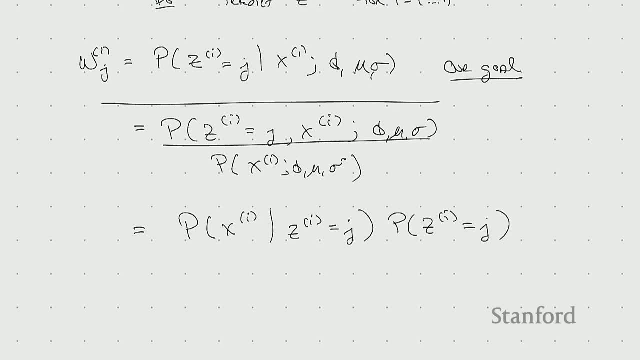 probability of zi j over sum. I have to use l here instead of j because I don't wanna confuse what we're doing. Zi equals l, comma, the whole thing. p. zi equals l. Okay, So the point is, we know all of these functions, okay. 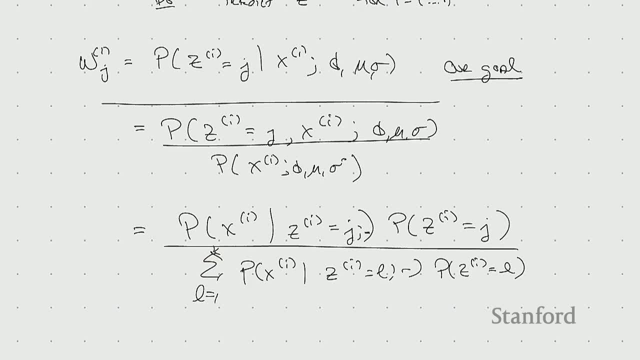 Oh, sorry, And everything here, by the way, has this stuff. We know all that information, so that's everywhere, okay, Okay, so we know all of the estimates and our guess. So what is this probability right here? Well, if we knew that it was a condition. 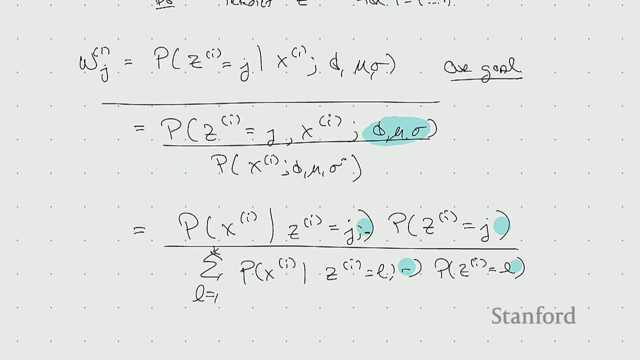 that we knew that this point came from the cluster. well, it's just a probability. Well, it's just nothing more than our friend, the Gaussian right. This is this character right here which I'll highlight. This is just a Gaussian. 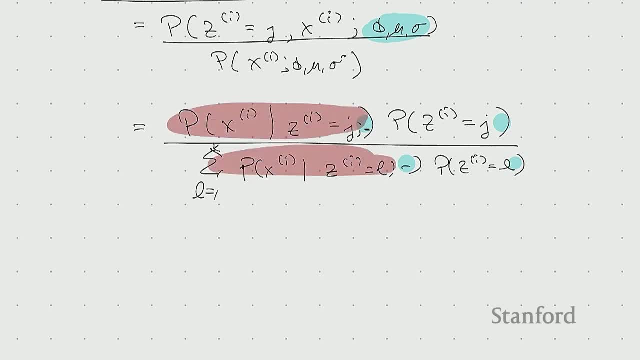 We know that from the model right. So is this right? So, if I can be really explicit about it, it's, like you know, exp of xi minus mu. i square over two sigma, i square right Times, some normalizing constant. 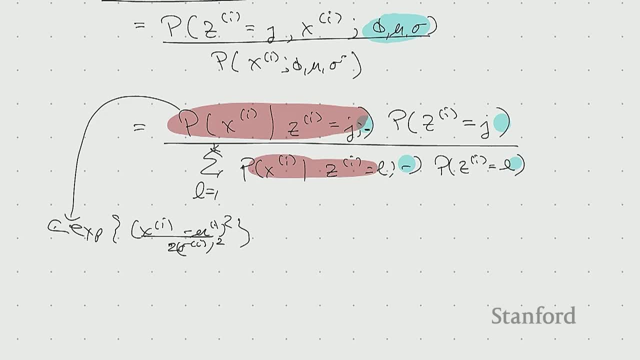 one over the square root of two pi. right, So we know what this is. What's this one? Those are our phis. So this character here. oops, I shouldn't use that color. This is phi j. This is phi l. 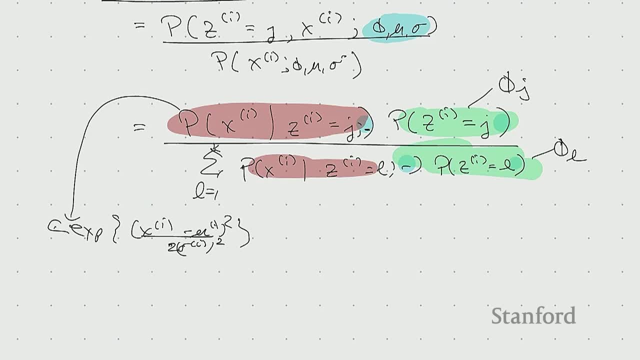 So I've decomposed the problem, once I know it, into estimating all of these quantities which I already kind of mechanically know how to compute. Okay. So the key point is, we can compute all the terms, Compute all the terms. Now, this isn't super surprising. 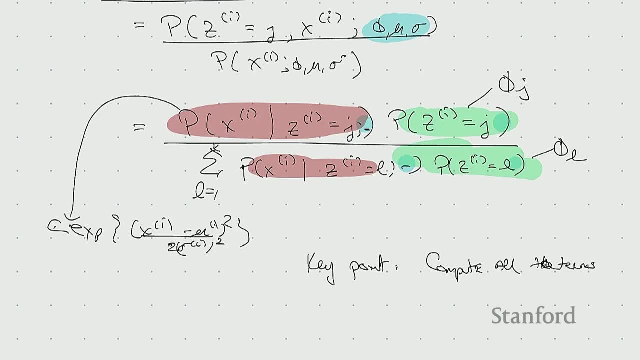 So maybe you look at this and you're like, wow, that's just a bunch of weird notation. What the heck is he talking about? Look, this is just k-means. It's saying in some kind of generalized sense it's saying I need to compute. 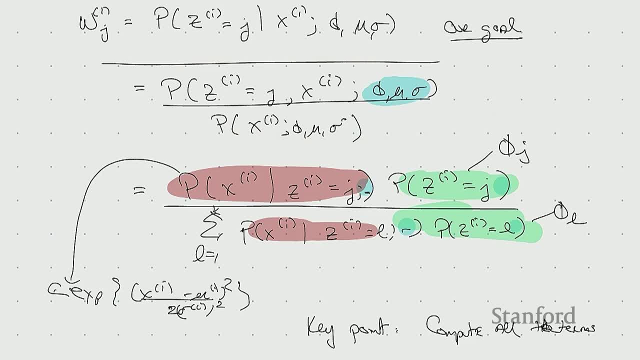 a probability distribution function. Okay, k-means doesn't need to do that, But how does it do it? It says: well, I consider the probability that this xi was generated from this j. I know how likely it is that a point came from it. 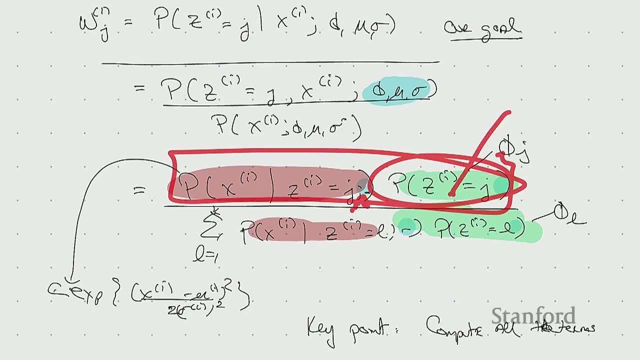 I know, given how likely, once I'm in the point, what the probability of this data point is. And then what I'm gonna do is I'm gonna compare it to the likelihood from every other cluster And that's the probability, right. 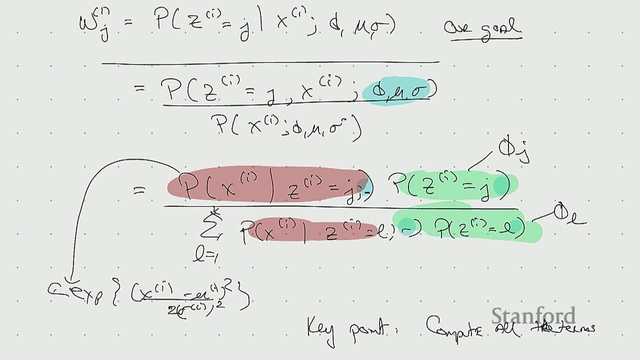 That's all it's encoding, Instead of having that hard assignment and saying which one's closest, like in k-means. this was just a max said. look at all the other clusters and you pick the closest one. Now I'm gonna average over it. 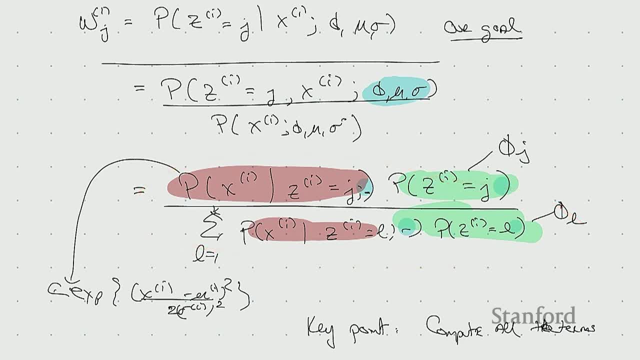 and I'm just averaging over it with Bayes' rule And it looks like notation. there's a bunch of notation, but it's not super scary. It's just things you know how to compute. Go ahead. They wouldn't be zero, but they'd be very close to zero. 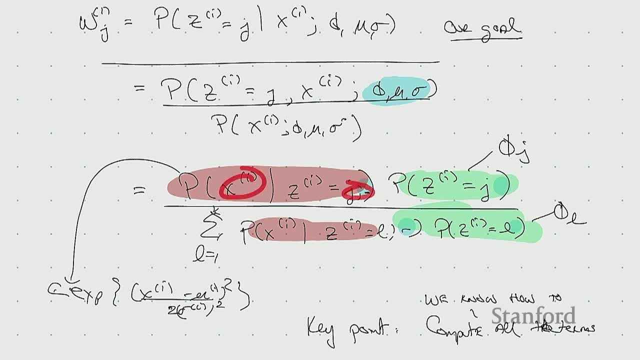 So what would happen in that scenario? So in your point, let's say xi is really close to this particular j. So this thing is very. it's not gonna be one of the thing, it's not exactly one, but it's gonna be some high number. 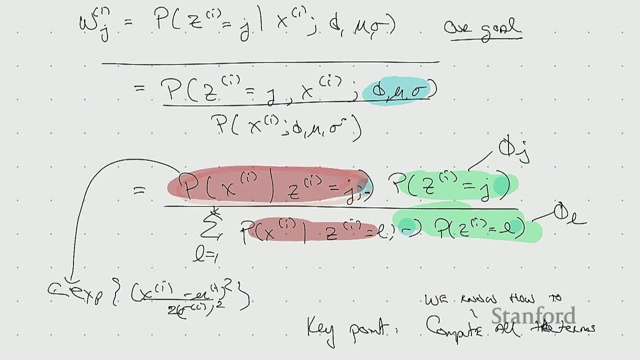 Let's say 0.5 or something, So some big, big number. okay. Then over here let's say phi j, that's the other term. So if phi j were equal across all the clusters, we'll come back to what happens when it's not in a second. 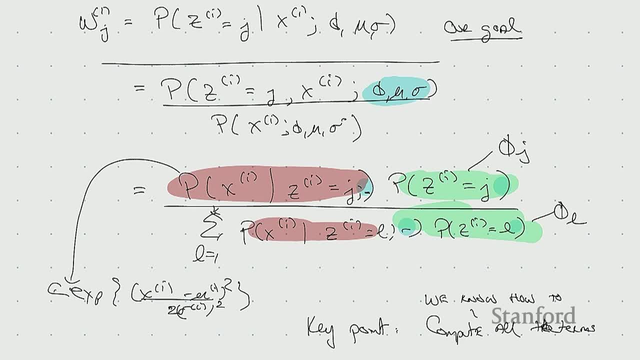 If it's equal across all the clusters, we get 0.5 times one over five or something, or five clusters one over five, And then we compare that likelihood to the rest of these And because you said these were really really far away- 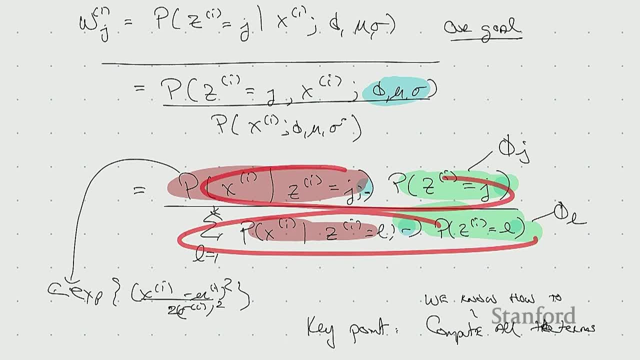 what happens here? You get this term repeated right, You get this term repeated right, So you get exactly that one term plus a bunch of things which are super close to zero, And so, as a result, this thing will be very, very close. 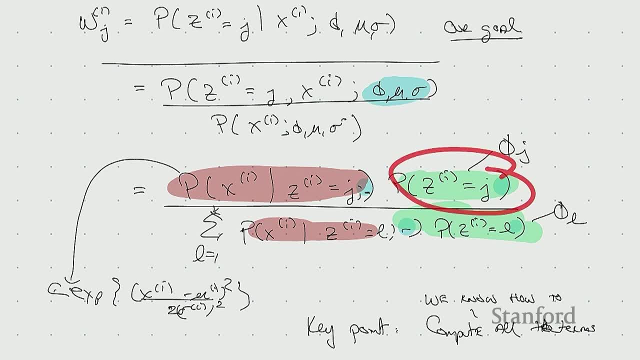 to one. yeah, does that make sense? Now, what happens, just in that inference, if phi j were very, very close to zero? So now there's this trade off As the point. if the point is like there's the cluster center and it's close, 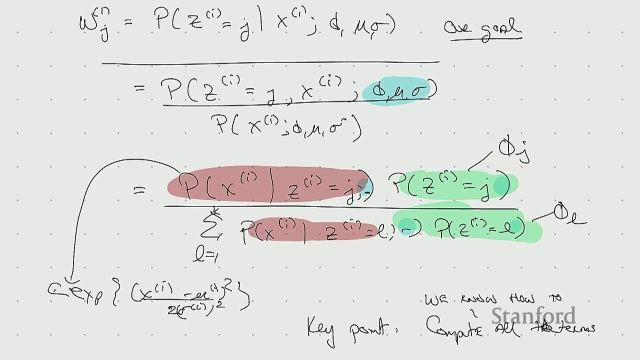 but I think it's extremely unlikely. like my phi j is like 10 to the minus 10, and I've only seen 1,000 points- I still don't consider it very likely that this source actually generated something Okay In that setting. 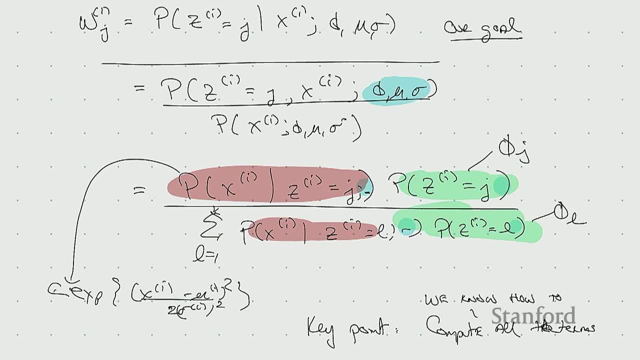 And that's all Bayes' rule does in general is trade off those two things. Does that make sense? Yeah, awesome, Okay, Right Now back to the oh please. Yeah, I just have a question. 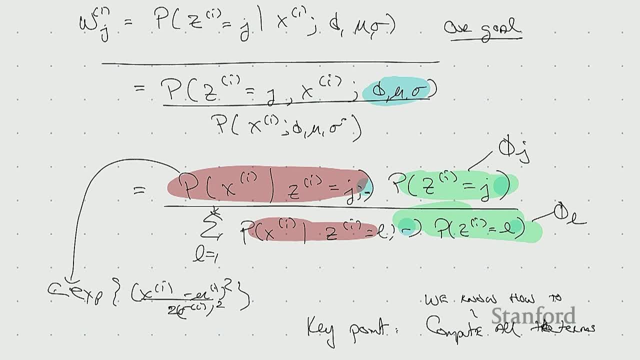 I'm a bit confused on the fact that phi j and phi l- those are like actual probabilities, whereas the probability of x, i is the probability density. Yeah, So I use them okay. so, yes, so you can do this because you can use. 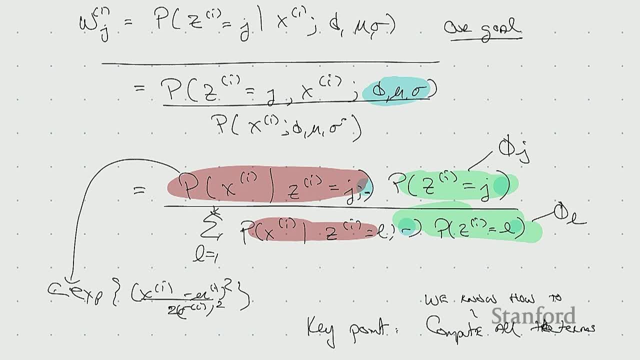 the likelihood ratios in this way. this is the correct thing to do from Bayes' rule, but it's a little bit sticky because this is just a PDF, but the fact that it's normalized up to it allows this thing to go through. 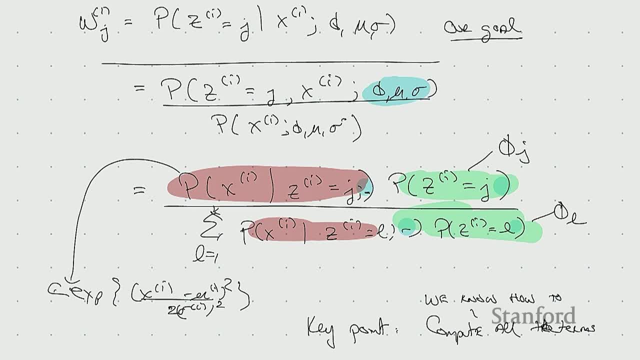 But yeah, you're exactly right, It's a little squishy but it works. Wonderful question, Awesome. So I hope what you got from this is- and also I want to come back- so that whole weird rant about how the data are generated- 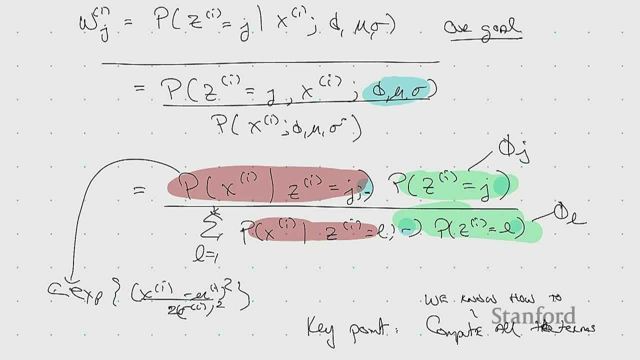 is now mechanically the way the math works. That's why I keep ranting about it. You pick a point, you generate the data. that's like assigning the likelihood score. When you wrote the generative model, you told me how likely it was right. 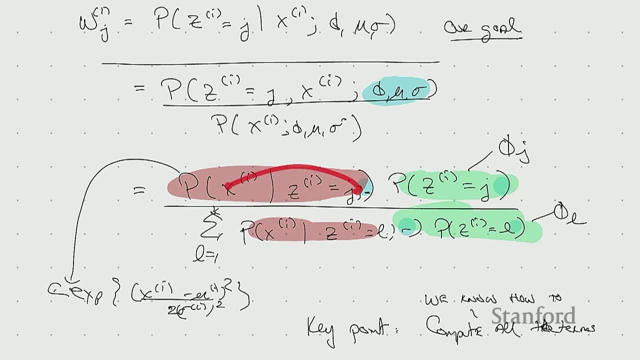 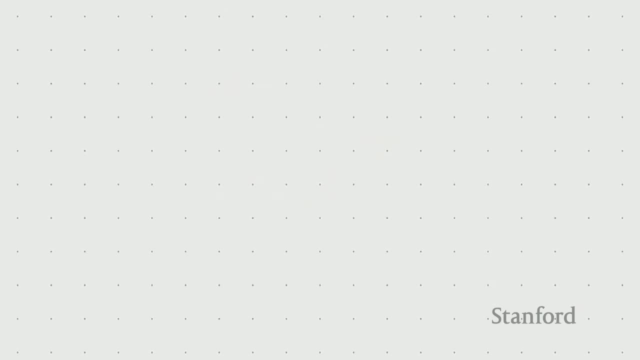 that, given you were in a particular cluster, that you would generate this point, that's the normal distribution. and then you compared and baked them off against each other and that gave you a probability distribution. That's it, Awesome. Now there's the other step. 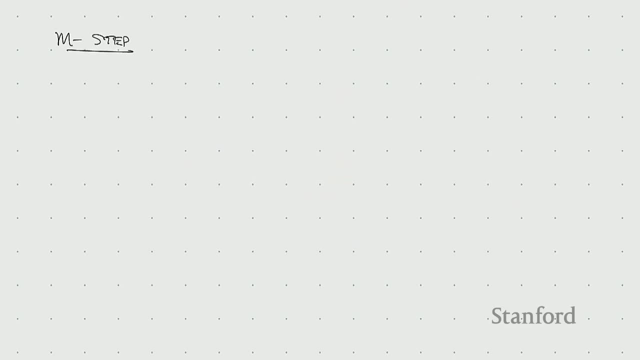 This step is much less interesting. So here we're, given all those w i, j's J, which is our current estimate. est of p, z i equals j. Okay, For i goes from one to n. j goes from one to k. 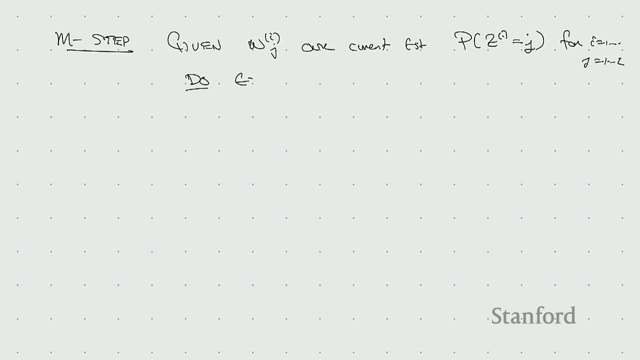 Okay, And what we have to do is estimate the observed parameters, The non-latent parameters. Now, this is conceptually interesting because, right, we split our thing into latent, which are not observed, the z? i's are not observed. 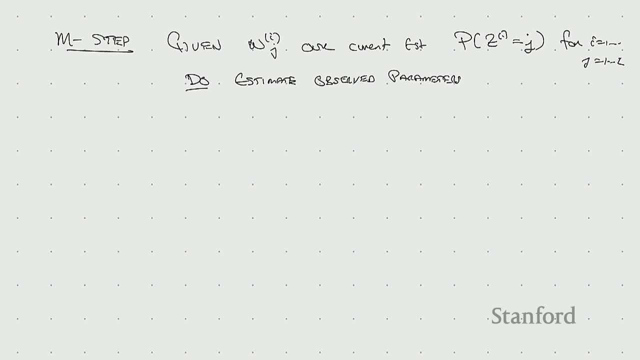 what the probability is that you were in a particular class and the things we did: observe The frequency. you know how many are in each class, you know their cluster sizes and all the rest. Like you can measure those things, Okay. 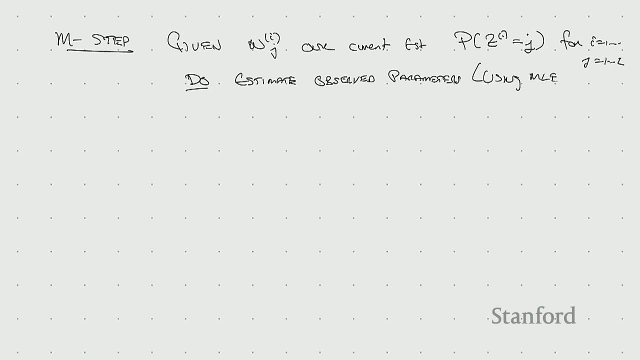 And we'll do that using MLE, because that's the tool we use. By the way, we use MLE a lot in this course, but there are it's not. it's very powerful, but it's not everything. I'll come back to that later. 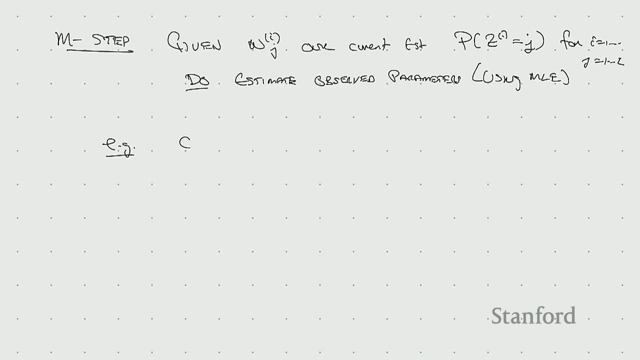 But that's, it's a principle, okay. So, for example, what is phi, j? What is the estimated frequency? Well, we sum over all the points. i goes from one to n of w, j, i. This is our guess of the fraction of elements. 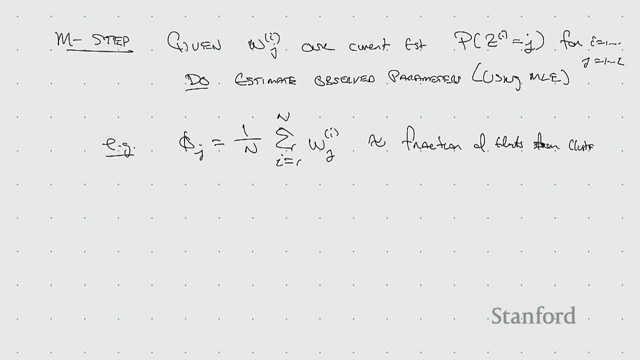 And from cluster j. We can make this a little bit more rigorous and we'll do it next time. And the point is, is you just do MLE? I don't want to go through these calculations because they're kind of boring. 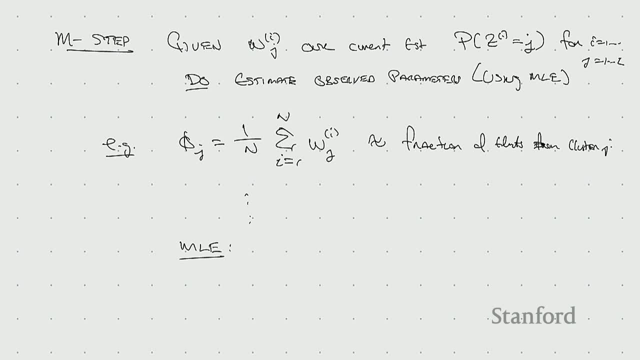 but you should go through them at least once and we can make that rigorous. And we'll do that when we do the MLE thing. so I'll do it in class. so don't worry, if it doesn't stick now, we'll do it on Monday. 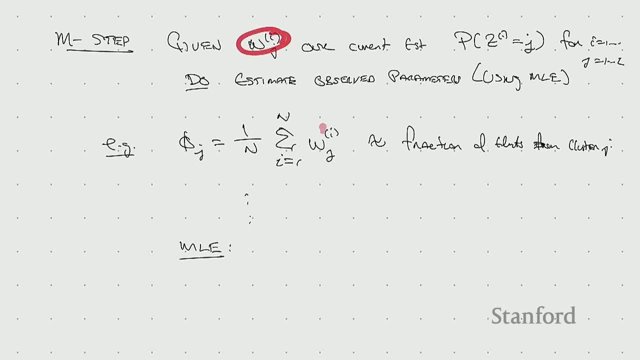 in a little bit more generalized setting. But what I hope you get here is, if I know the w i j's, I have to compute the estimate of phi j and then I just average over the probabilities And we'll make that, we'll do all the math to expand that out. 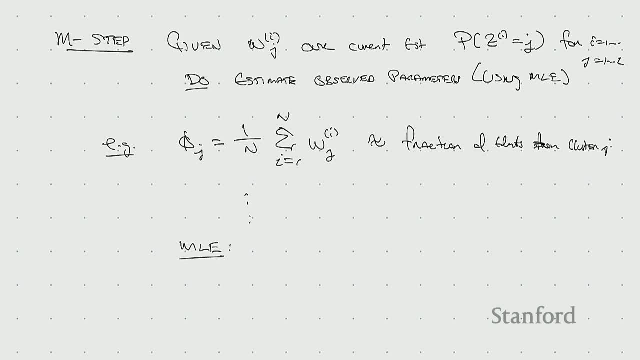 but you already know how to do this. This is just the MLE stuff that you've been doing for the last k weeks. Okay, So far, so good. Please, No, we're going to. we're not going to be. 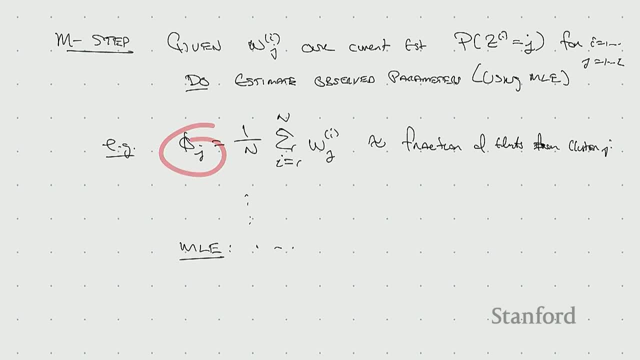 we're. this is the right answer. We're gonna derive this in more generality so you can solve for a larger class of models on Monday. Okay, Awesome, Please. Sorry, it's fraction of what from cluster? Oh, fraction of points. 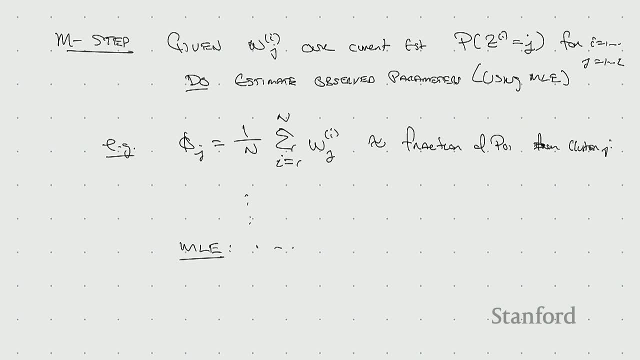 Sorry, that's really terrible. I said elements and then I don't know why. These are the points. Points from this should be source I kept using. I was trying to make source and target independent in my head and I did not use them carefully in this lecture. 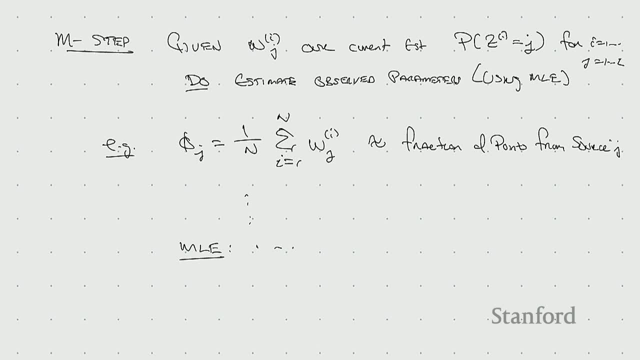 Apologies. Fraction of points from source j. Awesome Is the rough intuition of why this is. k means kind of similar to you. You pick a set of means which are like your sufficient statistics to describe your problem, Then you re-average over them. 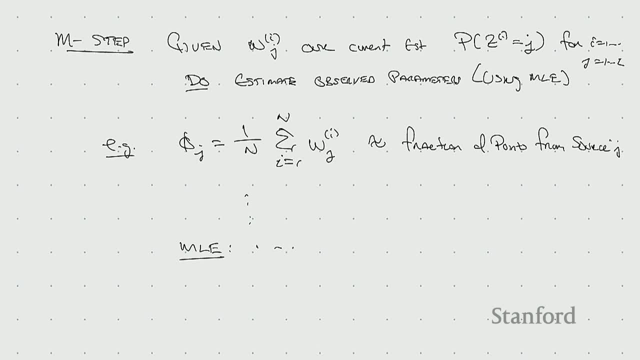 And what's going on here is you're picking a set. now, instead of just picking centers, you're picking distributions. Then what you're doing is you're re-weighting the distribution, saying if that was really the background probability of all these linkages. 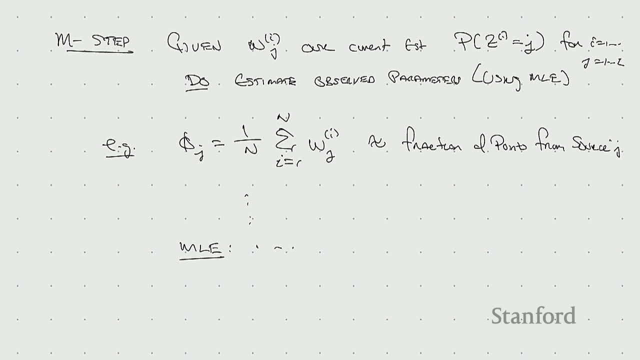 then this is what your most likely cluster sizes would be. This is how you know how much points you would have in each. Okay, does that agree with your guess? And you just cycle that again and again until you get back to the guess. 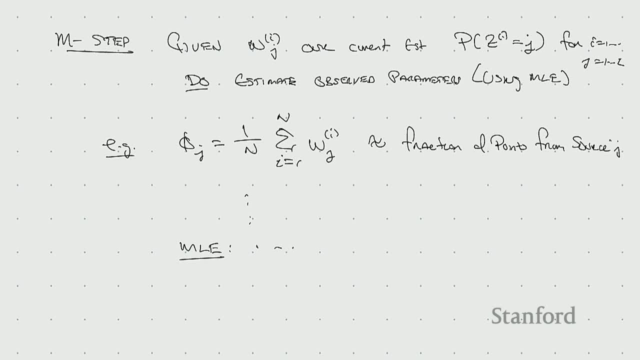 The same way you're doing. k means Awesome, All right, All right. so Yeah, please. What other EM models are we gonna show? A bunch, Yeah, a bunch Yeah. so, basically, an EM model can be applied whenever you have a latent z like this: 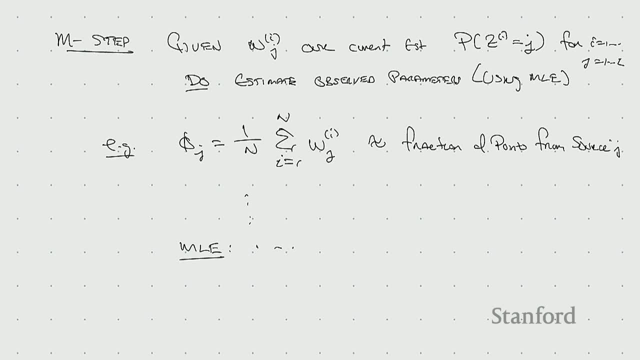 and you want to do some kind of decomposition to it. Yeah, it's going to have this two-step pattern where you have a latent z and then you want to do some kind of decomposition to it. Yeah, it's going to have this two-step pattern. 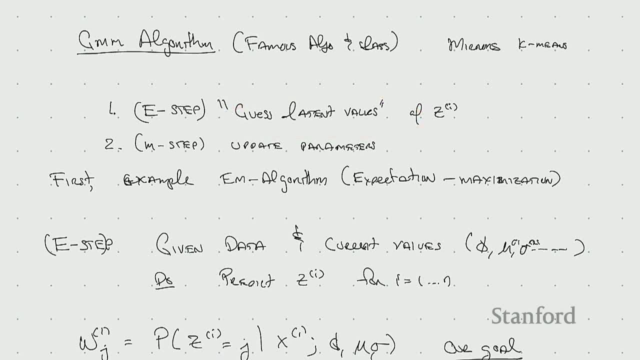 have a latent variable, and then I mean: it's not. there's no requirement that any of this be supervised. In some sense, the latent variable is like your guess at supervision. We'll see ways to inform so, for example. 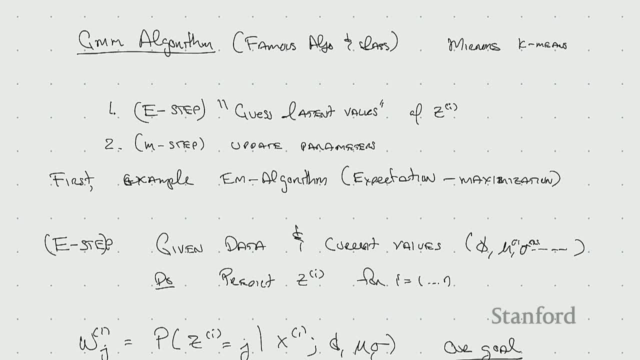 we'll see an algorithm where the first way it was derived actually did use EM. but there's a more clever way to solve it provably. but EM is the general form of like. there's a latent variable that you don't see. 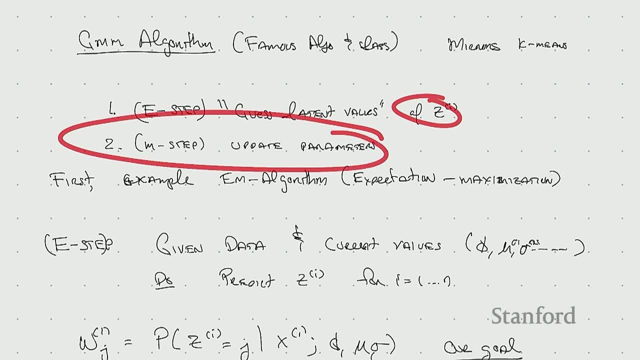 and you have a model for it. you estimate that parameter and then you solve like a traditional supervised machine learning or kind of estimation problem under the covers. yeah, and that's very, very general. Your latent variable here is clusters, but we'll see it could be distributions. 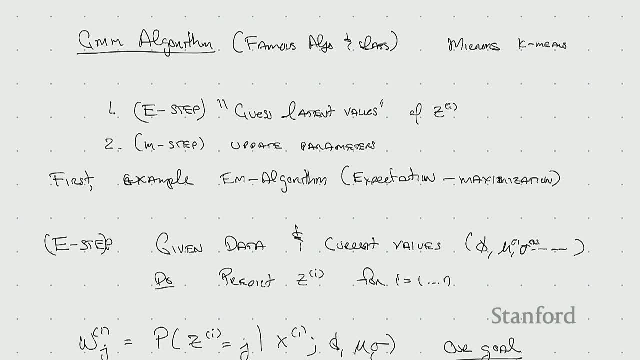 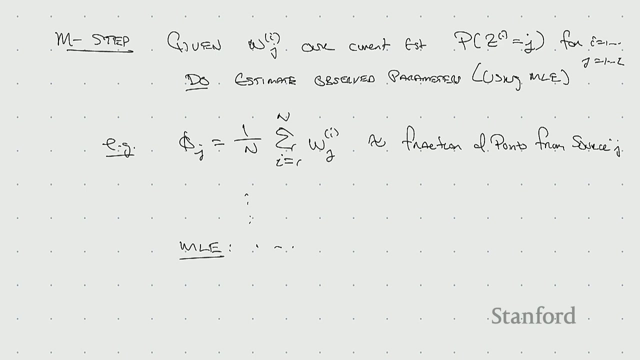 and all kinds of fancy stuff later. please Assume that we have an initial guess of a set of parameters. Yep, so no so, oh, great question. I see where the confusion comes in. No, so here it's like we are almost memoryless. 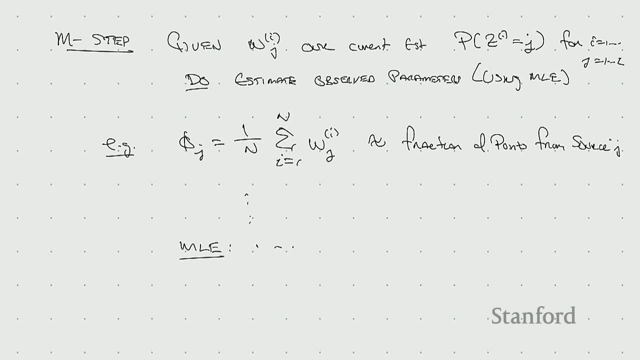 so we had those, you know, phi and sigma and all those other things, and now, just like in k-means, we throw away some information and we try to reconstruct it and here, given our link of PIs, we try to compute. 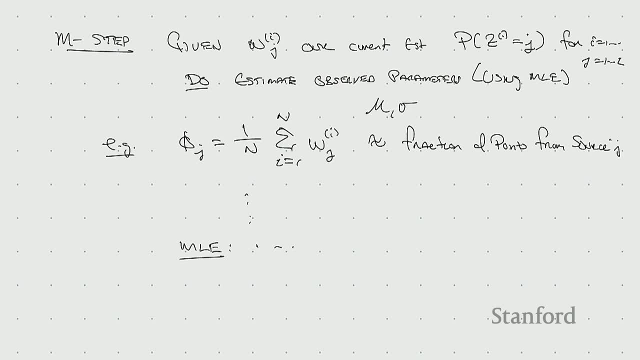 all of those observed parameters which are gonna be the mus and the sigmas and the phis and blah, blah, blah, the rest of the observed parameters. so it's like, given the linkage function, we do that again and then what we would expect is that those parameters 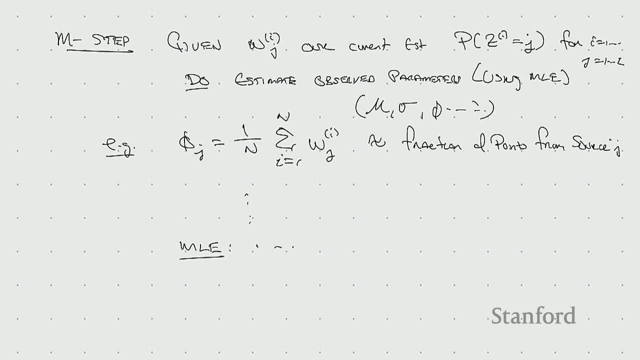 will not move around so much over time and that's when it will converge, similar to the way k-means worked. Great, great question, Awesome, please, Yeah, yeah. there is not something that has such a crisp solution to my knowledge. 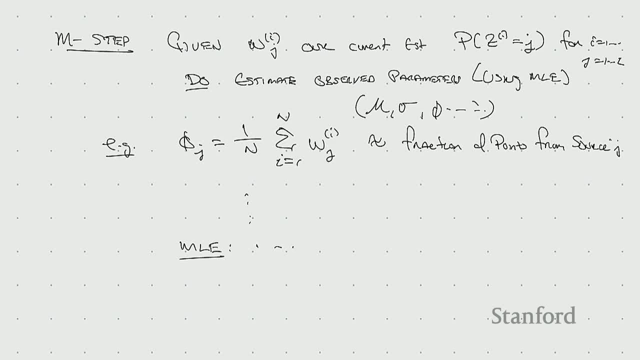 I don't actually know one, but that's a really good question. How do you initialize this and in what situations can you better initialize it? It seems natural enough to think about one, but I don't know a proof for one. Yeah, it's a great question. 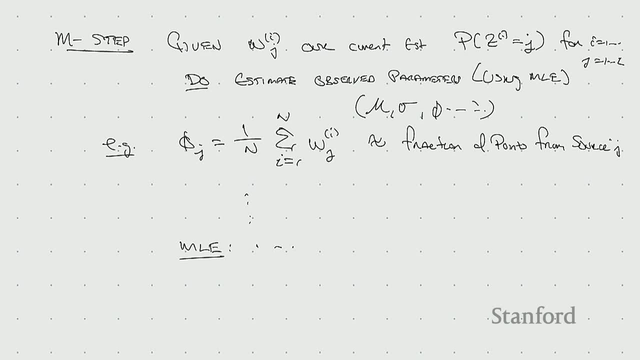 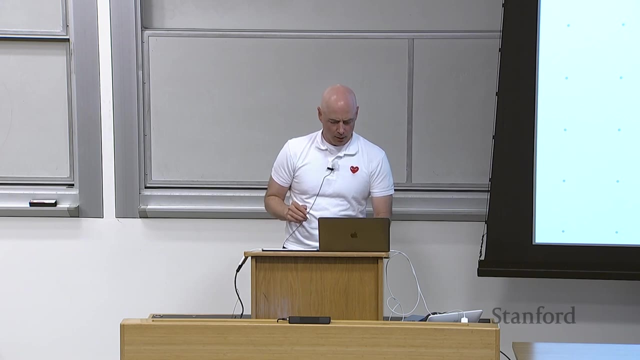 You can post it on Ed and I can dig around and see if anyone do that. My suspicion is yes, because k-means++ was such a important thing. It's a wonderful idea. Other questions, All right. okay, So looking at this, trying to think what I should tell you. 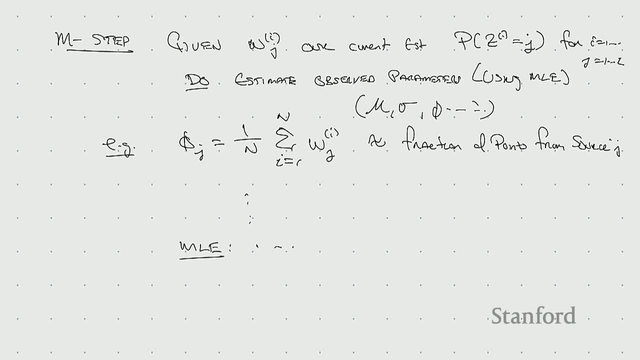 All right, so we have about nine minutes left. Let me see. All right. so what I want to do is- I think I want to- I want to just tell you the steps that we're going to go through next time, because I think over the weekend. 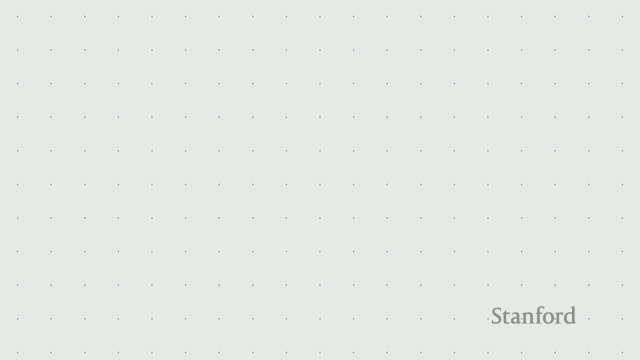 this will be too much. Traditionally, I teach it Monday, Wednesday, but I'm going to want to redo this. I think That's what I think. So, right now, what I want to do is have a detour into one thing that we need, which is convexity. 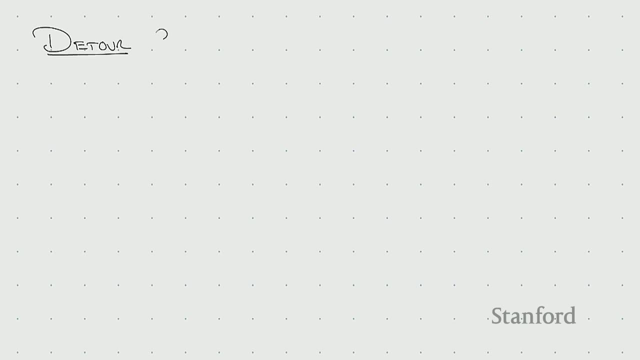 and generalization, and that's what I'm going to do. So I'm going to go ahead and do this. I'm going to go ahead and do this. I'm going to go ahead and do this. You can see, this is Dan Jensen's inequality. 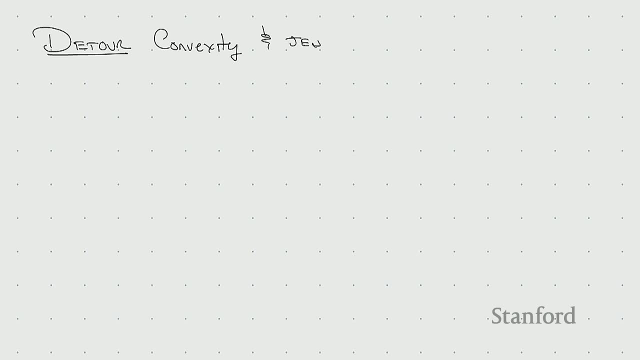 So I'm just going to draw the basics here, and then I'll give you a sense of what the EM algorithm looks like Now. the reason we need this is that this is a key result, and it confuses people every year, so I spend more time. 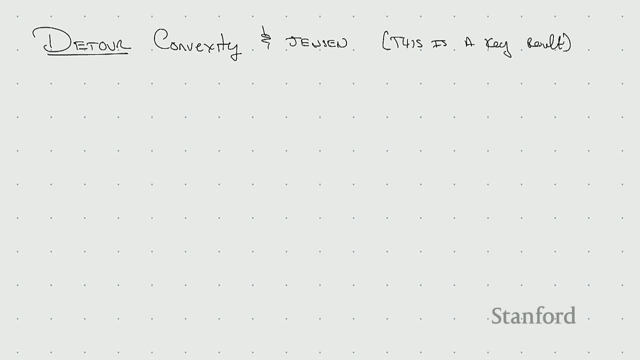 on it and hopefully it confuses them. last. Sometimes people say it's trivial and then I'm very, very happy. so if you think it's trivial, then I did my job. okay, All right, So what we're going to need to do? the reason I want. 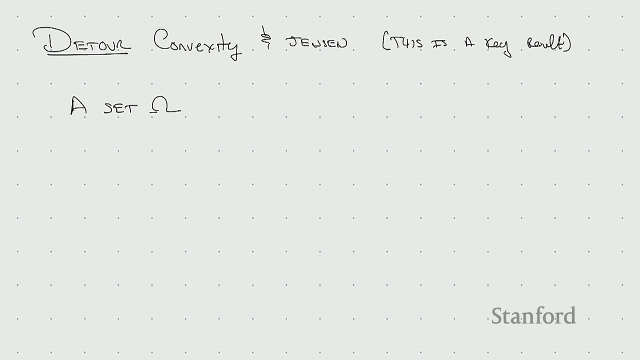 to tell you. this is what we're going to have to do, is we're going to have to have a mathematical abstraction of like this going to be back and forth and this guessing back and forth, and that's going to be basically two. 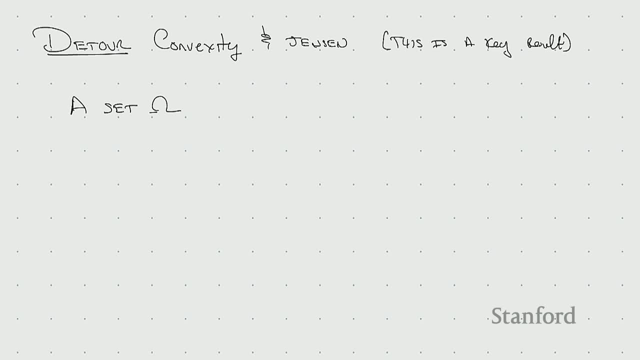 different functions. One function's going to be a lower bound of the function. there's going to be the actual loss function for the totally crazy probability distribution that has all the infinite models and everything jointly together, the actual likelihood function and what we're going. 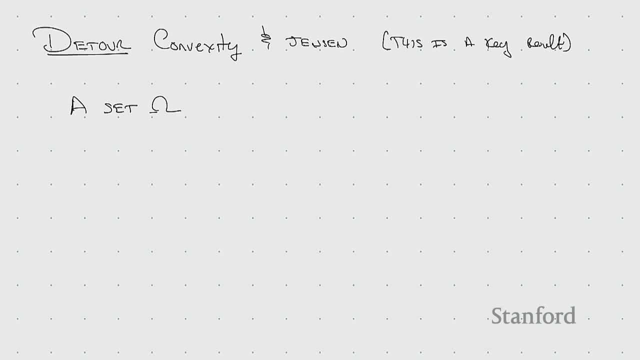 to do is we're going to have an approximation of it. that says, given we have a particular guess of the ZIs, we're going to have this lower bound and we're going to have to move between the lower bound and the upper bound and the lower bounding function, and that 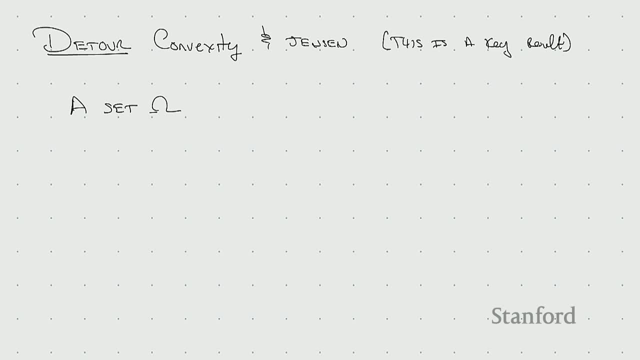 is going to be facilitated by something called Jensen's inequality, and it's worth understanding because it's something that you can use. So I'll just get started a little bit on it and draw some pictures, and then we'll pick it up next time. 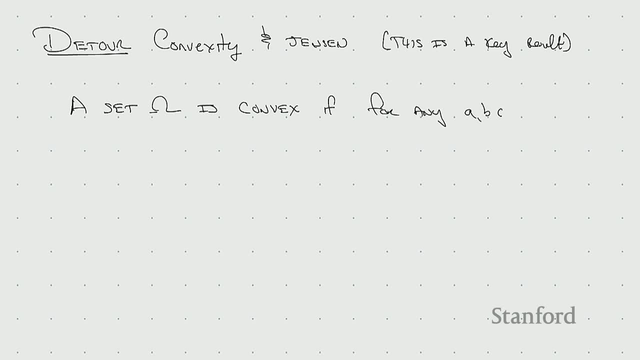 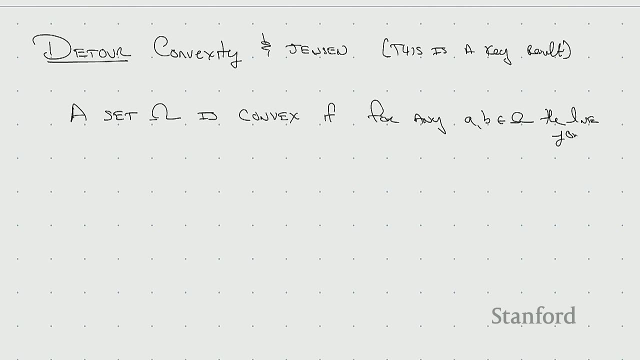 And I would certainly rather answer questions, because you know we can cut into later lectures so we don't need to rush. Okay, AB is in omega, So let me draw. Okay, so something is convex if the line joining them is inside them. 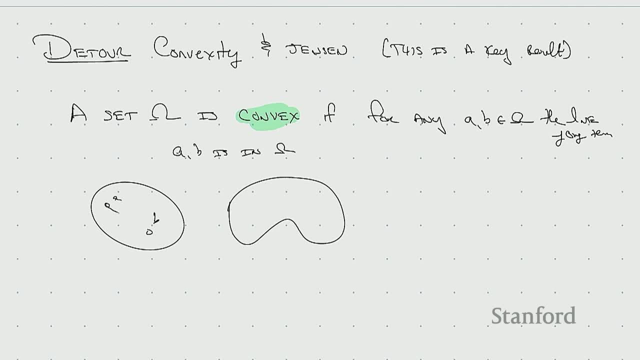 So like if I take any two points in here, any A and B, and I draw the straight line between them, or in Euclidean space, so it's a straight line, then if it's convex, then no matter which points I pick, the line between them is going to remain in the set. 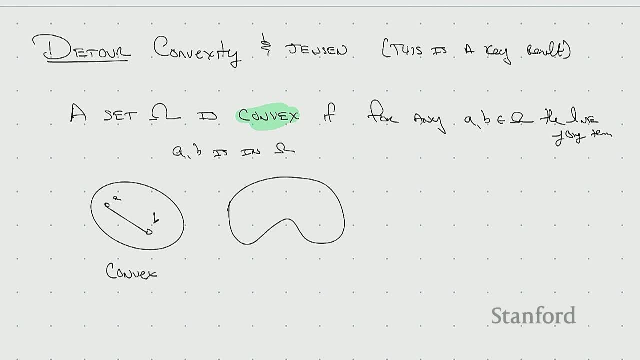 This is a convex object, so like an ellipse or a circle or something like that. In contrast, here if I pick points A and B, then I draw a straight line between them, and if it's A and B here, this is not convex, okay. 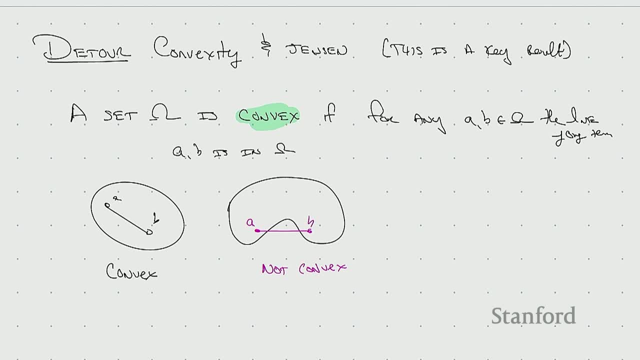 And these are going to be, you know, yeah, we're going to care about these quite a bit, okay. So what does this mean in symbols? In symbols, we have to check for all AB in omega, which is our set, omega lambda, A plus. 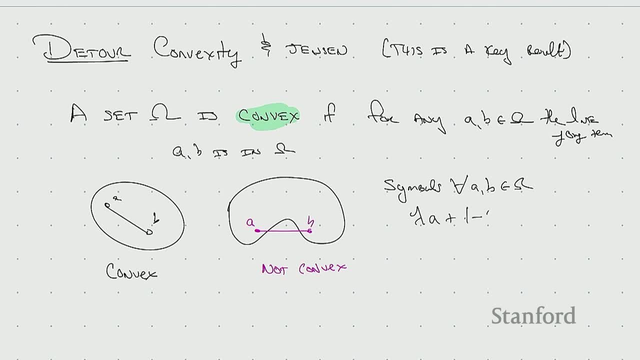 1 minus, oops, 1 minus lambda B- That's the line between them- is an element of omega And lambda here is an element of 0, 1, okay, That's all this picture is saying. This picture and this math are the same, okay. 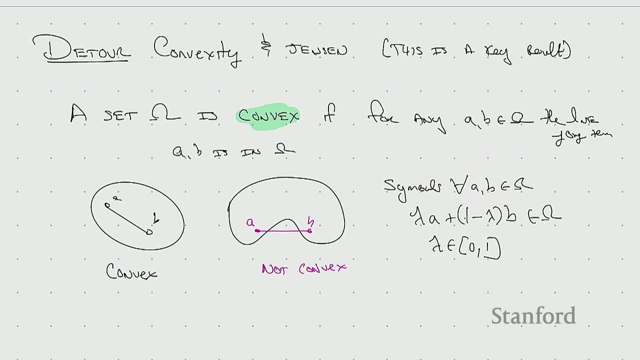 And you need to check for all right Right here. clearly, if I put A here and B here, there's a line between them. The reason it's not convex is there exists one pair of A and B for which I go out of. 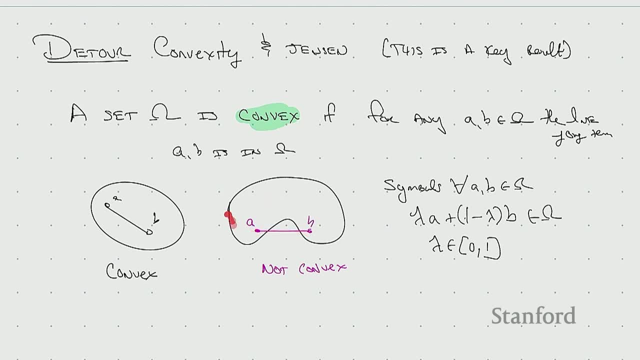 this set. okay, Now we're going to use it. when this bottom piece is a function, right, We think about the function going up to infinity, The graph of the function, The function being convex, And what this tells us is, if we look at chords, that is, points between the function, like this: 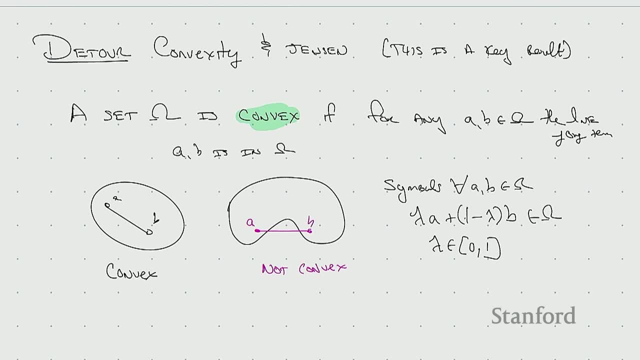 they should always be lower bounds to the function And that will be a little bit opaque, but I feel like you think about a function that looks like this: the x squared function that set will be convex. That's the canonical convex function. okay. 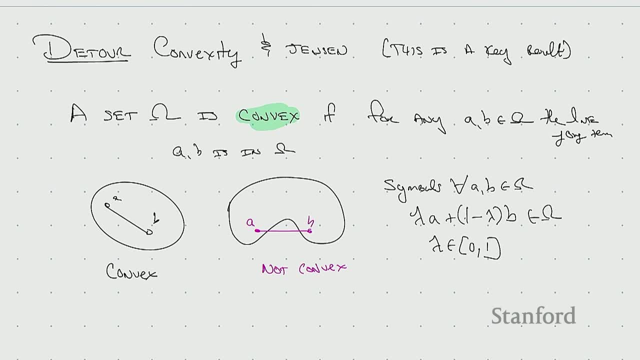 All right. So what we're going to see is we're going to go from these definitions of convexity on sets to convexity on functions, And that's going to allow us to, And that's going to allow us to basically prove the following statement, which we will: 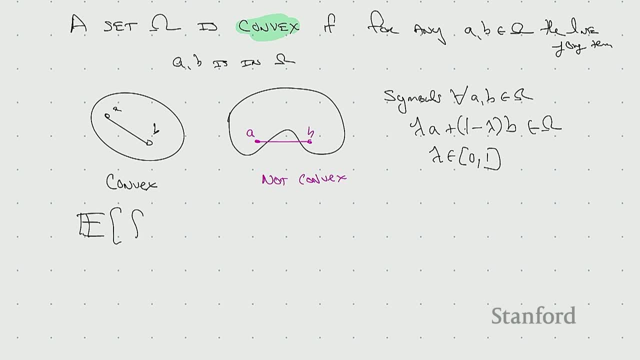 prove next time, which looks mysterious but is not, and you'll see, this is greater than f, of e, of x, okay, So there's going to be. We're going to show next time. just I want to give a little bit of a roadmap. 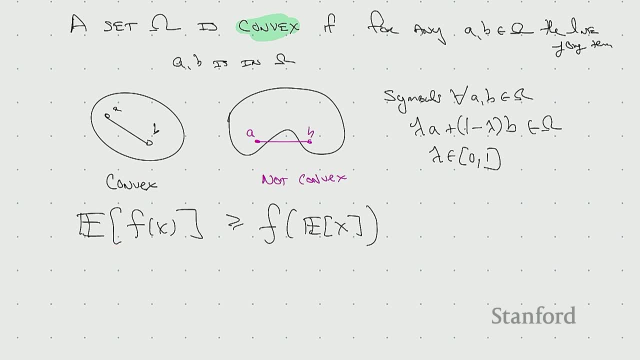 We're going to use this definition of convexity to prove a theorem. This theorem is called Jensen's theorem and it's effectively immediate from the definition. Once you understand the definition of this for functions, you're going to be able to use it for functions. 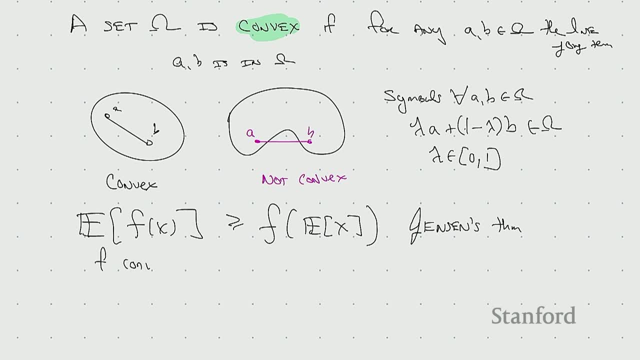 If f is convex. this is true: f convex. A function is convex if its graph is convex, and we'll draw that out, okay. Once we know that we're going to need that for convex and concave functions, That's going to be a key building block for what we do for the next couple of lectures.